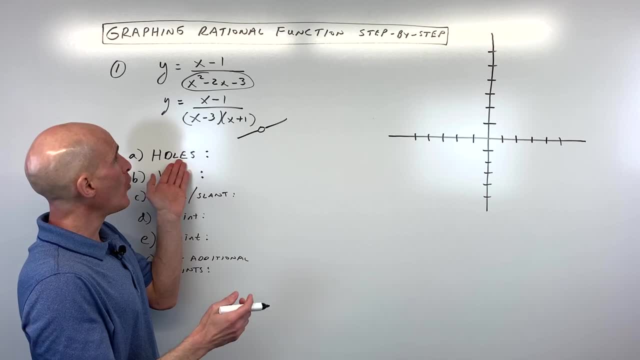 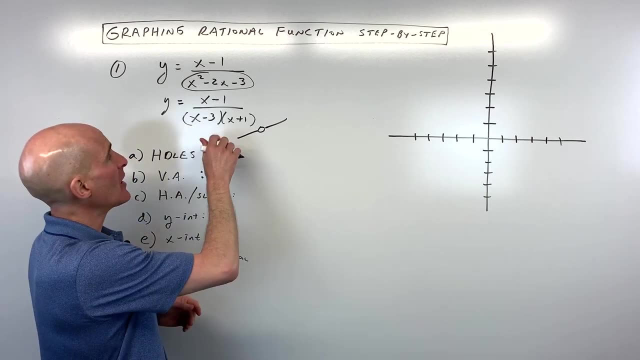 you know, just like a pixel, right? And the way that you know if you have a hole is if there's a factor in the numerator that cancels with a factor in the denominator. We're going to look at an example like that coming up, But in this case you can see there's not a factor in the 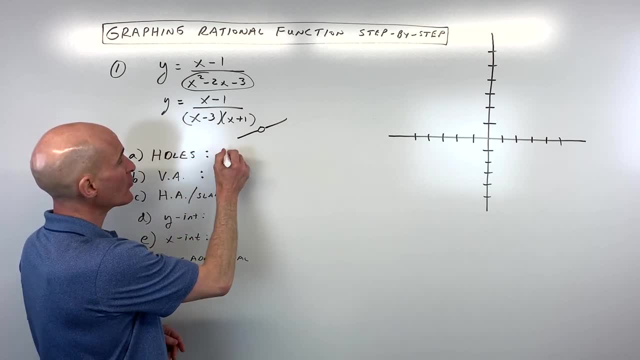 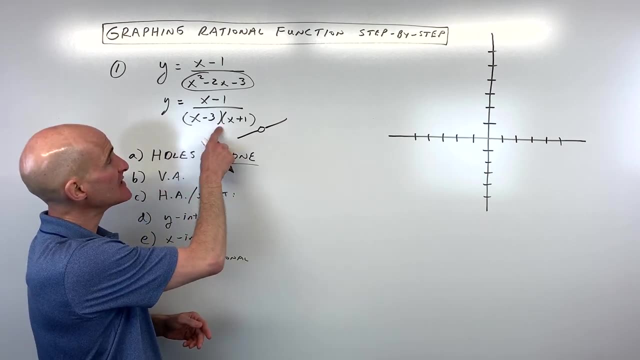 numerator that cancels with a factor in the denominator. So there's no holes, we're just going to write none. Okay, now we're going to go to the vertical asymptotes. Now the vertical asymptotes. you're going to want to look at the denominator And you want to set these. 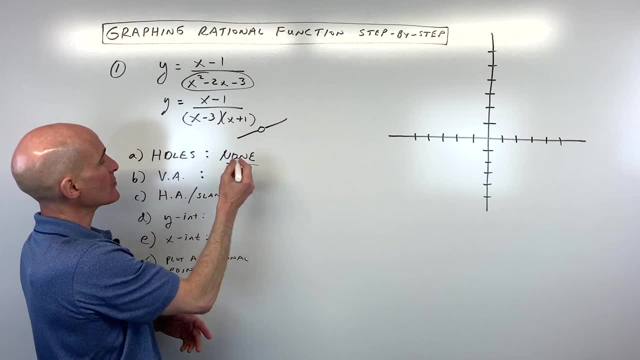 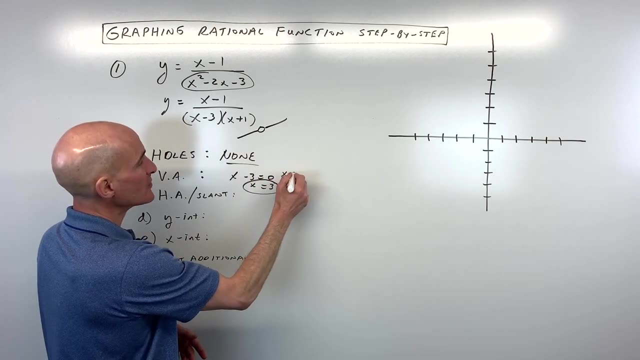 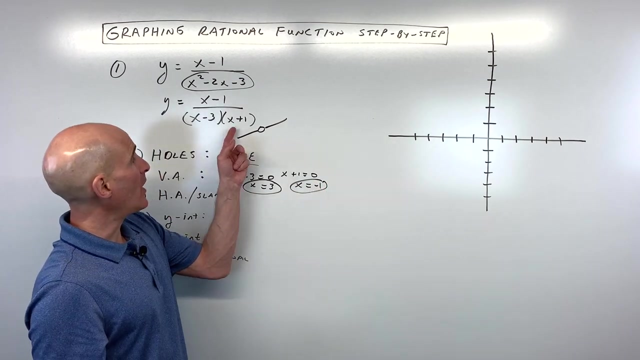 factors equal to zero. So if we say x minus three equals zero and we add three to both sides, you can see x equals three. And if we set x plus one equal to zero, you can see that x equals negative one. Now, really, if you think about it, x cannot be negative one, because negative one plus. 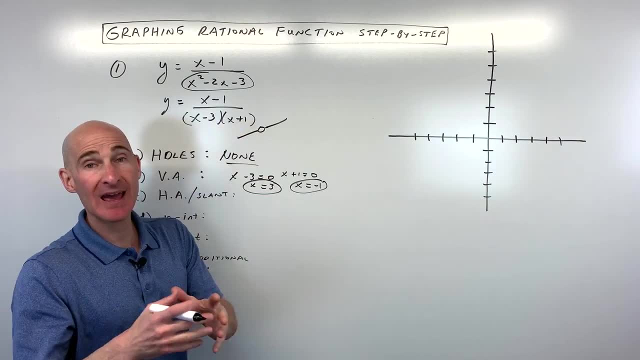 one is zero. zero equals zero. So you're going to want to look at the denominator and you want to see that sometimes this factor will be zero and you can't divide by zero And that's why we get vertical asymptotes by setting these factors in the denominator equal to zero, because we really 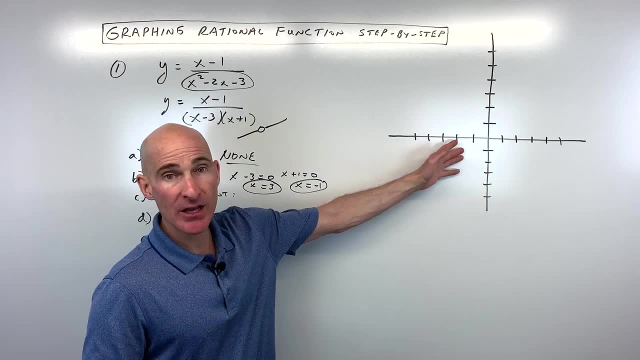 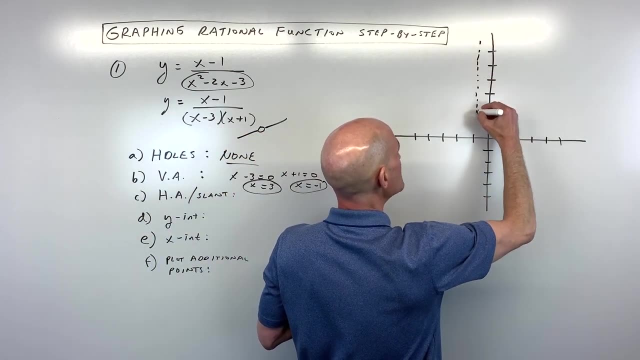 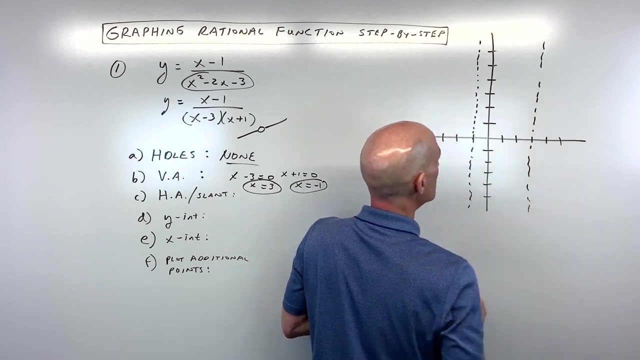 don't want the denominator to be zero. So I like to kind of graph as I go through this, as I go through the different steps. So let's go ahead and graph the vertical asymptote: x equals negative one. Remember x equals lines, are vertical lines, And x equals three, which is right here. Okay. 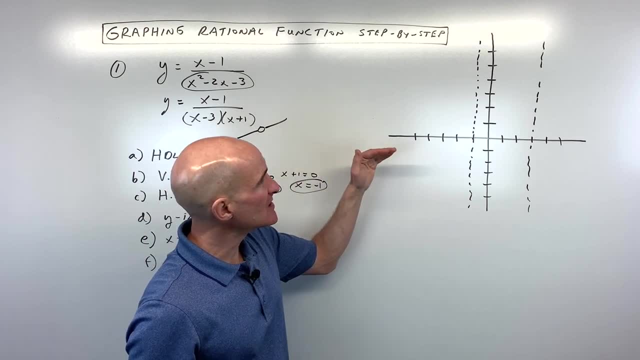 it's a dash or dotted line. you won't actually see the lines on the graph. you're just going to see that the graph is going to get closer and closer. You're going to see that the graph is going to get closer and closer to those lines, but not cross them or touch them. Okay, the next thing is to look. 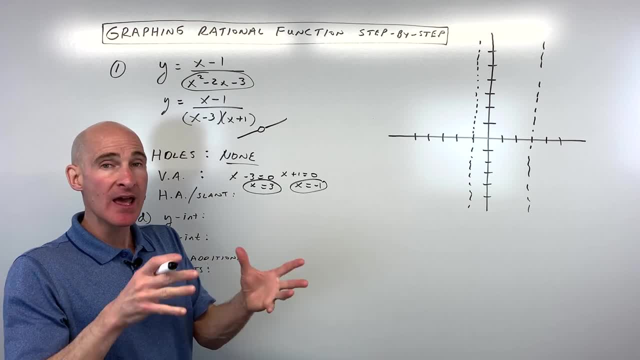 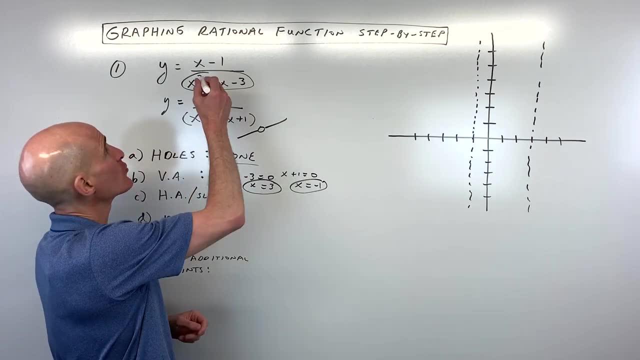 at whether there's a horizontal asymptote or a slant asymptote. It can't be both. it's going to be one or the other. And the way that you analyze the horizontal asymptote is: you want to look at the highest degree term in the numerator and the highest degree term in the denominator. What I 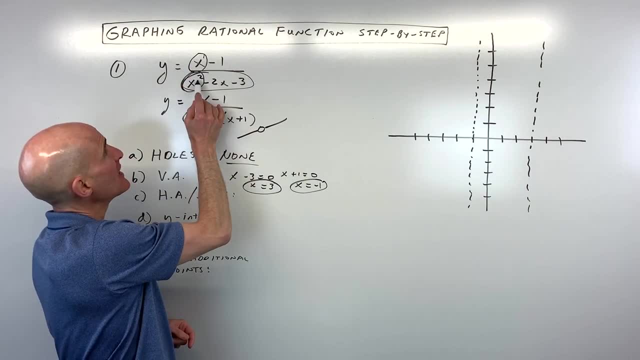 mean by that is, you want to look at these exponents, See how this is like x to the first and this is x to the second power. You want to analyze those highest power terms in the numerator and the denominator. Now, if the denominator is a degree, you want to look at the denominator. 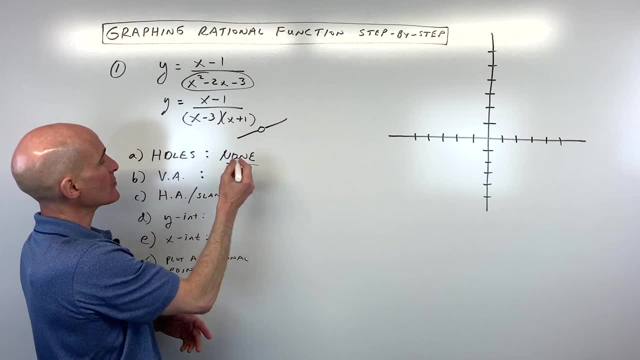 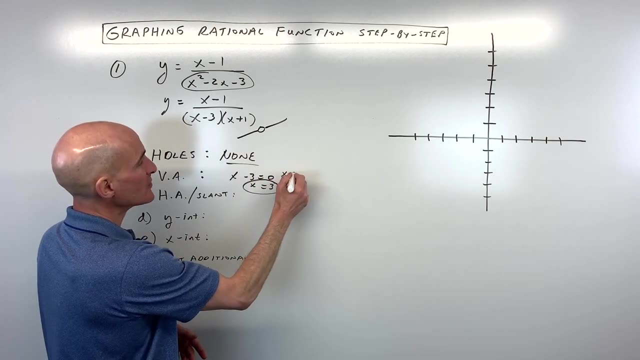 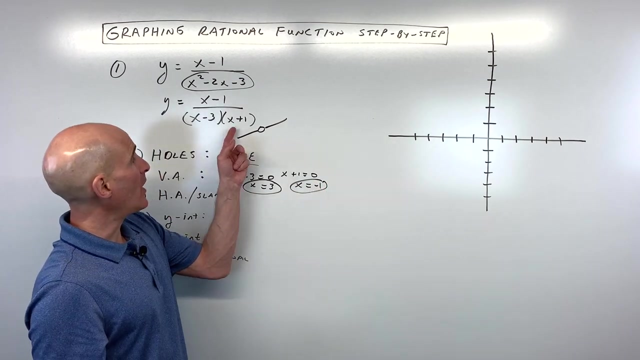 factors equal to zero. So if we say x minus three equals zero and we add three to both sides, you can see x equals three. And if we set x plus one equal to zero, you can see that x equals negative one. Now, really, if you think about it, x cannot be negative one, because negative one plus. 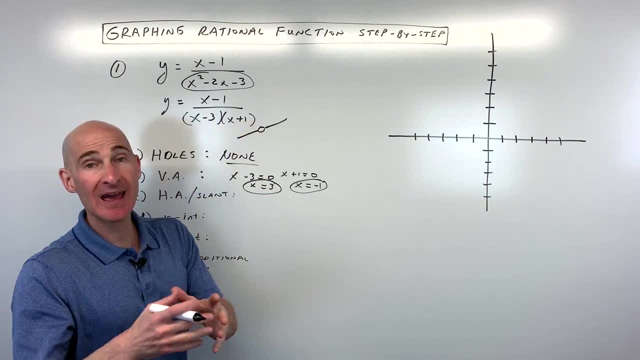 one is zero. zero equals negative one. So, if you think about it, x cannot be negative one because zero times this factor will be zero and you can't divide by zero. And that's why we get vertical asymptotes by setting these factors in the denominator equal to zero, because we really 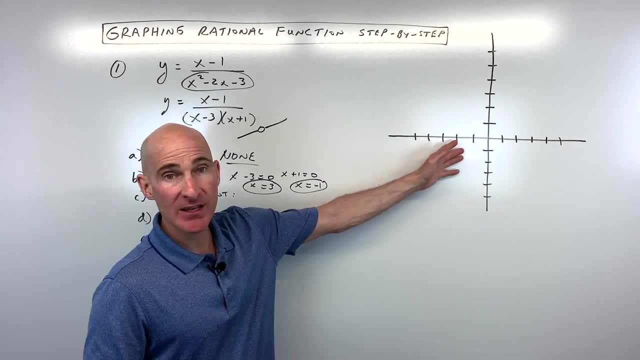 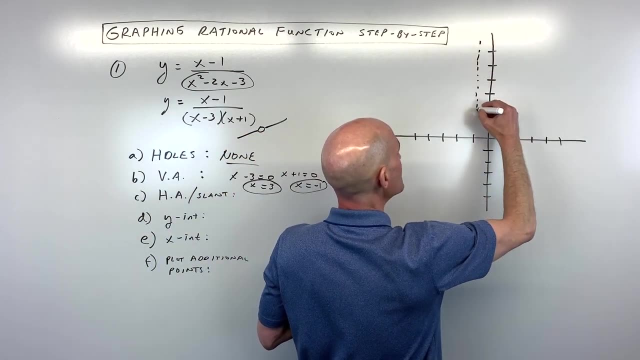 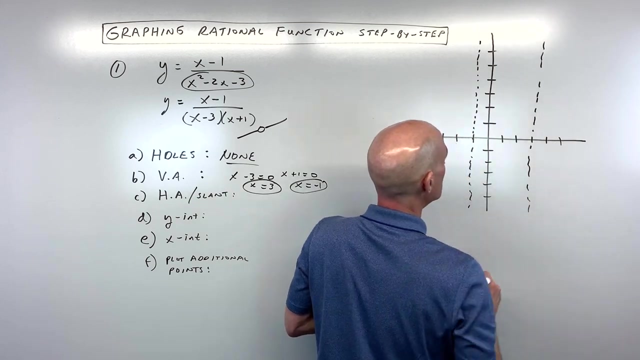 don't want the denominator to be zero. So I like to kind of graph as I go through this, as I go through the different steps. So let's go ahead and graph the vertical asymptote: x equals negative one. Remember, x equals lines, are vertical lines, And x equals three, which is right here. Okay, it's a. 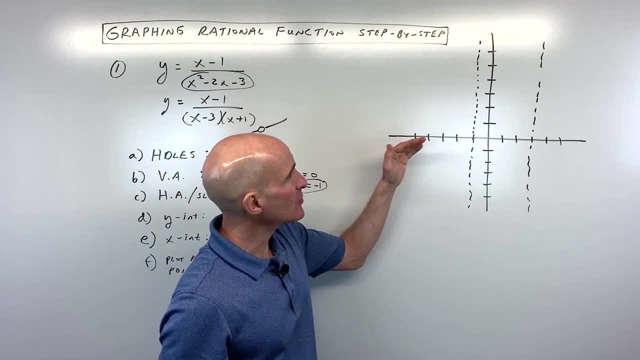 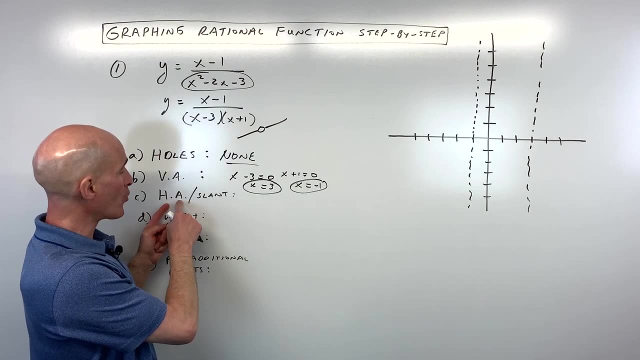 dash or dotted line. you won't actually see the lines on the graph. you're just going to see that the graph is going to get closer and closer to those lines, but not cross them or touch them. Okay, the next thing is to look at whether there's a horizontal asymptote or a slant asymptote. 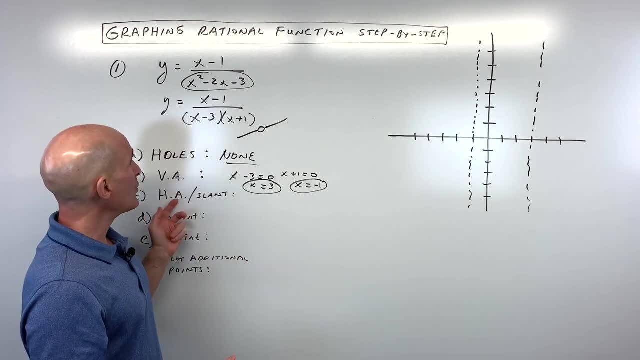 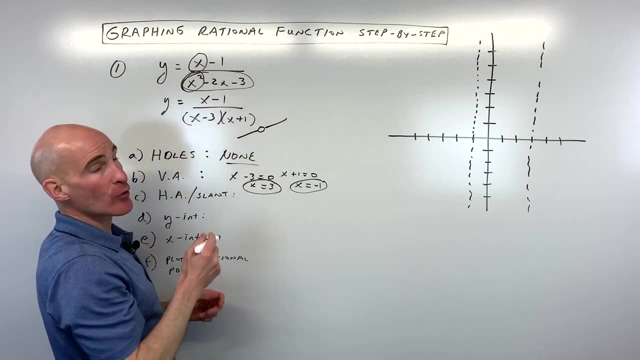 It can't be both. it's going to be one or the other. And the way that you analyze the horizontal asymptote is: you want to look at the highest degree term in the numerator and the highest degree term in the denominator. What I mean by that is: you want to look at these. 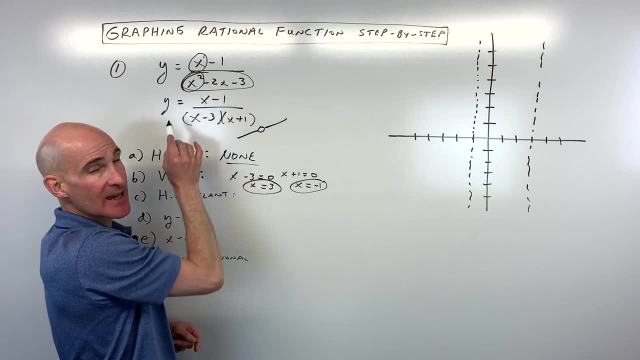 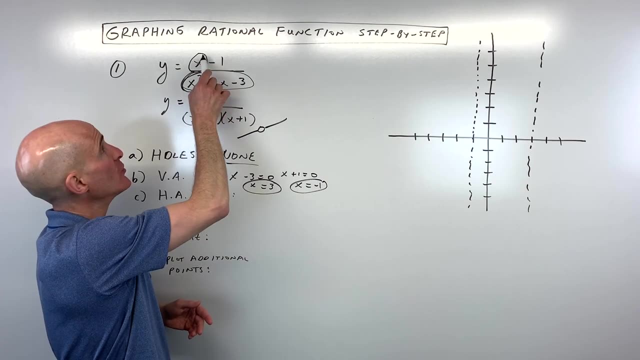 exponents. see how this is like x to the first and this is x to the second power. you want to analyze those highest power terms in the numerator and the denominator. Now, if the denominator's degree is higher than the numerator's highest degree, then the horizontal. 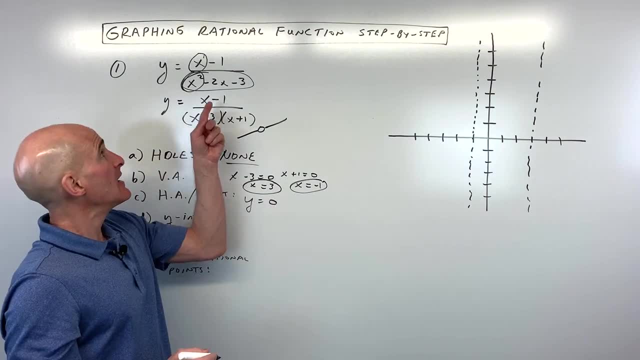 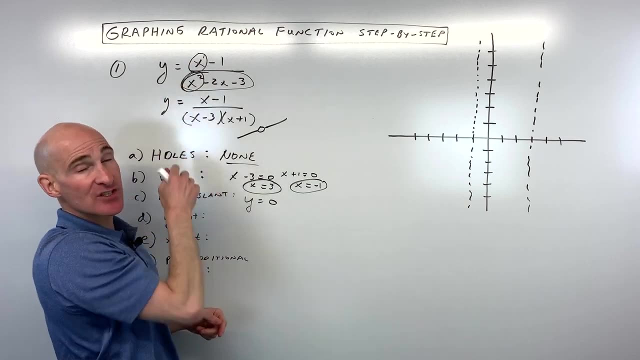 asymptote is going to be: y equals zero. If it's a tie between these two degrees- let's say they were both two or they're both to the third degree- then it's going to be the ratio of the coefficients in front of those variables. And then the third case is if the degree in the 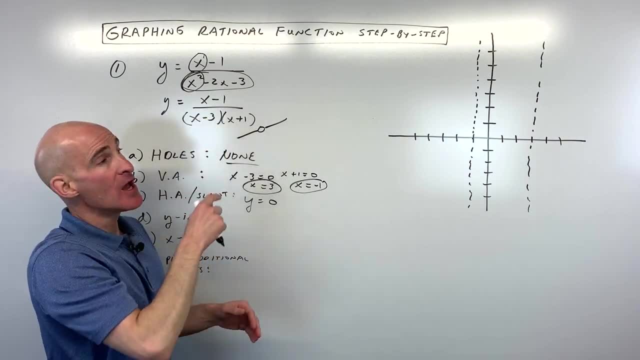 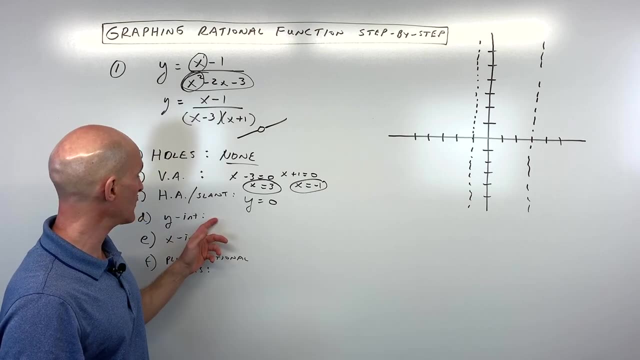 numerator is higher by one than the degree in the denominator, you're going to get a slant asymptote like a diagonal asymptote, And we're going to look at all three of those cases in these example problems. So stay tuned for the next couple examples. But in this case y equals zero. 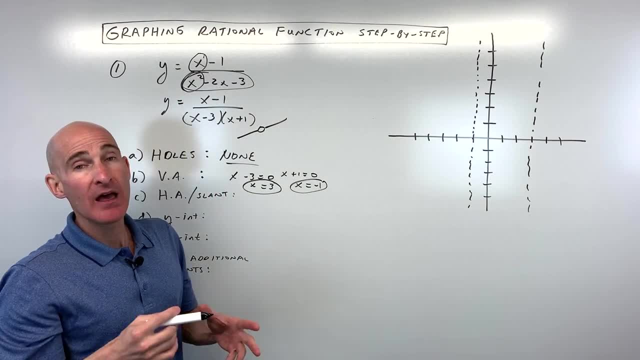 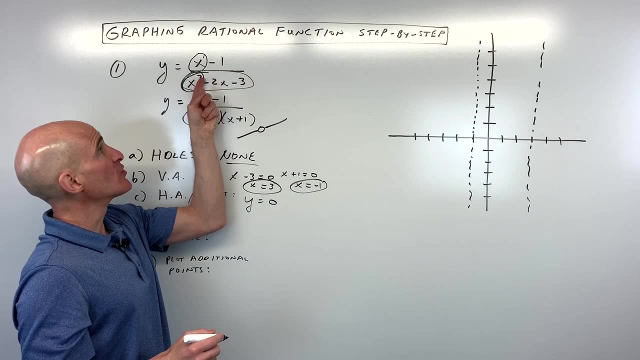 and you want to look at the horizontal asymptote. So if the denominator is higher than the numerator's highest degree, then the horizontal asymptote is going to be y equals zero. If it's a tie between these two degrees- let's say they were both two or they're both to the third degree- then it's going. 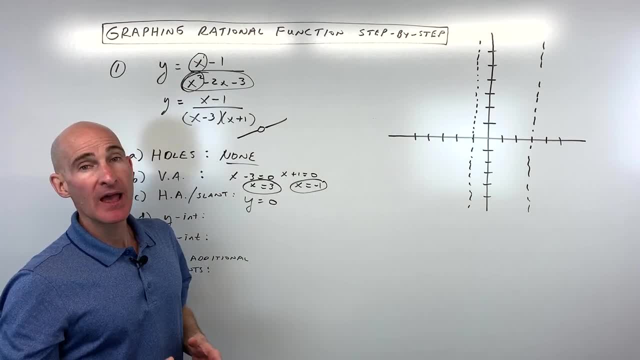 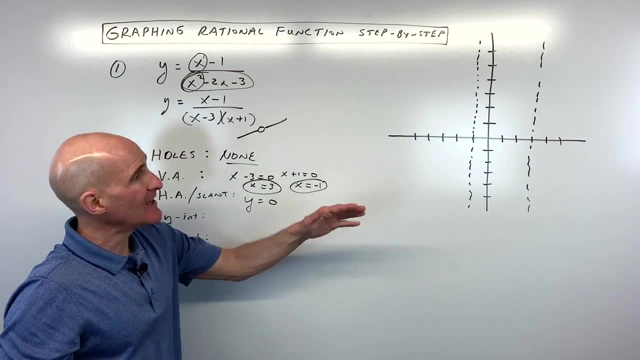 to be the ratio of the coefficients in front of those variables. And then the third case is if the degree in the numerator is higher by one than the degree in the denominator, you're going to get a slant asymptote like a diagonal asymptote, And we're going to look at all three of those cases. in these three example problems. So let's look at the horizontal asymptote and we're going to look at all three of those cases in these three example problems. So let's look at all three of those cases. So let's look at all three of those cases in these three example problems. So stay tuned for the next. 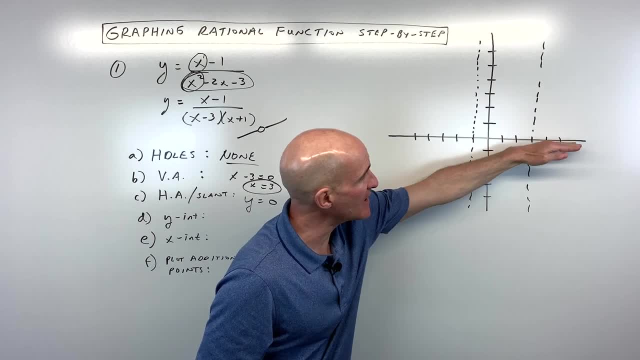 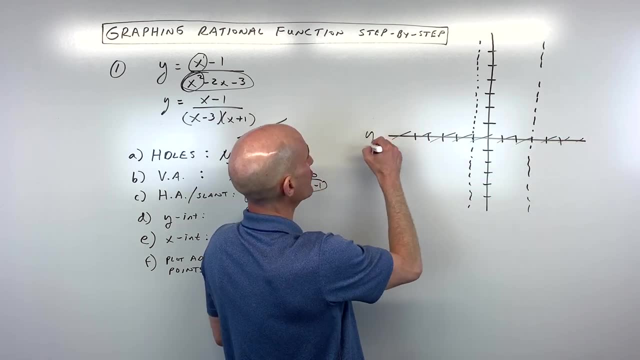 So let's look at all three of those cases in these three example problems. So stay tuned for the next couple examples. But in this case y equals zero. Remember: y equals lines are horizontal lines. y equals zero is actually going to be right on the x-axis, So I'll just write over here: y equals zero. 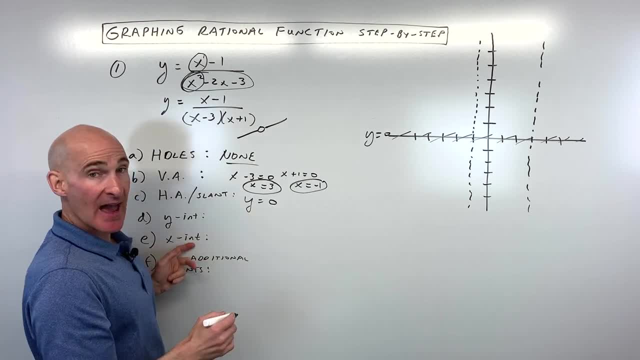 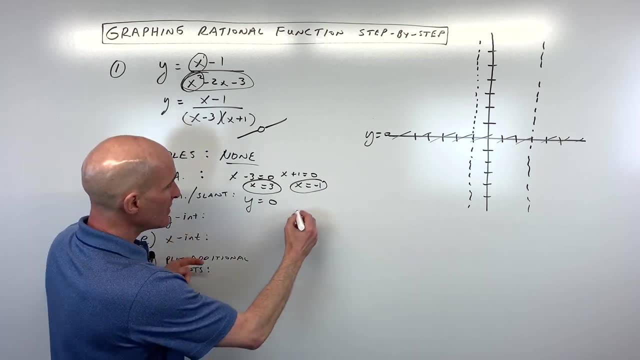 Okay, now we've got the y-intercept and the x-intercept, So these are kind of like some key points that are, you know, easy to find and good to help you get a good graph. So what I like to do with these ones is just think of making like a table like this: If you set x equal to zero, that's. 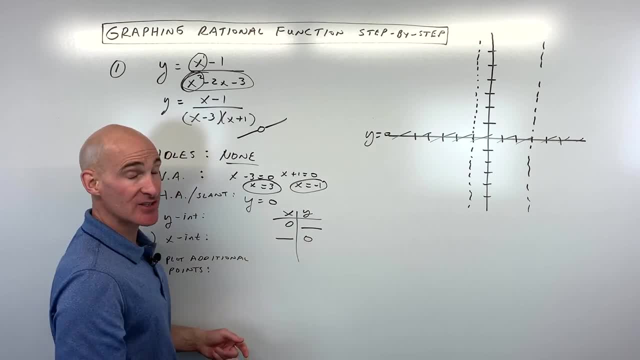 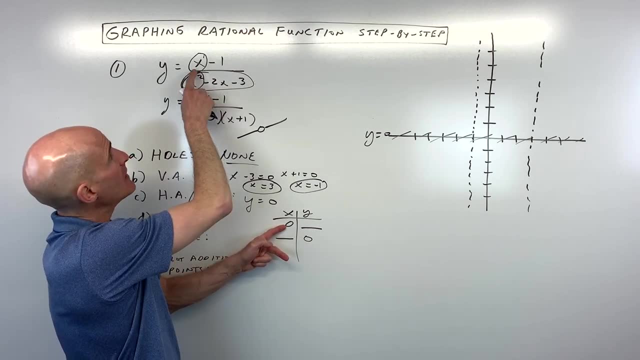 going to give you your y-intercept, And if you set y equal to zero, that's going to give you your x-intercept. So let's go ahead and put zero in for x. Sometimes I like to go back to the original problem before we factored it. If you put zero in for x, that's going to cancel out this term. 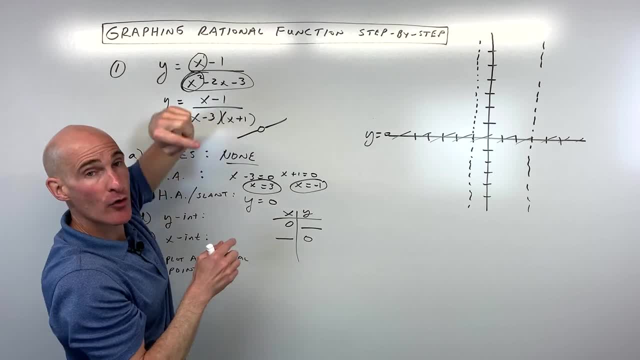 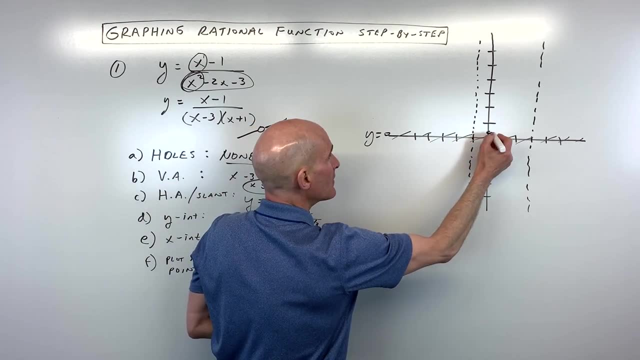 this term and this term. So you're really going to be just left with negative one over negative three, which those two negatives cancel, and that gives you one-third. So zero comma. one-third is going to be right here on the y-axis, Now the x-intercept. we have to set the y. 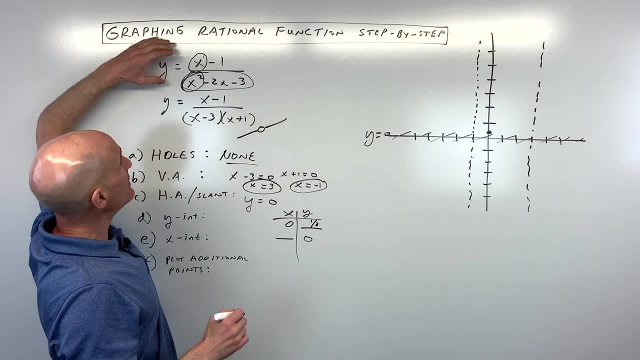 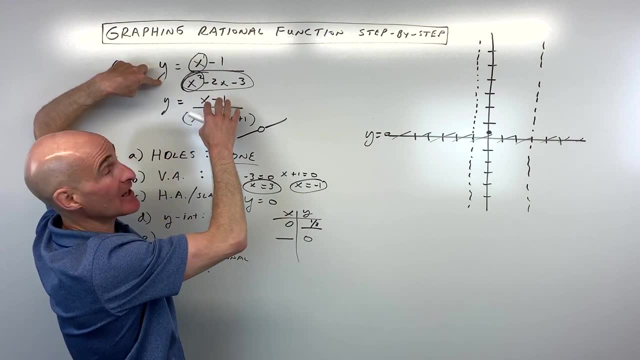 variable equal to zero. That's over here. But one thing to kind of notice is that the only way that y would be equal to zero is if the numerator is equal to zero and the denominator is not equal to zero. But basically just set the numerator to zero, because if you have like zero over something, 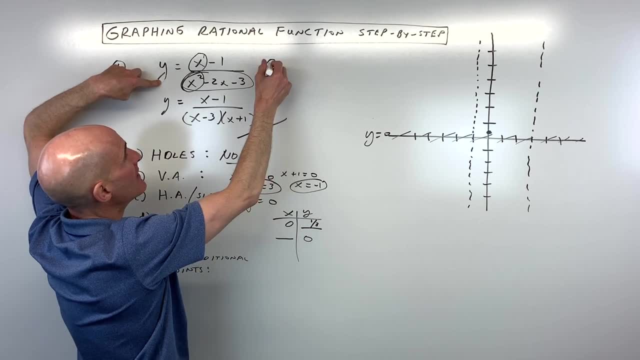 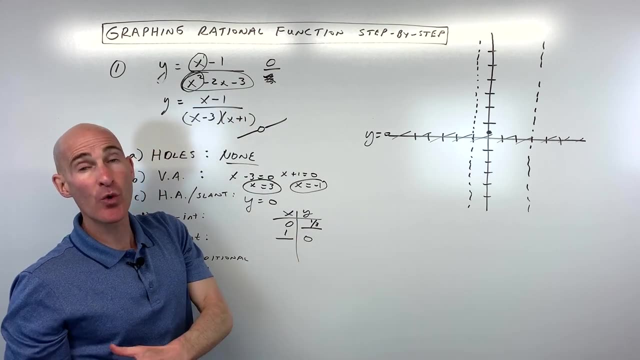 that's not zero. right like that, that fraction is going to be equal to zero. That means y equals zero. So we're just going to set the numerator to zero. x minus one equals zero. That's going to be x equals one when you add one to both sides. So that means this is going to cross right here. 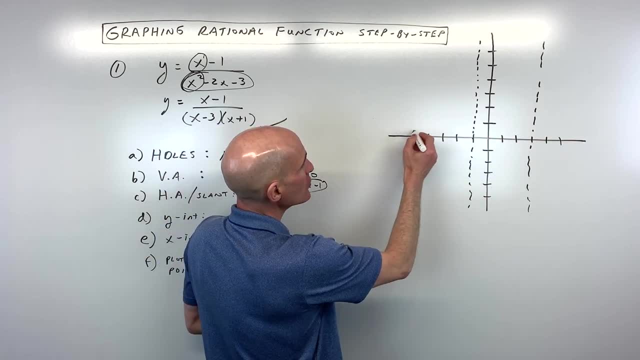 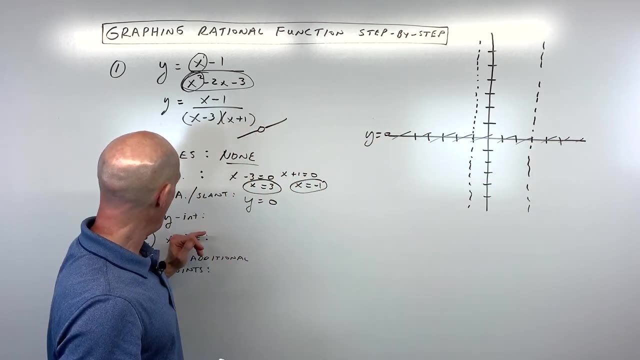 remember, y equals lines are horizontal lines. y equals zero is actually going to be right on the x-axis. I'll just write over here: y equals zero. Okay, now we've got the y-intercept and the x-intercept, So these are kind of like some key points that are, you know, easy to find. 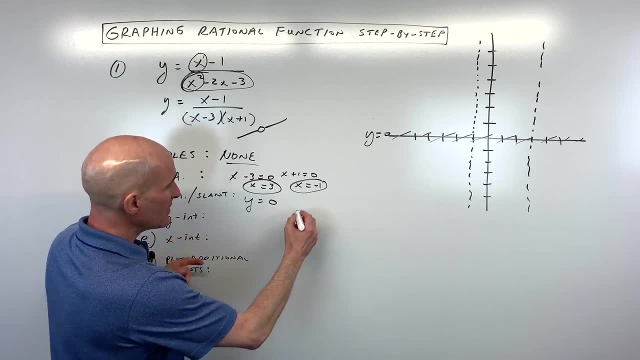 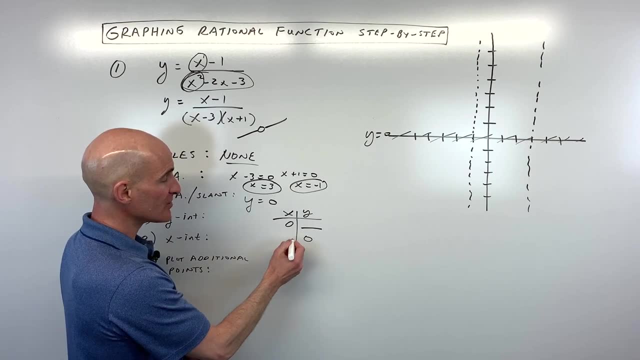 and good to help you get a good graph. So what I like to do with these ones is just think of making like a table like this: If you set x equal to zero, that's going to give you your y-intercept, And if you set y equal to zero, that's going to give you your x-intercept. 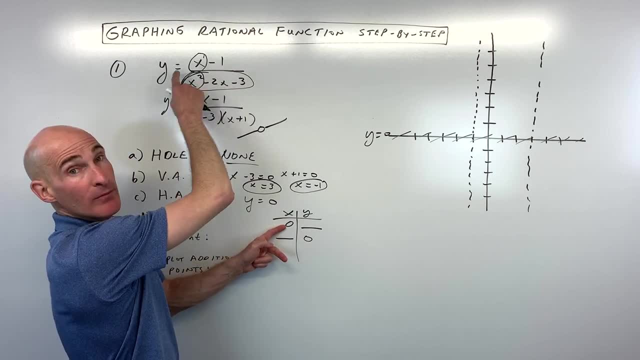 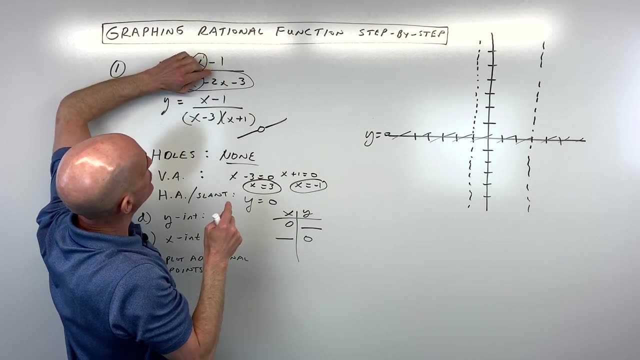 So let's go ahead and put zero in for x. Sometimes I like to go back to the original problem before we factored it. If you put zero in for x, that's going to cancel out this term, this term and this term, So you're really going to be just left with negative one over negative. 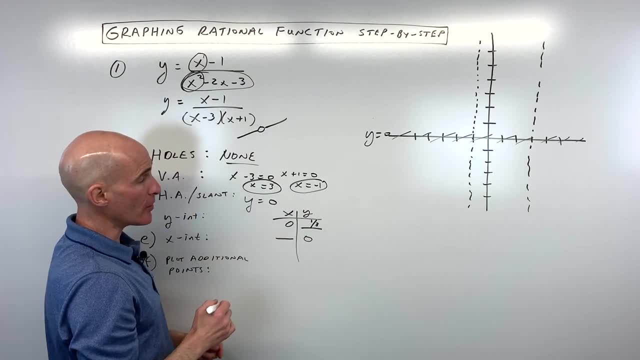 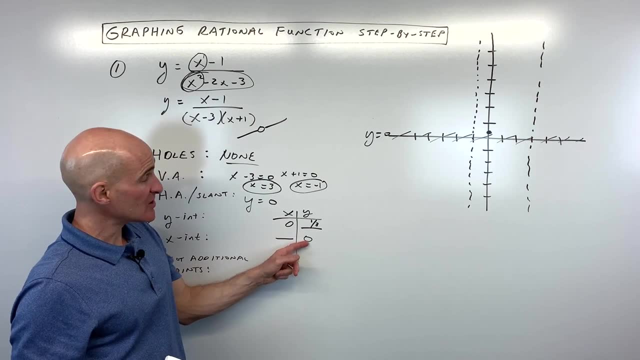 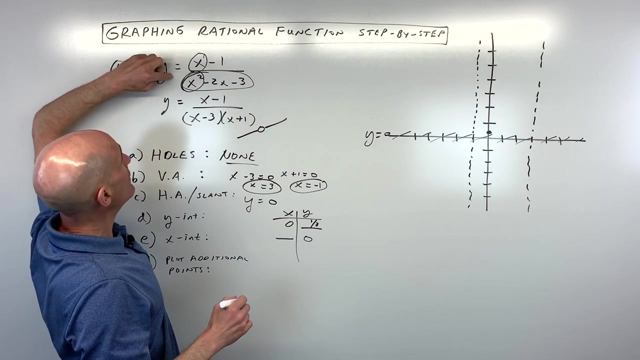 three, which those two negatives cancel, and that gives you one third. So zero comma one third is going to be right here. on the y-axis, Now the x-intercept, we have to set the y variable equal to zero. That's over here. But one thing to kind of notice is that the only way that 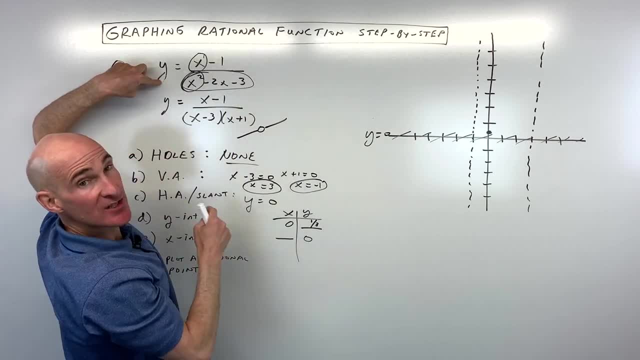 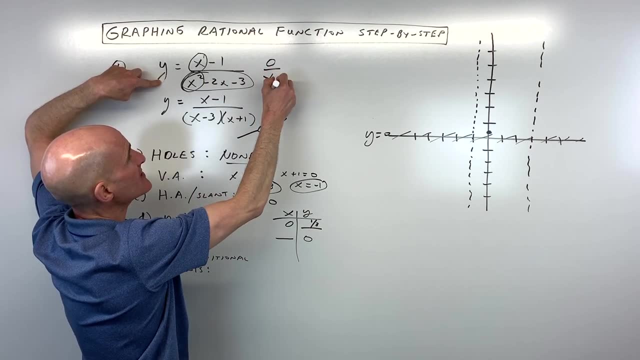 y would be equal to zero is if the numerator is equal to zero and the denominator is not equal to zero. But basically just set the numerator to zero, because if you have like zero over something that's not zero, right like that, that fraction is going to be equal to zero. That means y equals. 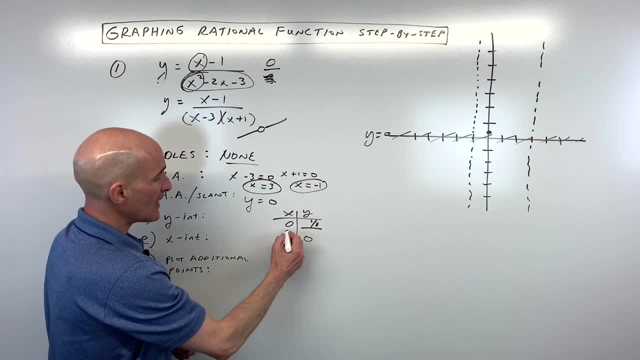 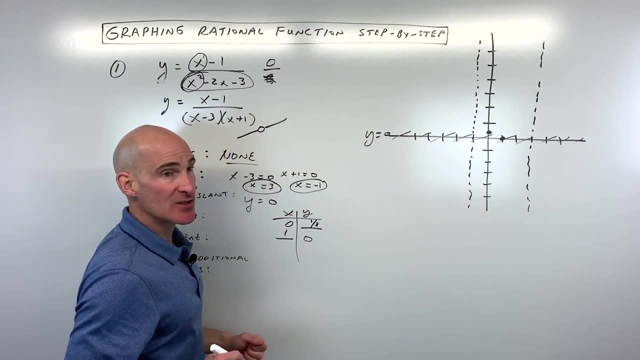 zero. So we're just going to set the numerator to zero. x minus one equals zero. That's going to be x equals one when you add one to both sides. So that means this is going to cross right here at one comma zero. So basically you're setting the opposite variable equal to zero. What some 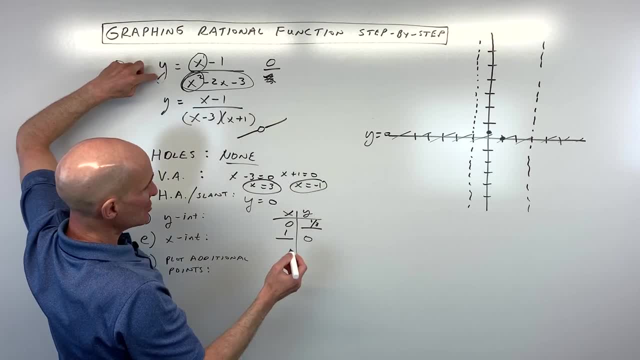 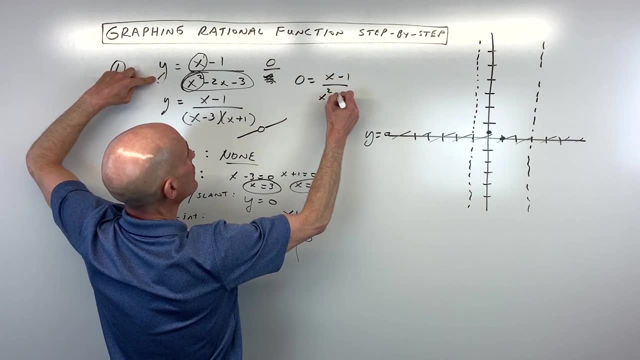 students like to do- like that part was a little confusing to you- is again: just put zero in for y, So this would be like: zero equals x minus one over x. squared minus two, x minus three. Zero is like zero over one, And what you can do is you can cross multiply if you know the. 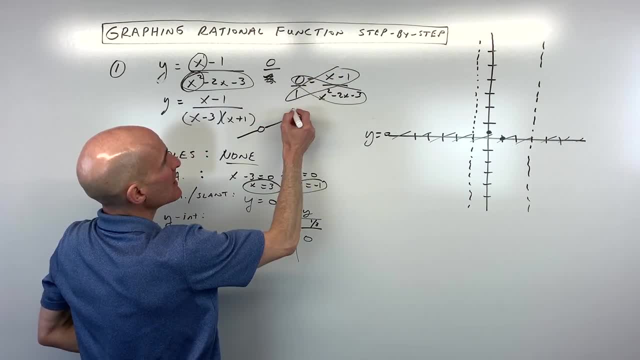 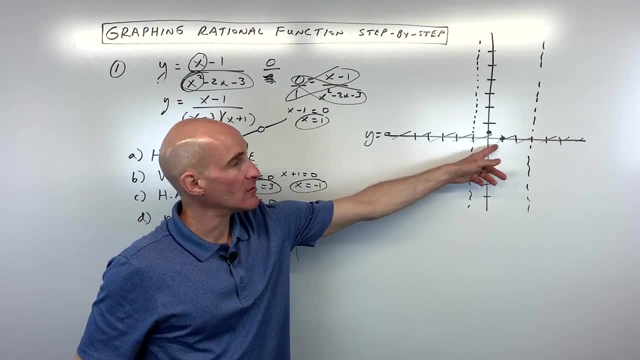 cross product property. x minus one times one is itself, and this times zero is just zero. So then, if you do that, you're going to get x minus one over x squared minus two, x minus three, So you're adding one to both sides. x equals one, So that's your x intercept. So just two different ways to 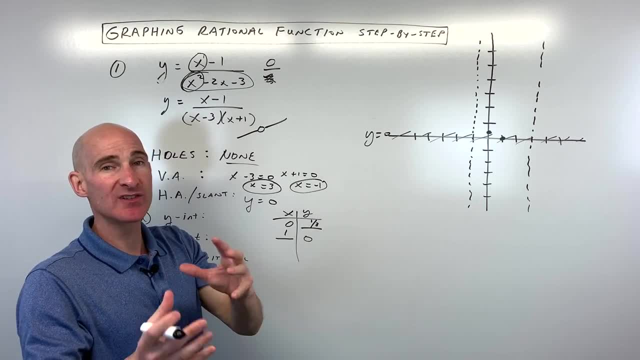 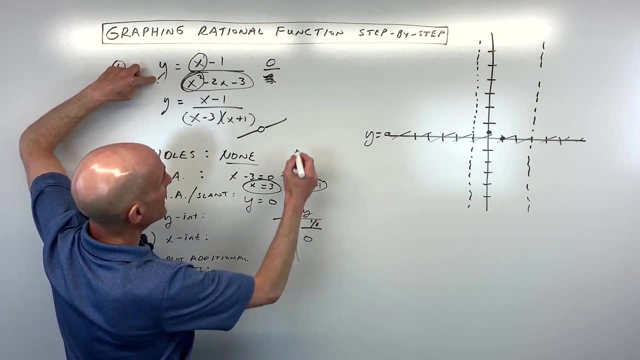 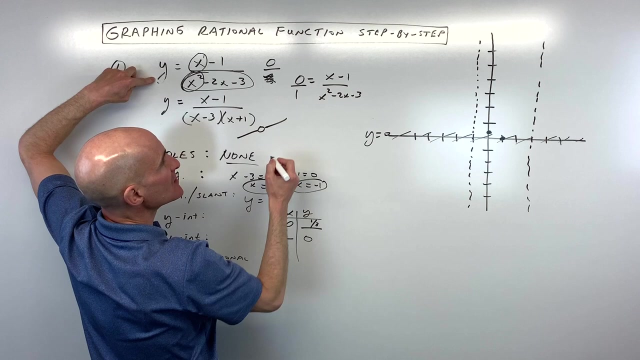 at one comma zero. So basically you're setting the opposite variable equal to zero. What some students like to do- like that part was a little confusing to you- is again just put zero in for y. So this would be like: zero equals x minus one over x squared minus two, x minus three. Zero is like: 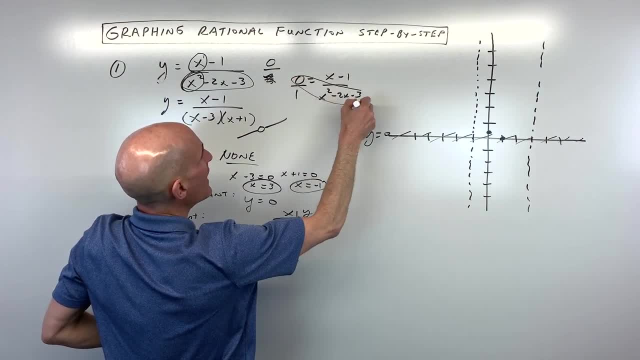 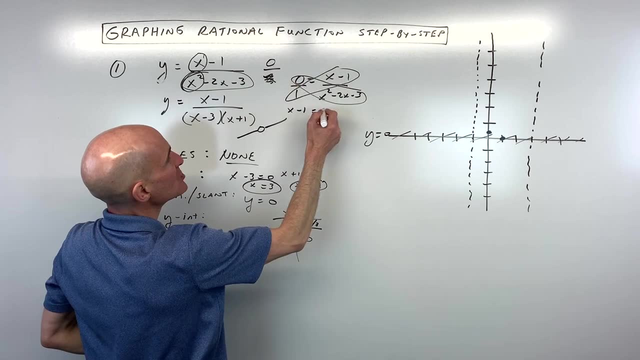 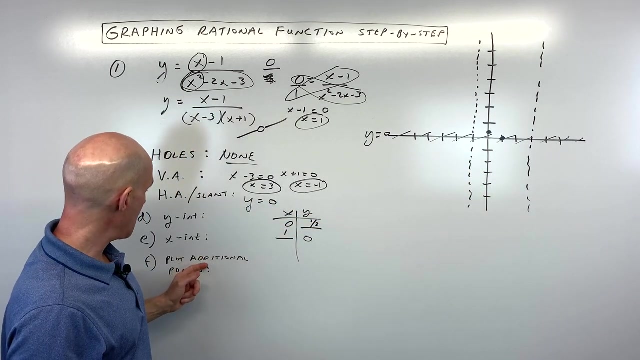 zero over one, And what you can do is you can cross, multiply. if you know the cross product, a property, x minus one times one is itself, And this times zero is just zero. So then if you add two times zero you get zero. So that's x minus one times one. So that's your x-intercept. So 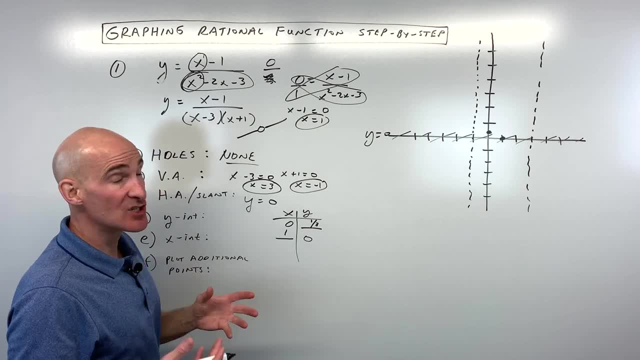 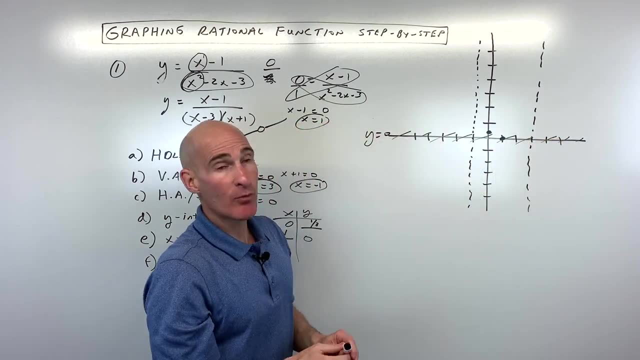 just two different ways to look at it. And then the last part is to plot additional points to get a good graph. Now what I like to do here is see: you can cross a horizontal asymptote, That's no problem, You can cross it. A vertical asymptote, you cannot cross or touch because you would be. 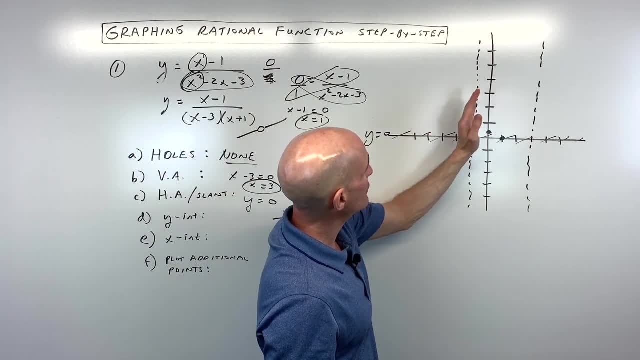 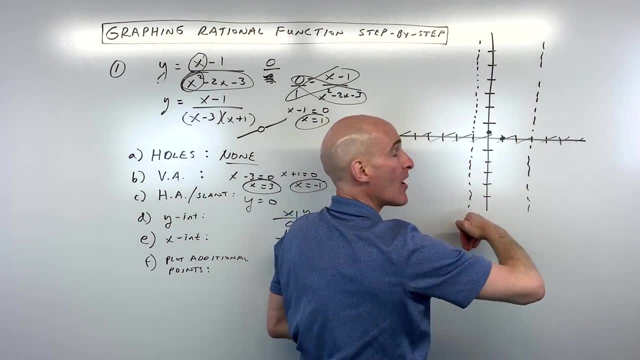 dividing by zero, and that's undefined. But what happens is because you can't cross these vertical asymptotes. you can't cross these vertical asymptotes. you can't cross these vertical asymptotes. So what you can do is you can either go from the left side or from the right side. It's either. 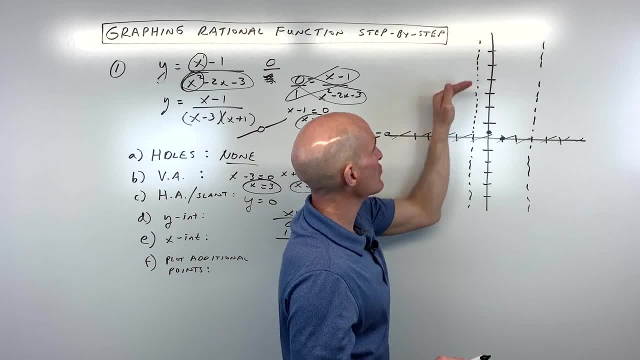 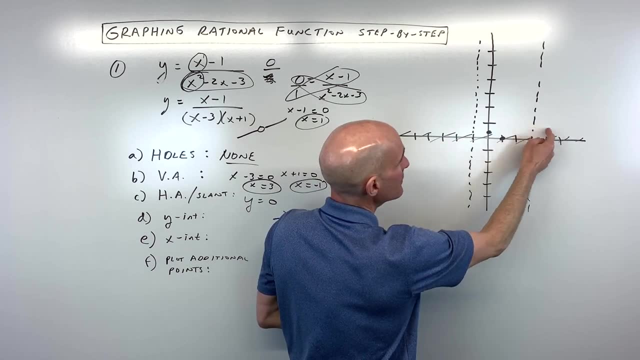 going to go up like this or it's going to go down like that. So either up towards positive infinity, down towards negative infinity. It's basically like a brick wall: You can't go through it. You're either going to have to turn like that or turn like that. So what I recommend doing is: 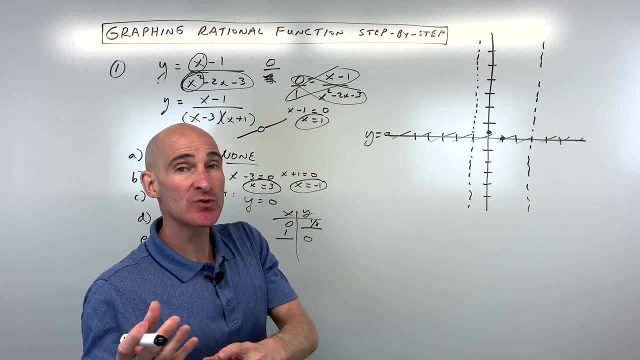 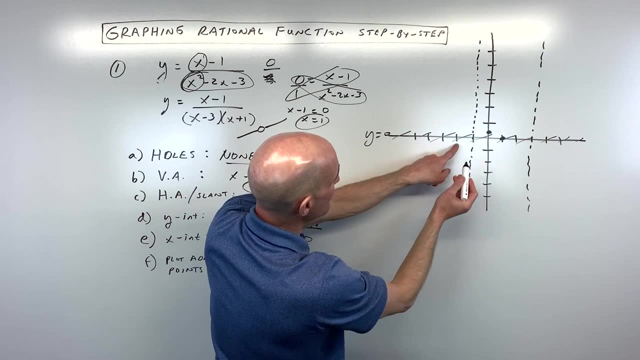 picking some points on either side of the vertical asymptotes, And you can do this one of two ways. You can do what they call sign analysis, which I'm going to show you in this video, Or you can just take negative two. So negative two. I'm going to put it into this factored form right here. 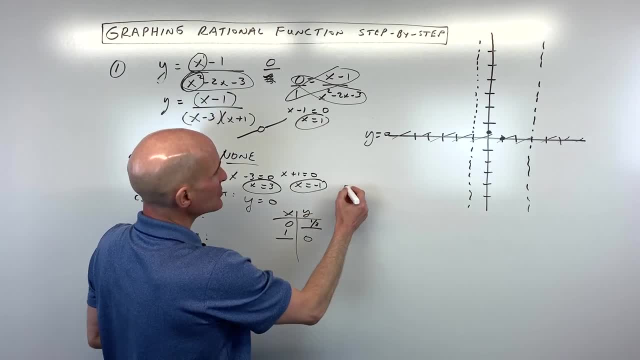 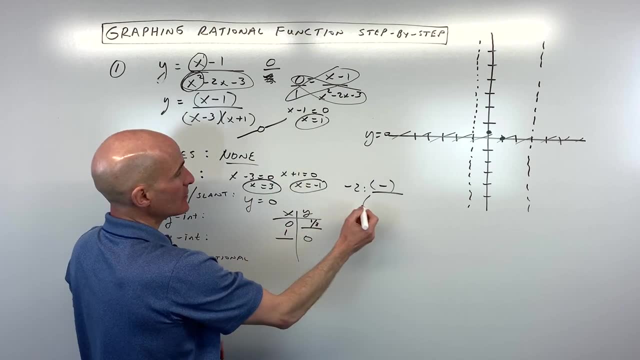 Negative. two minus one is negative three, Which I'm just going to write this as a negative because it came out to negative three. And then over here, negative two minus three is negative five. So I'm going to write negative And negative. two plus one is negative one. I'm 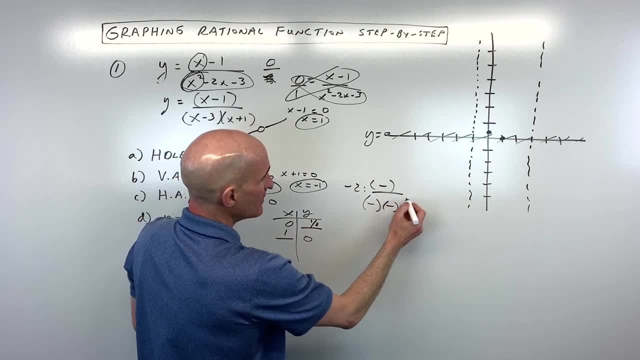 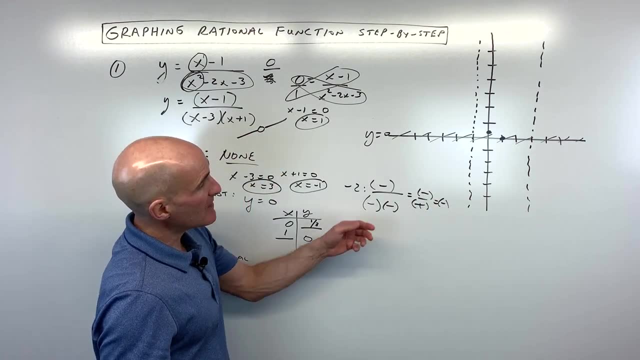 just going to write negative A negative times. a negative is a positive And a negative divided by a positive is a negative, right? So what that means is that when you divide by a positive, when you're approaching from this side, okay, over here. at negative two, it's going to be negative. 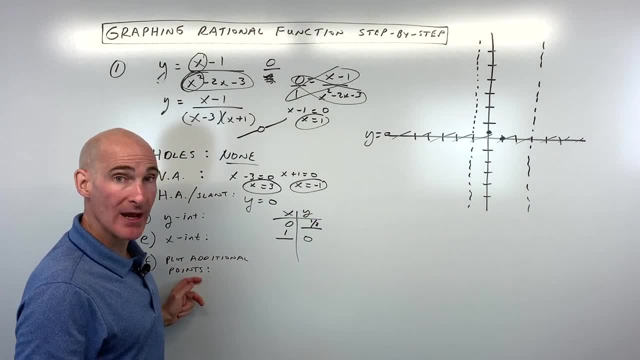 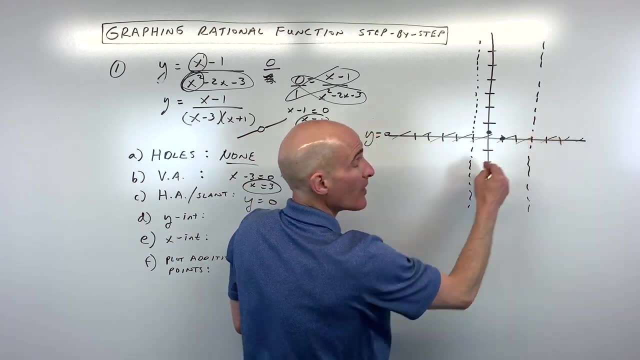 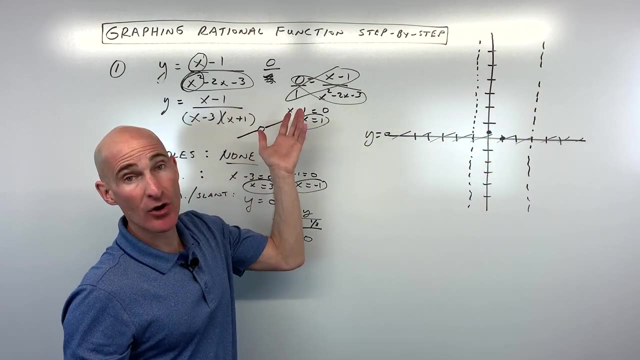 look at it And then the last part is to plot additional points to get a good graph. Now what I like to do here is see: you can cross a horizontal asymptote, That's no problem, You can cross it. A vertical asymptote, you cannot cross or touch because you would be dividing by zero. 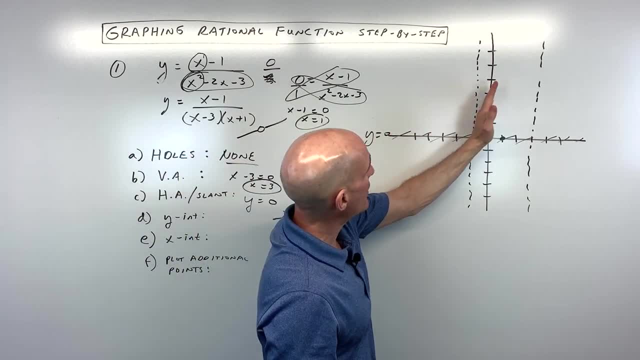 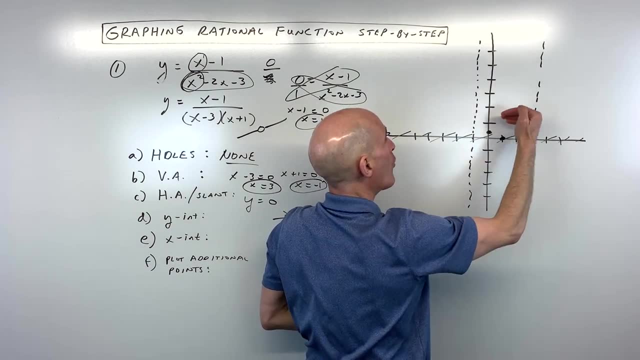 and that's undefined. But what happens is because you can't cross these vertical asymptotes when you approach it from the left side or from the right side, it's either going to go up like this or it's going to go down like that. 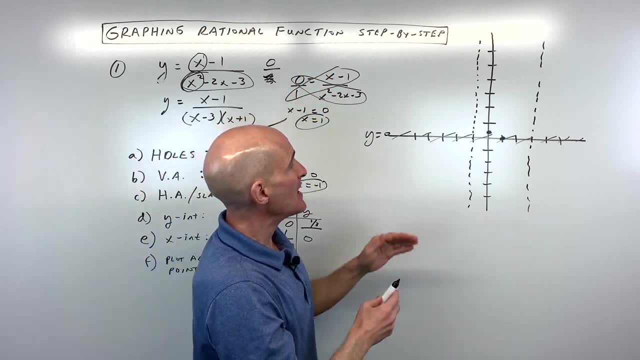 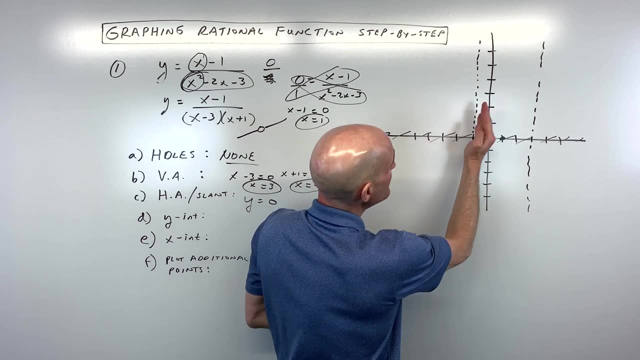 So either up towards positive infinity, down towards negative infinity. It's basically like a brick wall: You can't go through it. You're either going to have to turn like that or turn like that. So what I recommend doing is picking some points on either side of the vertical. 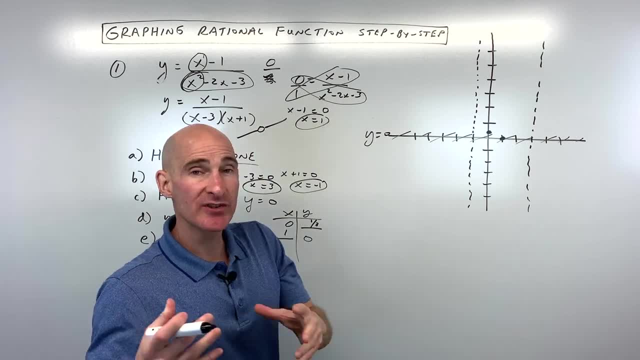 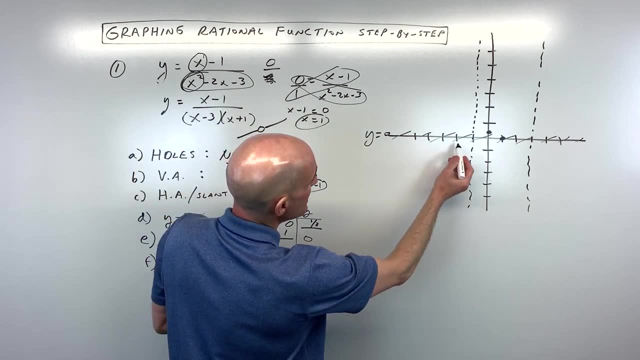 asymptotes. And you can do this one of two ways. You can do what they call sine analysis, which I'm going to show you in this video, or you can just go ahead and just plot some points, But let me show you. So let's say, for example, if we were to do this: 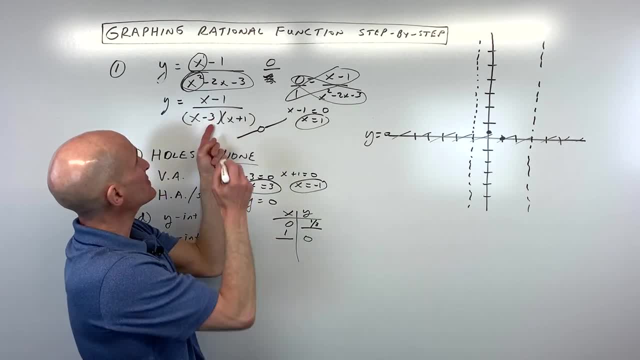 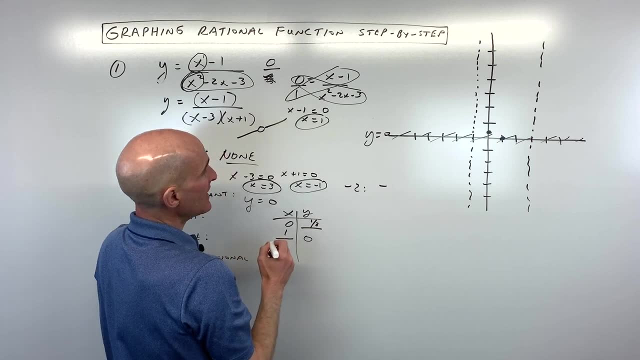 we were to take negative 2.. So negative 2, I'm going to put it into this factored form right here: Negative 2 minus 1 is negative 3, which I'm just going to write this as a negative because it. 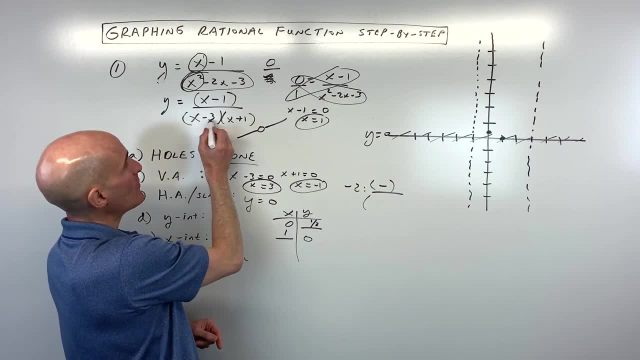 came out to negative 3.. And then, over here, negative 2 minus 3 is negative 5.. So I'm going to write negative And negative. 2 plus 1 is negative 1.. I'm just going to write negative. 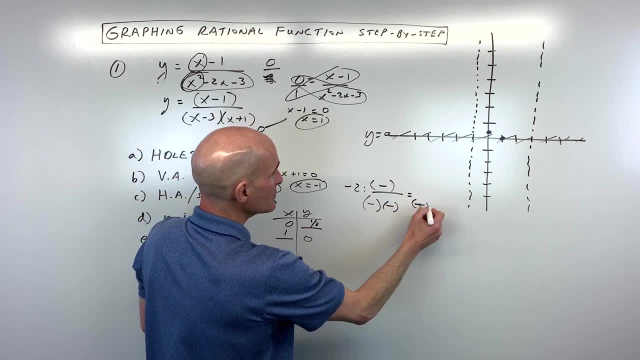 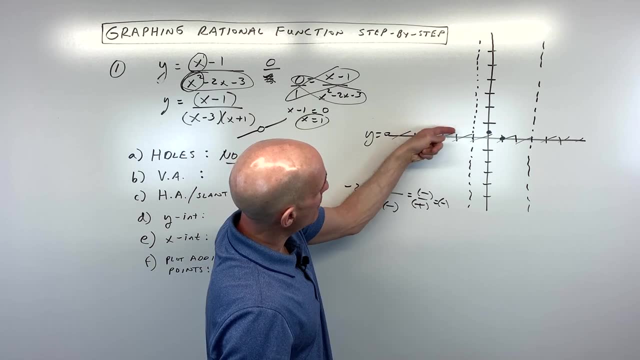 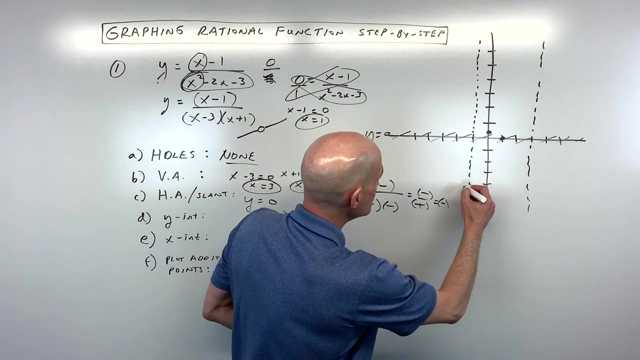 A negative times, a negative is a positive And a negative divided by a positive is a negative. When you're approaching from this side over here at negative 2, it's going to be negative, meaning it's going to go down towards a negative infinity. So I'm just going to draw an arrow like: 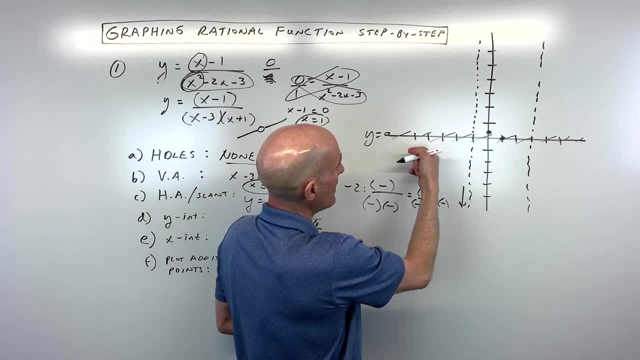 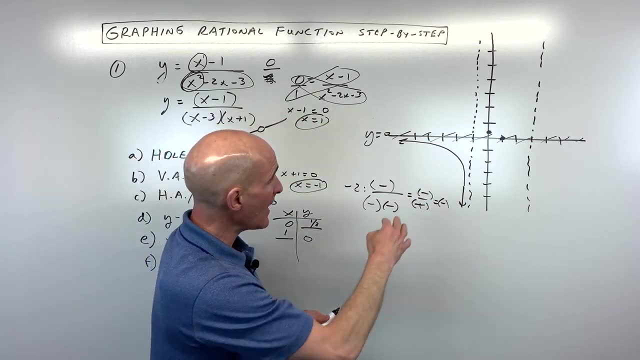 that And I can tell that this graph is going to approach this horizontal asymptote- see on the x-axis like that. So that gives us a pretty good idea what the graph looks like. Again, you can plot additional points, But our main concern is whether it's going down as it approaches. 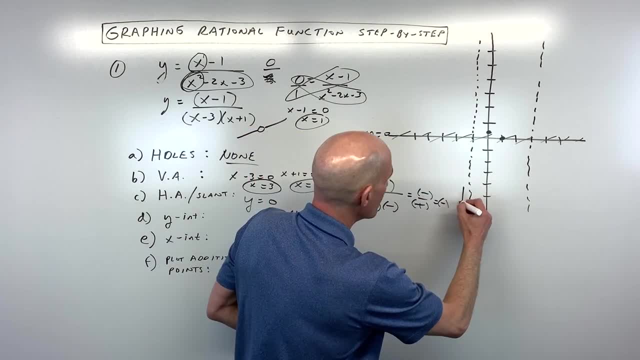 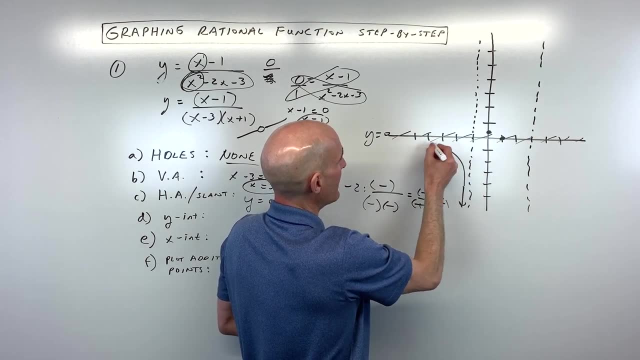 Meaning it's going to go down towards a negative infinity. So I'm just going to draw an arrow like that And I can tell that this graph is going to approach this horizontal asymptote. see on the x-axis like that. So that gives us a pretty good idea what the graph looks like. Again, you can 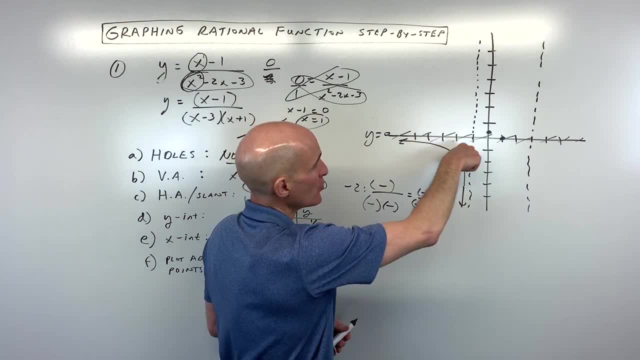 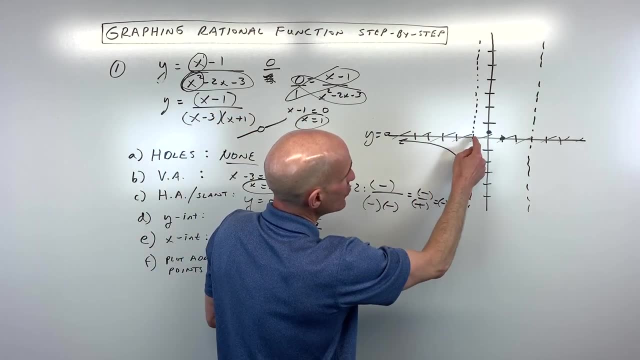 plot additional points, But our main concern is whether it's going down as it approaches this vertical asymptote or whether it's going up towards positive infinity. Okay, now let's pick a point on vertical asymptote. I'm going to pick like negative 0.9.. So I'll just write that down. 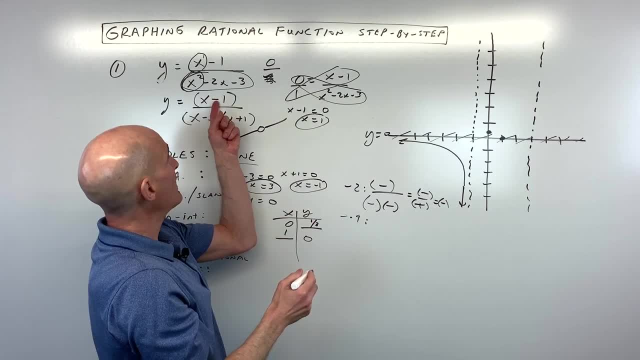 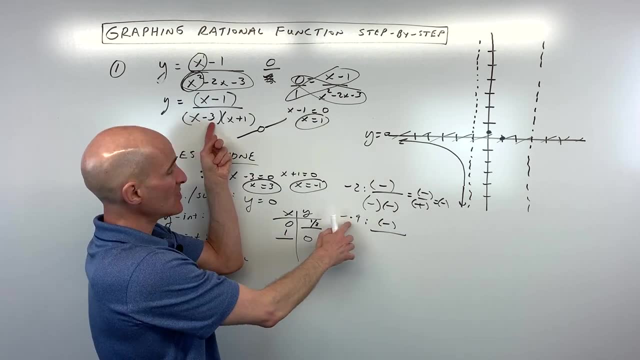 Negative 0.9.. So if we put negative 0.9 in the numerator, that's going to be negative 1.9, which is just negative. Negative 0.9 minus 3 is negative 3.9.. That's negative And negative 0.9. 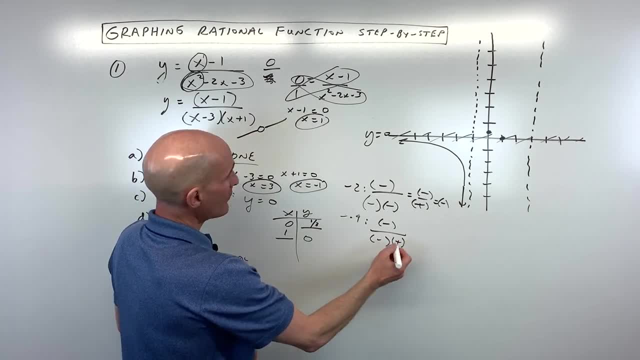 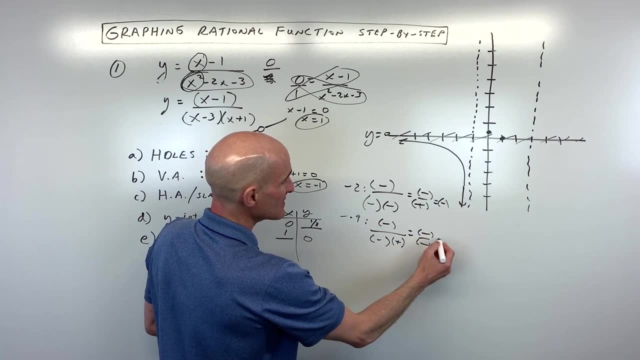 plus 1 is positive 0.1, right, So that comes out to a negative And a negative times. a positive is a negative And a negative divided by a negative is a positive. That tells us that we're over here at negative 0.9.. This is going up towards positive infinity. You can. 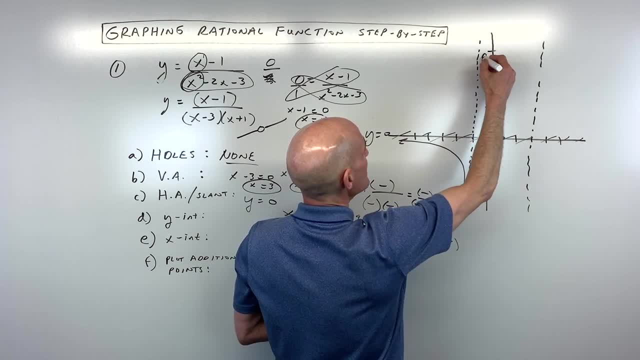 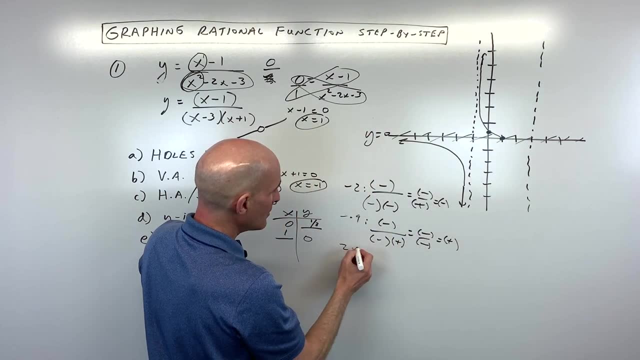 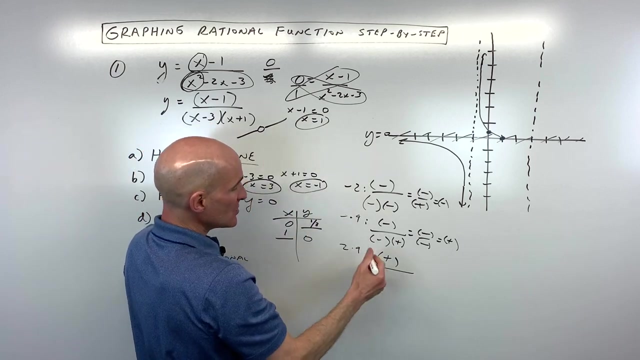 probably tell that, because you see these points going like this. It's going to go like this, right? Okay, now let's pick some points on either side of this vertical asymptote, Maybe like 2.9 now. So if I put 2.9 in here, 2.9 minus 1 is going to give us a positive value. 2.9 minus 3 is going 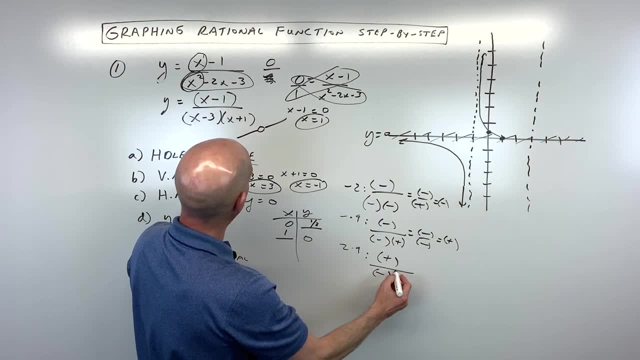 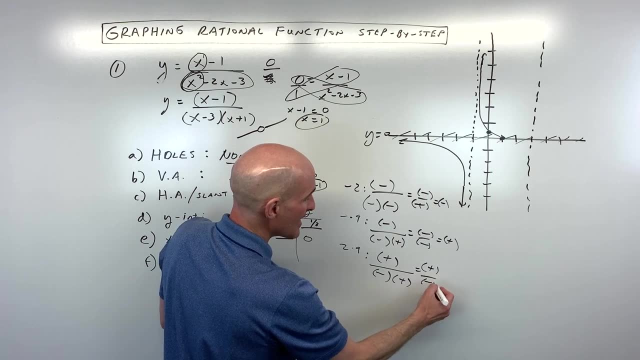 to give us a negative value, And 2.9 plus 1 is going to give us a positive value. So here we get a positive A negative times. a positive is a negative, But a positive divided by a negative is a negative, which means this is going down towards negative infinity, But we probably already. 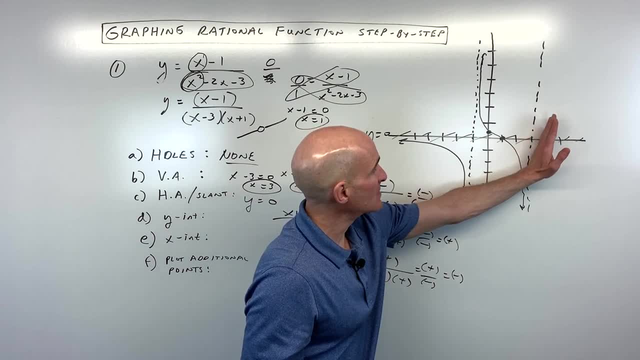 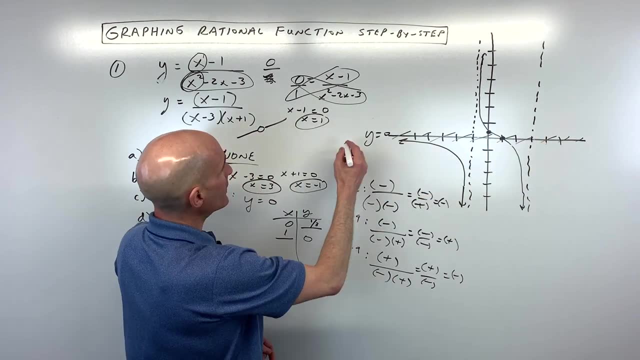 knew that just based on these couple of points here. The last one is to pick over here, just to the right of this vertical asymptote, maybe here at 3.1. Or we could even just do 4.. So if we put 4 in, let's see that's 4 minus 1, which is 3.. That's positive, And 4 minus 3 is 1. That's. 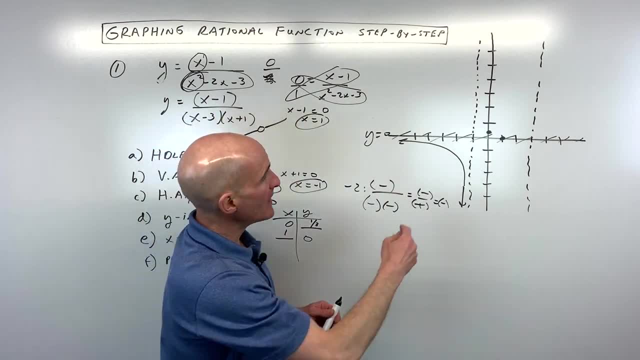 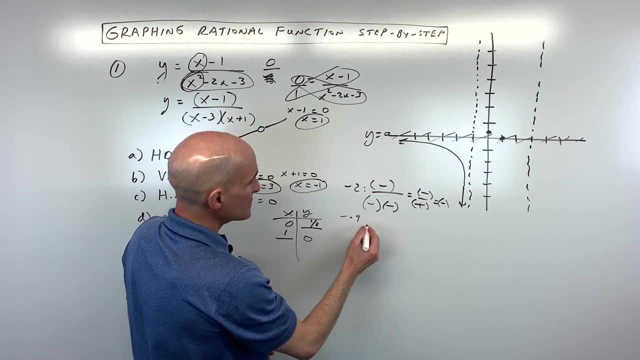 this vertical asymptote or whether it's going up towards positive infinity. Now let's pick a point. vertical asymptote I'm going to pick like negative 0.9.. So I'll just write that down: negative 0.9.. So if we put negative 0.9 in the numerator, that's going to be negative 1.9,. 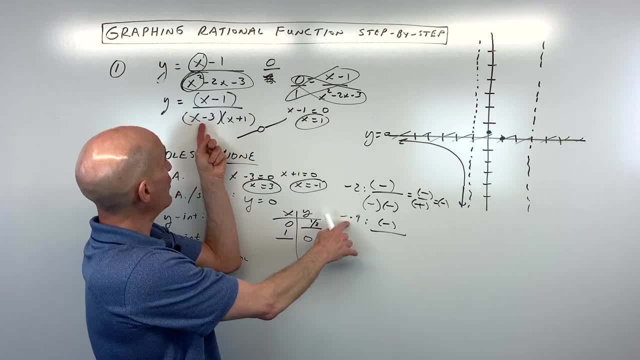 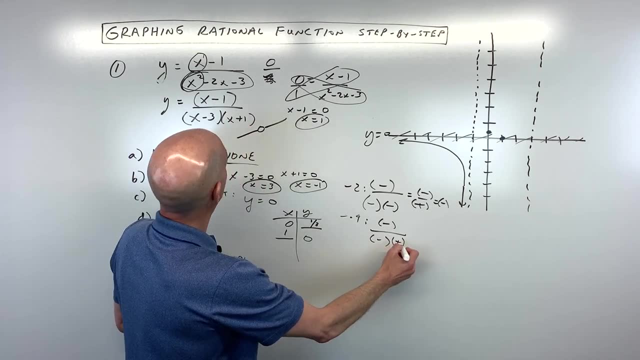 which is just negative, Negative. 0.9 minus 3 is negative 3.9.. That's negative And negative. 0.9 plus 1 is positive 0.1.. Right, So that comes out to a negative And a negative. 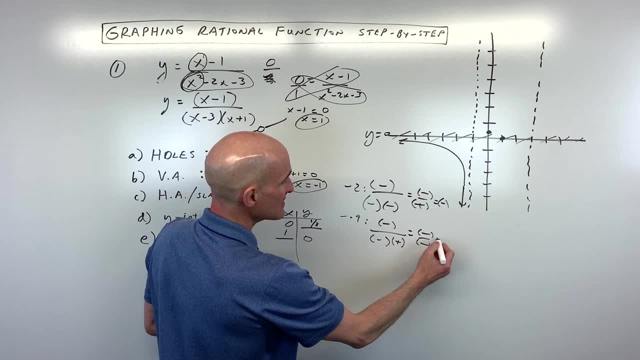 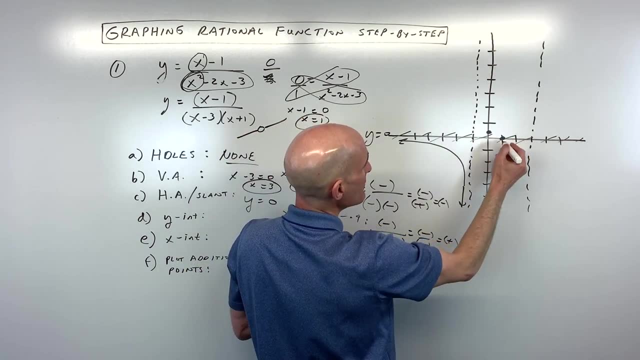 times a positive is a negative And a negative divided by a negative is a positive. That tells us that we're over here at negative 0.9.. This is going up towards positive infinity. You can probably tell that because you see these points going like this. It's going to go like this. 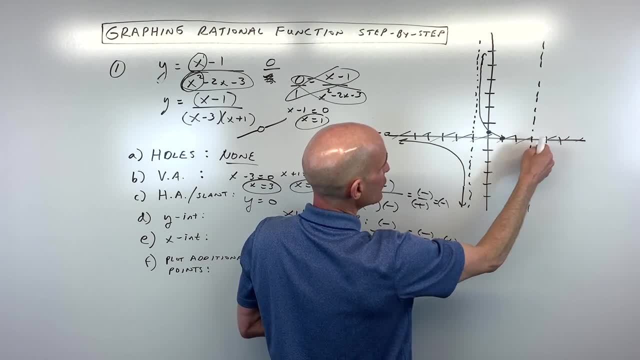 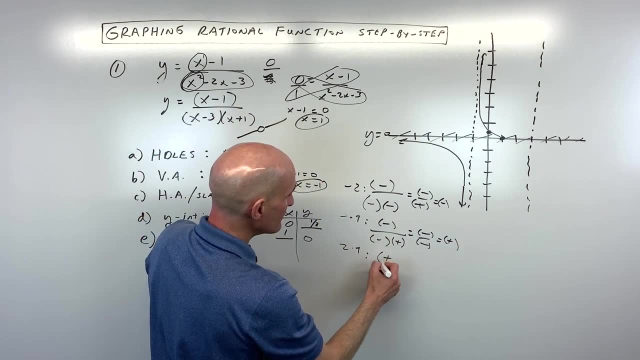 right. Okay, now let's pick some points on either side of this vertical asymptote. Maybe like 2.9 now. So if I put 2.9 in here, 2.9 minus 1 is going to give us a positive value. 2.9 minus 3 is going. 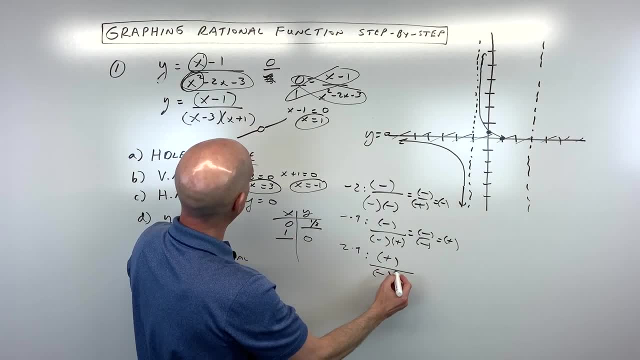 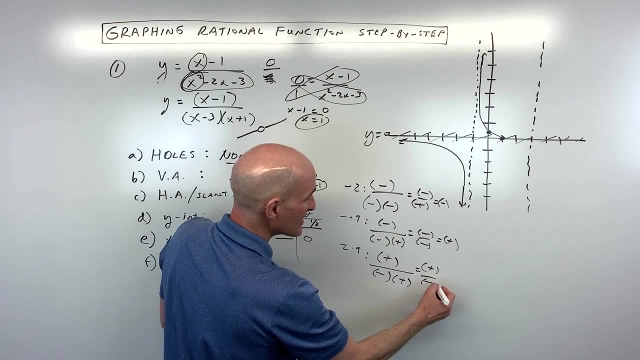 to give us a negative value, And 2.9 plus 1 is going to give us a positive value. So here we get a positive A negative times. a positive is a negative, But a positive divided by a negative is a negative, which means this is going down towards negative infinity, But we probably already. 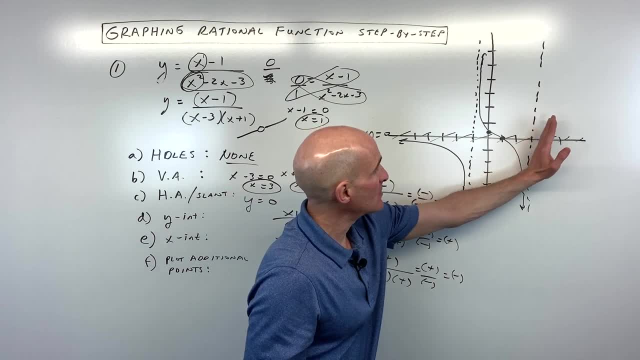 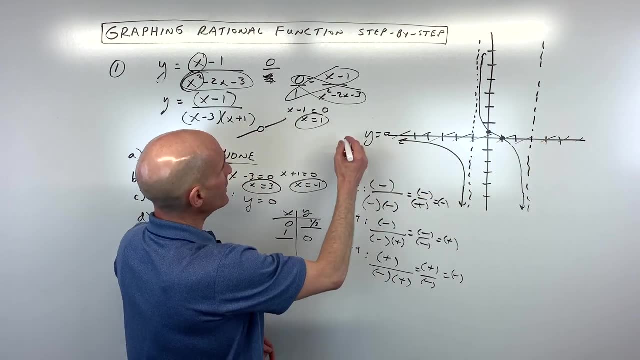 knew that just based on these couple of points here. The last one is to pick over here, just to the right of this vertical asymptote, maybe here at 3.1. Or we could even just do 4.. So if we put 4 in, let's see that's 4 minus 1, which is 3.. That's positive, And 4 minus 3 is 1. That's. 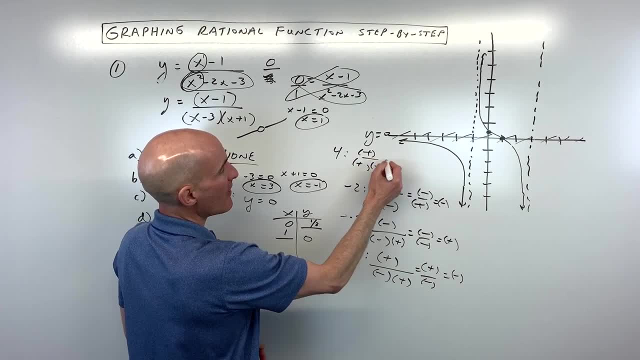 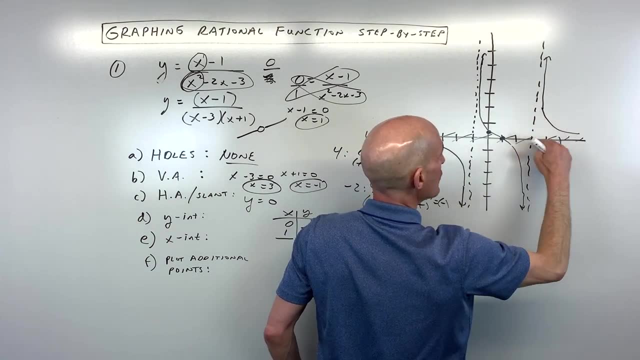 positive And 4 plus 1 is 5. That's positive. So positive divided by positive is a negative Positive And that means that when you're approaching from this side, it's going up towards positive infinity. As you go out here towards the right, it's approaching that x-axis. 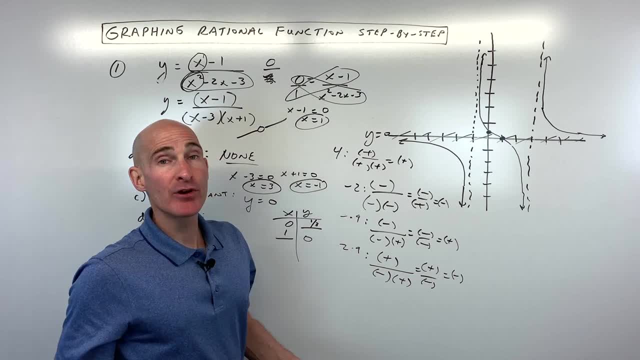 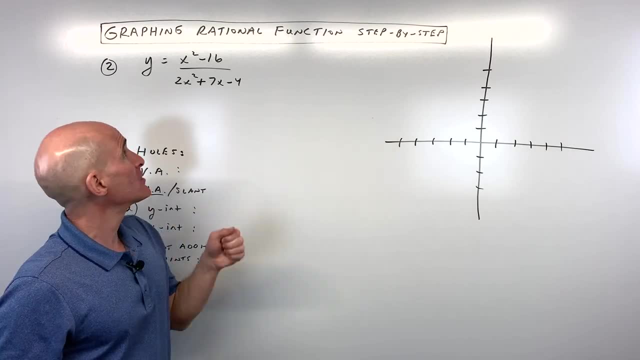 that horizontal asymptote y equals 0.. And we've got a pretty good sketch of the graph, So let's go ahead and do some more challenging examples. Okay, number two: See if you can do this problem on your own. So we've got y equals x squared minus 16, all over 2x squared plus 7x minus 4.. 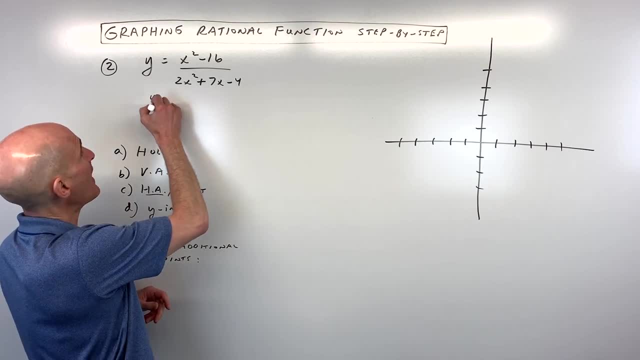 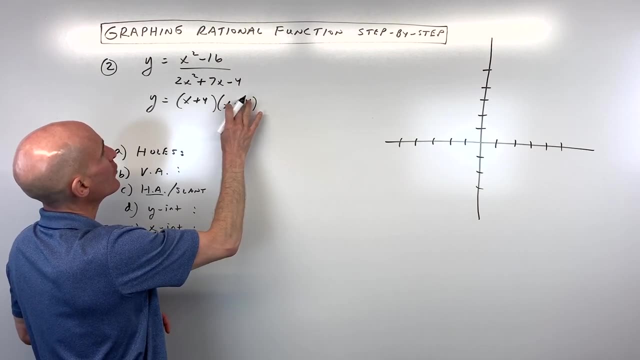 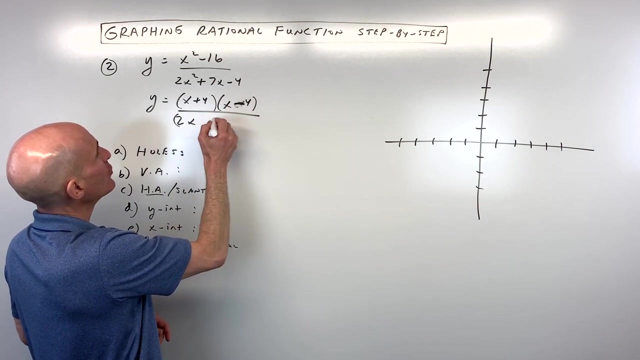 So what's the first step? Well, the first step is: you want to factor it as much as you can. The numerator is a difference of two squares, two perfect squares: x plus 4, x minus 4.. And the denominator is a trinomial with a leading coefficient. that's not. 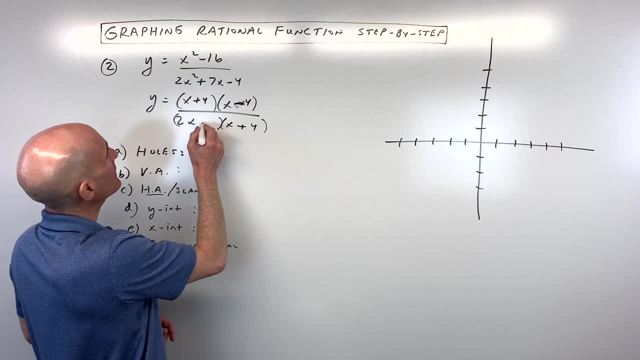 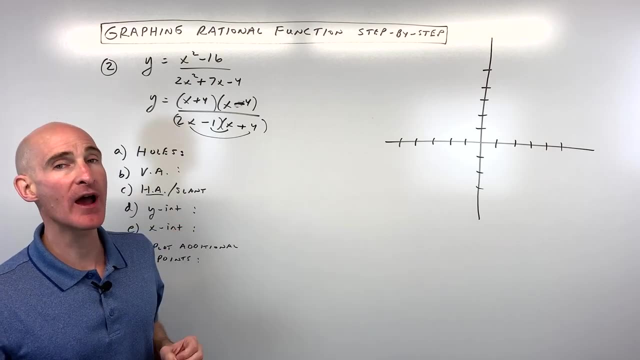 equal to 1.. So this one is going to factor like this: So 8x minus 1x is 7x. Okay, so now what you want to do is you want to analyze it to see if there are any holes in the graph. 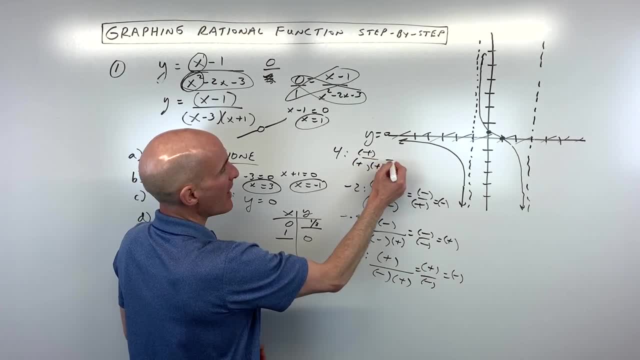 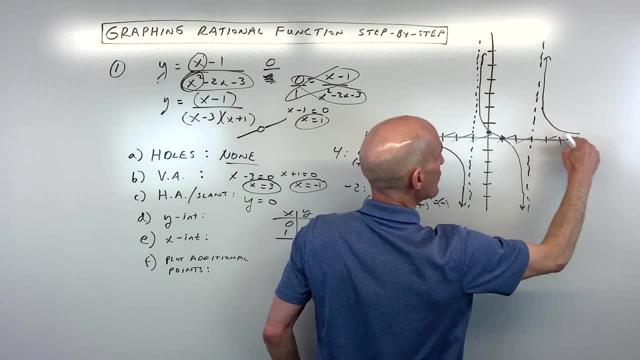 positive And 4 plus 1 is 5. That's positive. So positive divided by positive is a negative Positive And that means that when you're approaching from this side, it's going up towards positive infinity. As you go out here towards the right, it's approaching that x-axis. 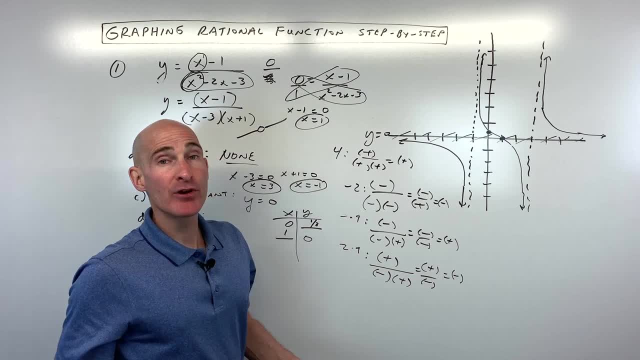 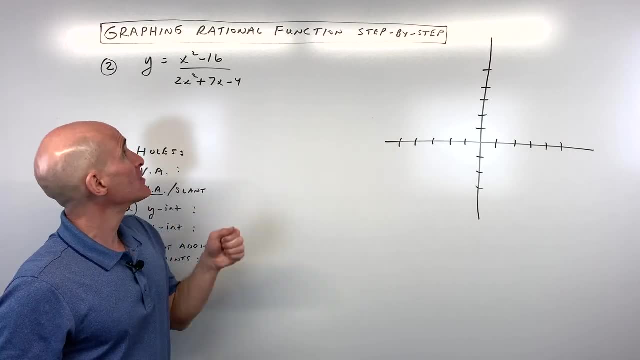 that horizontal asymptote y equals 0.. And we've got a pretty good sketch of the graph, So let's go and do some more challenging examples. Okay, number two, see if you can do this problem on your own. So we've got y equals x squared minus 16, all over 2x squared plus 7x minus 4.. 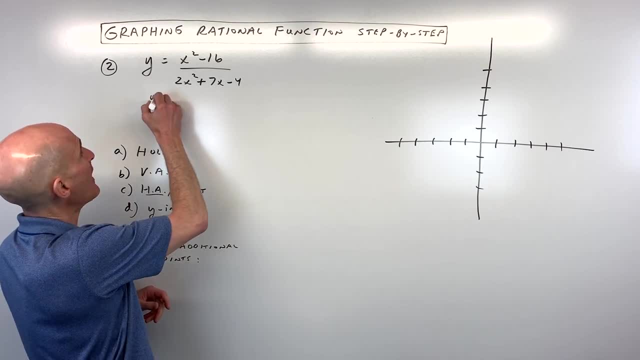 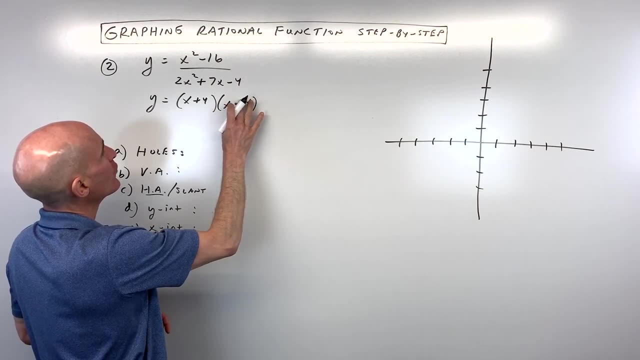 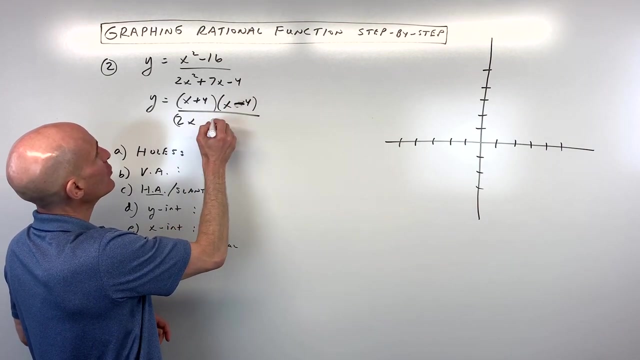 So what's the first step? Well, the first step is: you want to factor it as much as you can. The numerator is a difference of two squares, two perfect squares: x plus 4, x minus 4.. And the denominator is a trinomial with a leading coefficient. that's not. 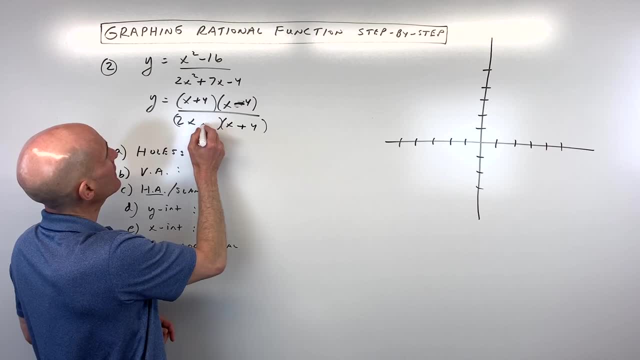 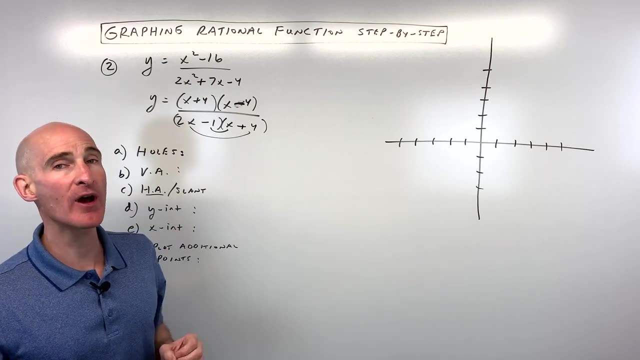 equal to 1.. So this one is going to factor like this: So 8x minus 1x is 7x. Okay, so now what you want to do is you want to analyze it to see if there are any holes in the graph. 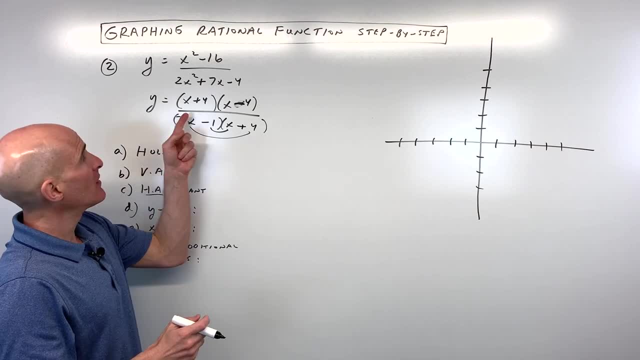 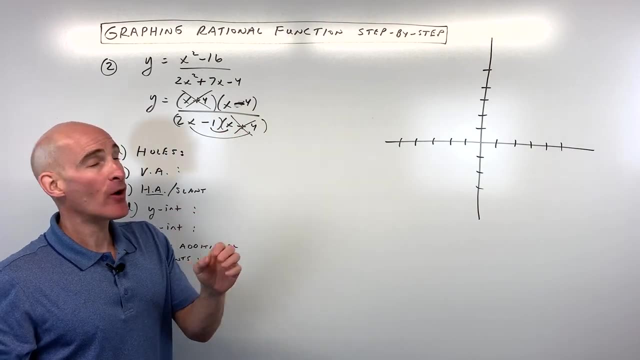 And remember, the holes occur when there's a factor in the numerator that cancels with a factor in the denominator, which is exactly what we have here. We've got x plus 4, x plus 4.. But to find the location of that hole, what you want to do is you want to. 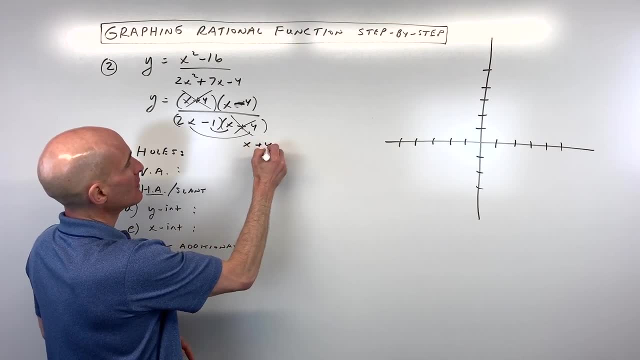 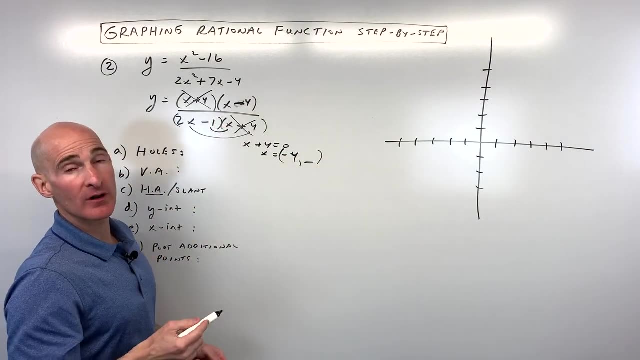 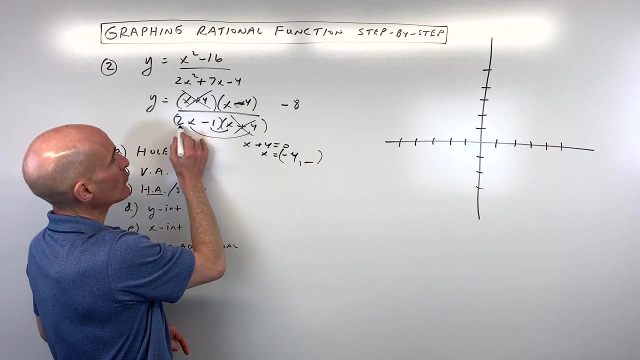 set x plus 4 equal to 0, solve for x. that's negative 4.. And then if you take negative 4 and put it back into what's left over in that equation, that'll give us our y-coordinate of our hole. So if we do that, we get negative 4 minus 4, which is negative 8.. Negative 4 times. 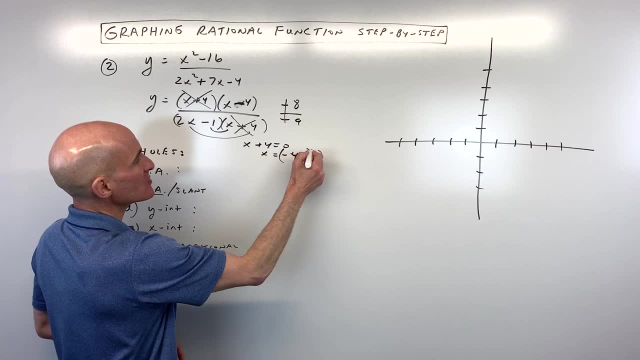 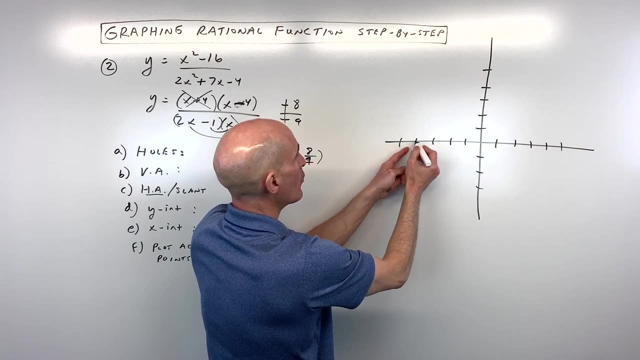 2 is negative, 8 minus 1 is negative 9.. And two negatives cancel. so we're going to get negative 4 comma 8, ninths. So that's going to be- let's see right here- 1,, 2,, 3,, 4, and 8. 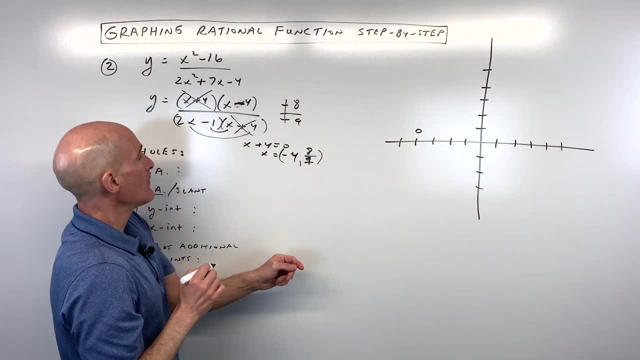 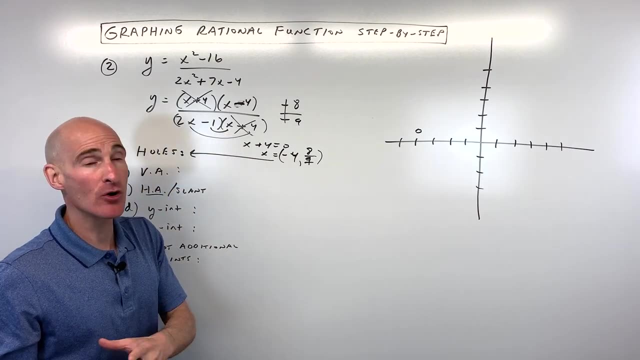 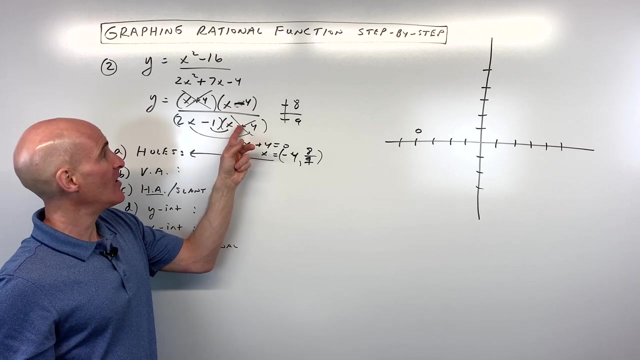 ninths is going to be right about here. Okay, so now let's go to the vertical asymptotes. So the vertical asymptotes, remember, you cannot divide by 0. So by setting these factors in the denominator equal to 0, but not this one, because, remember, this one was where our hole was. okay, you're. 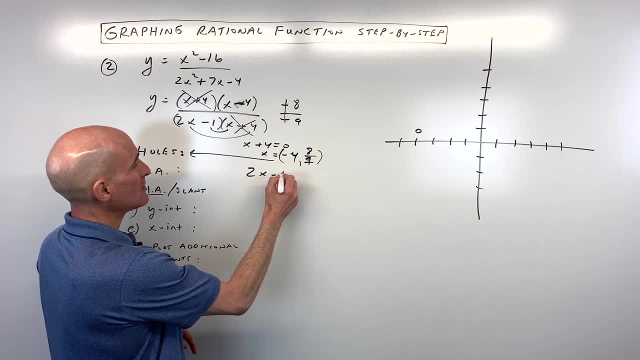 going to find the vertical asymptotes. So here we've got: 2x minus 1 is equal to 2x minus 1, equal to 0, add 1 to both sides and divide by 2.. So you can see, x cannot equal 1 half. 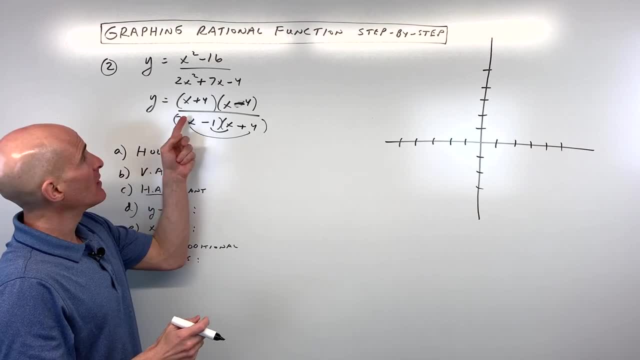 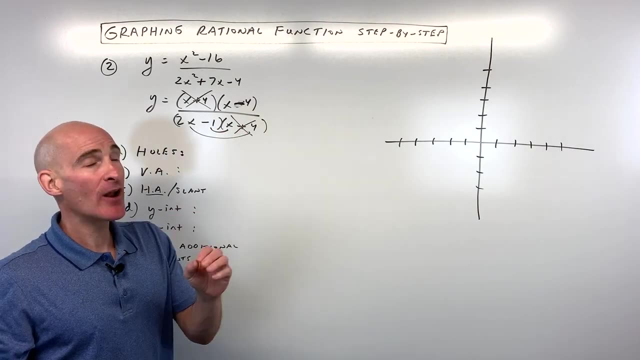 And remember, the holes occur when there's a factor in the numerator that cancels the factor in the denominator, which is exactly what we have here. We've got x plus 4, x plus 4.. But to find the location of that hole, what you want to do is you want to set x plus 4. 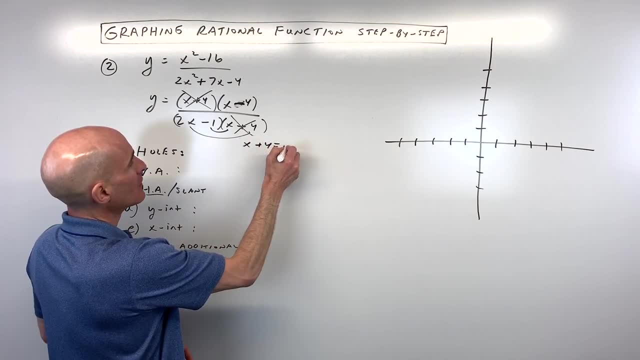 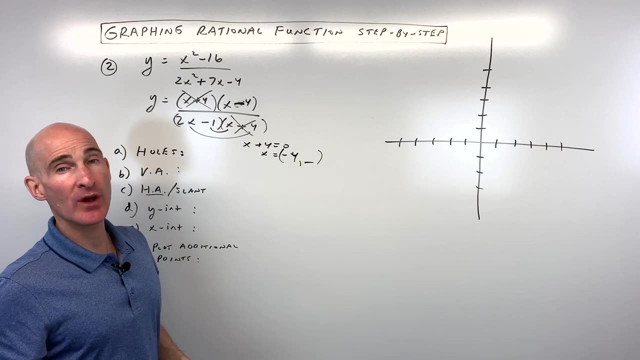 equal to 0, solve for x, that's negative 4.. And then if you take negative 4 and put it back into what's left over in that equation, that'll give us our y coordinate of our hole. So if we do that, 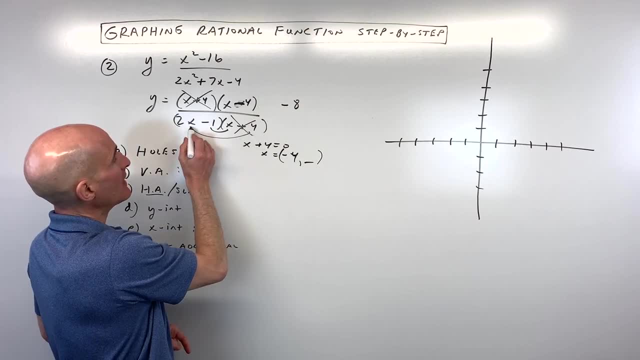 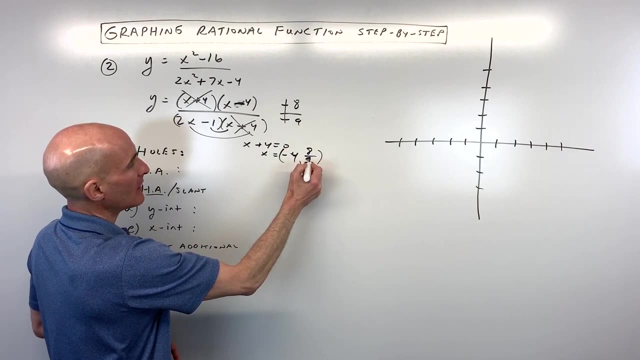 we get negative 4 minus 4, which is negative 8.. Negative 4 times 2 is negative. 8 minus 1 is negative 9.. Two negatives cancel. So we're getting negative 4 comma 8 ninths. So that's going to be. let's see right here. 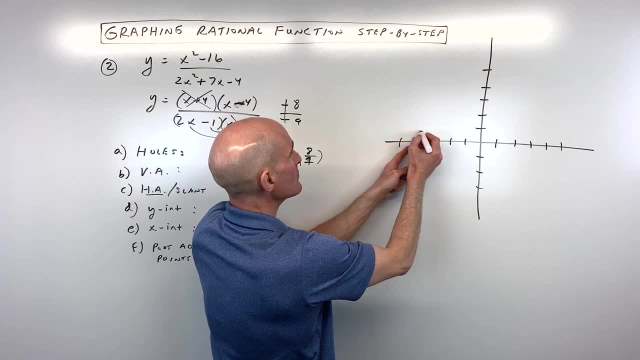 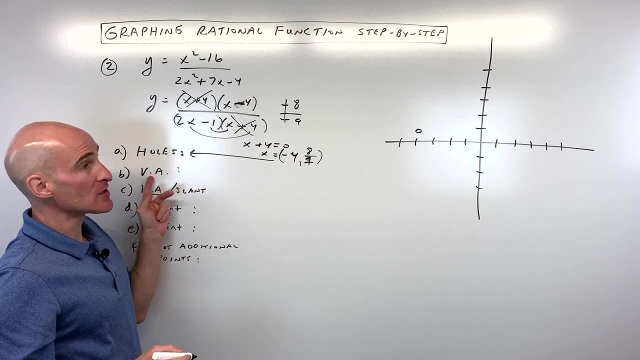 1,, 2,, 3,, 4, and 8. ninths is going to be right about here. Okay, so now let's go to the vertical asymptotes. So the vertical asymptotes, remember, you cannot divide by 0. So by setting these: 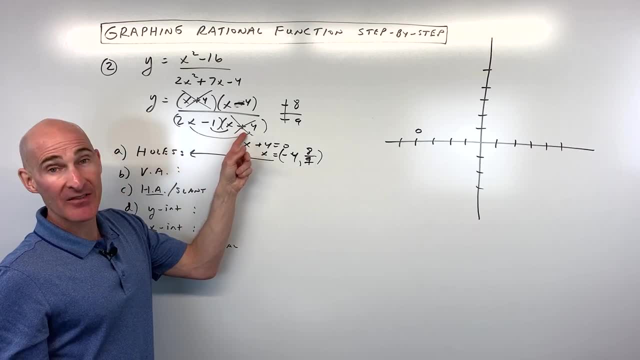 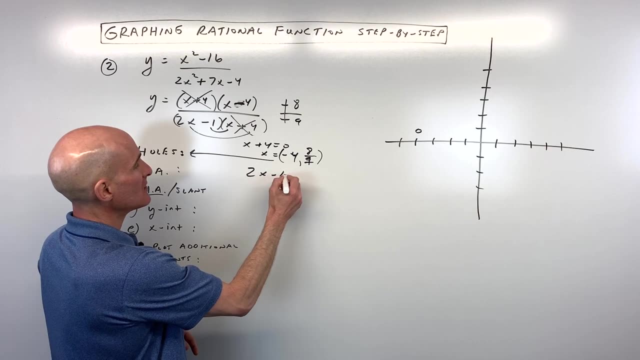 factors in the denominator equal to 0, but not this one, because remember this one was where our hole was. okay, you're going to find the vertical asymptotes. So here we've got: 2x minus 1, is equal to 0, add 1 to both sides and divide by 2.. So you can see, x cannot equal 1 half. 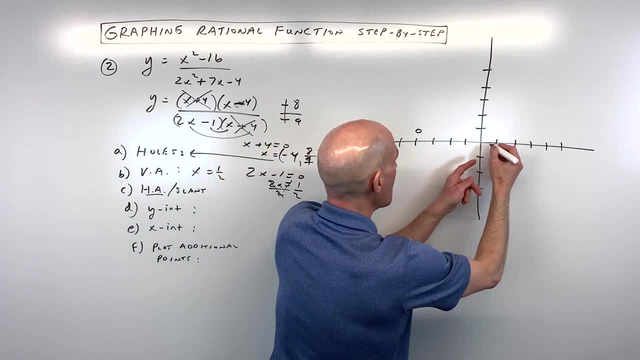 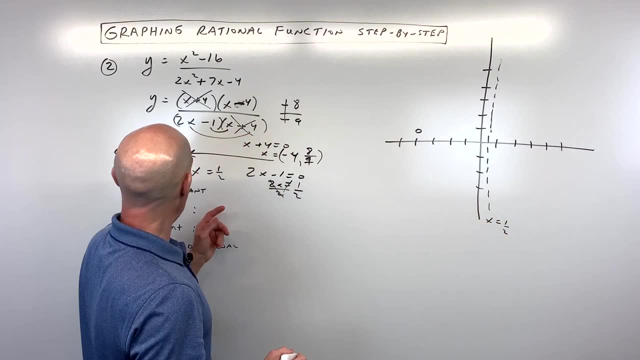 And that's going to be our vertical asymptote. 1 half is right here. Okay, x equals 1 half. And again, remember this: one can't be a vertical asymptote. It's either going to be a hole or a vertical asymptote. It can't be both. It's one or the other, Of course. 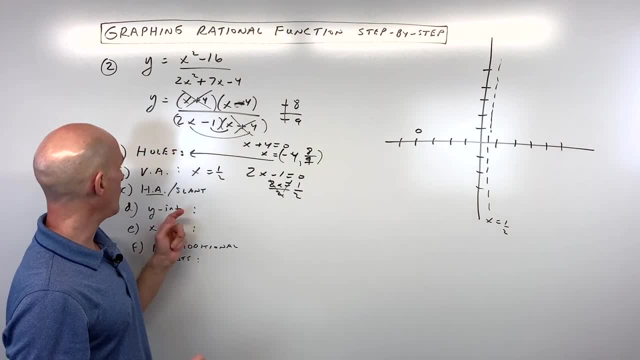 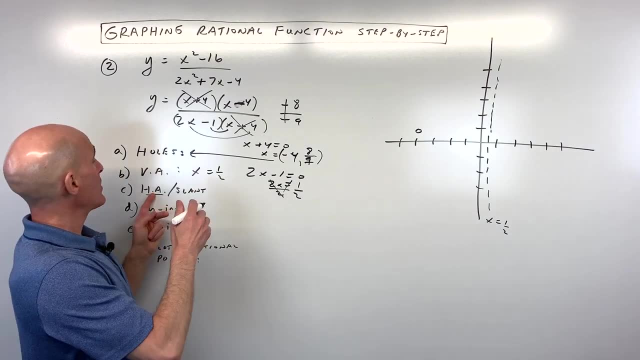 x cannot be negative 4.. But again we saw that as a removable point. So for letter c we want to analyze whether it's a horizontal asymptote or a slant asymptote. So here what we do is we zero in on the highest degree term in the numerator, the highest degree. 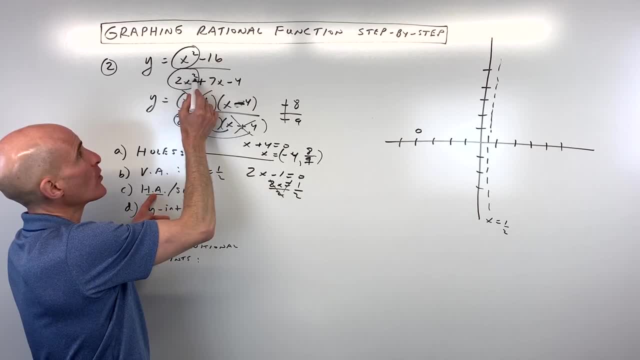 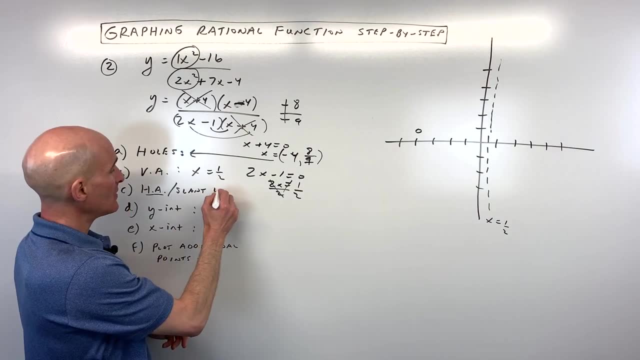 term in the denominator And notice it's a tie. These are both x squared. So when it's a tie like that, you want to look at the ratio of the coefficients in front of those terms. That's 1 over 2.. That's going to be: y equals 1 half, which is going to be right here. 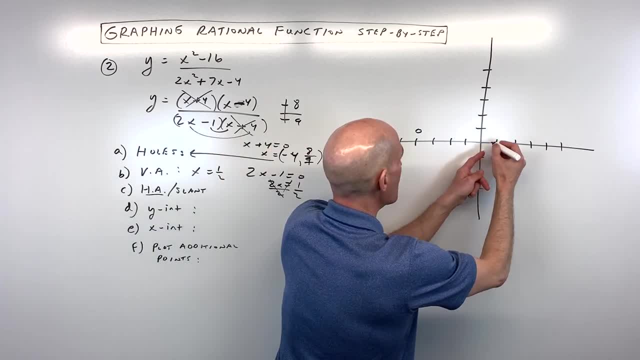 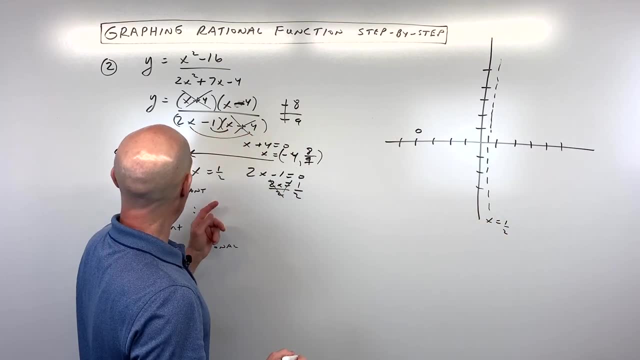 And that's going to be our vertical asymptote. 1 half is right here. Okay, x equals 1 half. And again, remember this: one can't be a vertical asymptote. It's either going to be a hole or a vertical asymptote. It can't be both. It's one or the other, Of course. 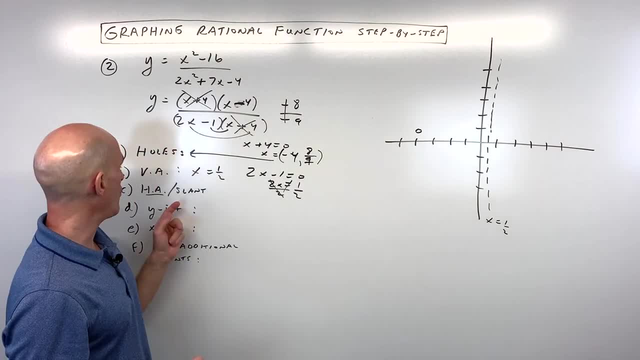 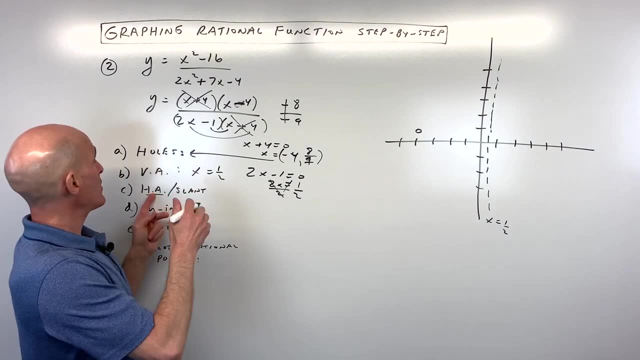 x cannot be negative 4, but again we saw that as a removable point. So for letter c now we want to analyze whether there's a horizontal asymptote or a slant asymptote. So here what we do is we zero in on the highest degree term in the numerator. 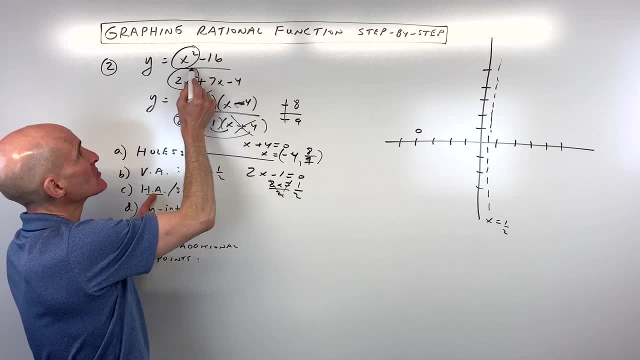 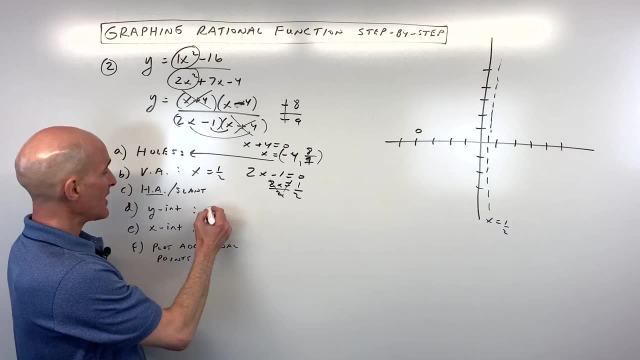 the highest degree term in the denominator And notice it's a tie. These are both x squared. So when it's a tie like that, you want to look at the ratio of the coefficients in front of those terms. That's 1 over 2.. That's going to be: y equals 1 half, which is going to be right here. 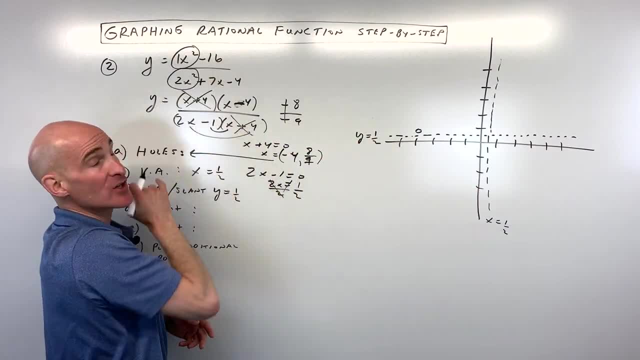 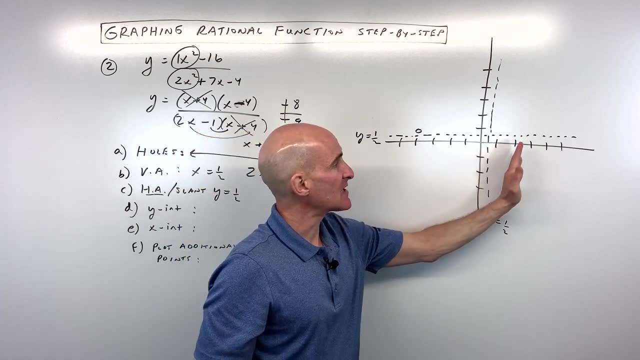 Now you might be saying: Mario, I don't understand. Why is it the ratio of the coefficients? Well, what you can think of is that when you go to the right end of the graph, or the left end of the graph, meaning as x gets larger and larger, 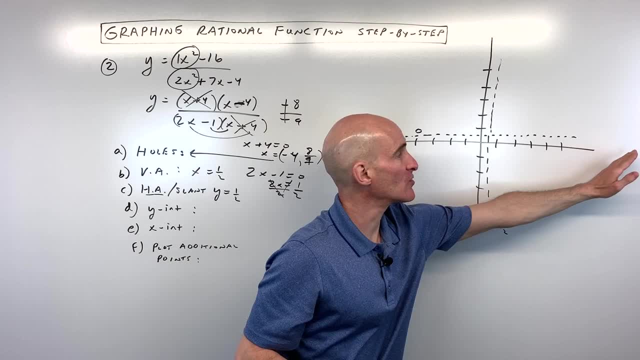 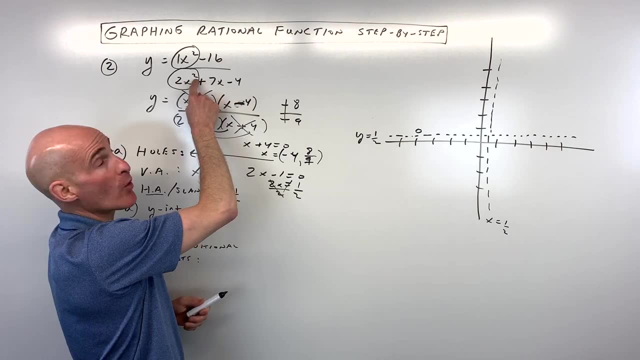 or x gets smaller and smaller towards negative infinity, or x approaches positive infinity. the negative 16 and the negative 4 doesn't change. The 7x is not growing as fast as x squared. So what happens is: you can do this on your calculator. 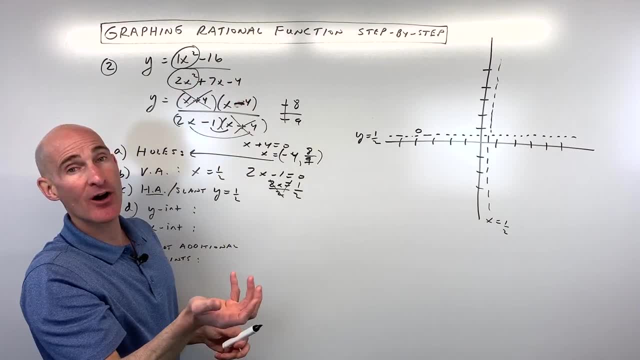 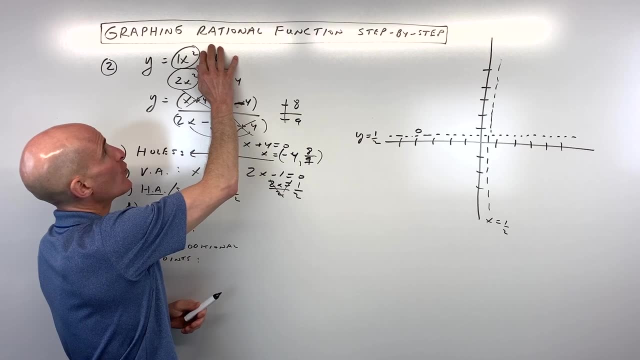 Put in a large value for x, maybe like 100, or then maybe try 1,000. And what you'll notice is because these terms are growing much faster than these terms as x gets bigger and bigger. it's really just going to look like 1x over 2x squared. 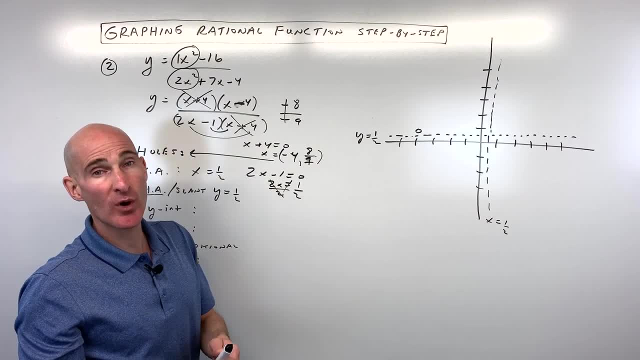 1x squared over 2x squared, The x squareds are going to cancel and you're going to just be left with y equals 1 half And you can just do that experiment and you'll see that that's approaching 1 half. 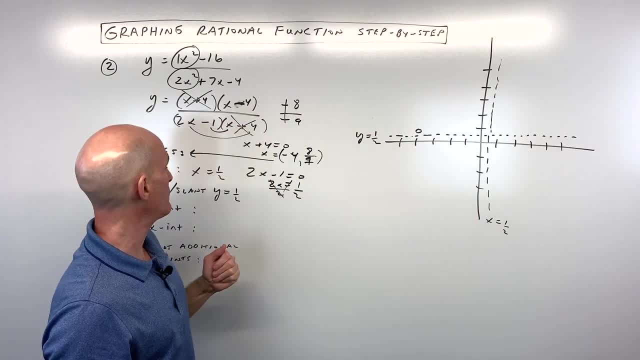 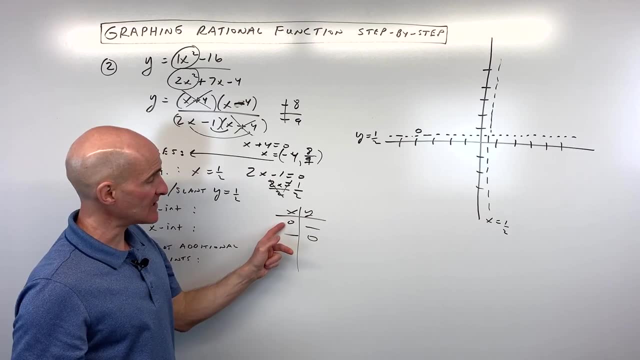 as x gets really large positive or a really large negative number. Okay, so now for the y-intercepts and the x-intercepts. What you want to do is you want to make a table, You want to set x equal to 0 to find the y-intercept. 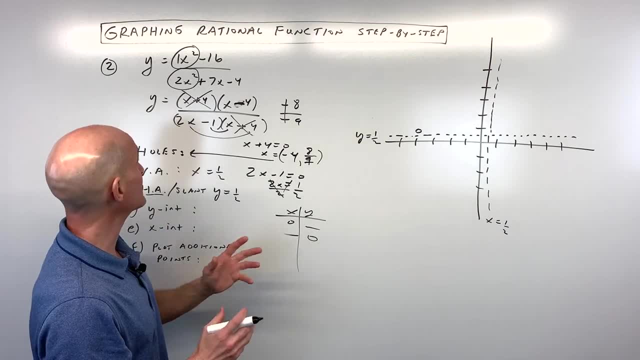 and y equal to 0 to find the x-intercept. So it's kind of like setting the opposite variable equal. So here if we put 0 in for x, it's going to cancel out this term, this term and this term. 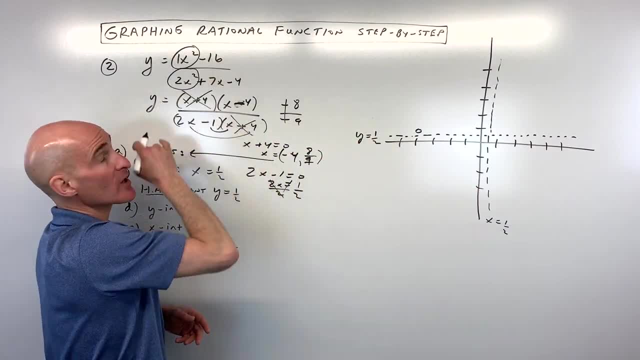 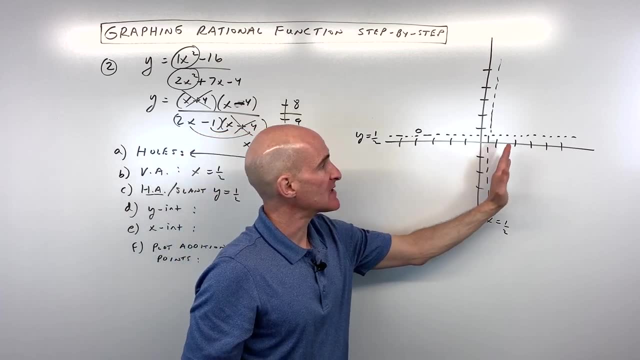 Now you might be saying: Mario, I don't understand. Why is it the ratio of the coefficient? Well, what you can think of is that when you go to the right end of the graph or the left end of the graph, meaning as x gets larger and larger, or x gets smaller and smaller, towards negative, 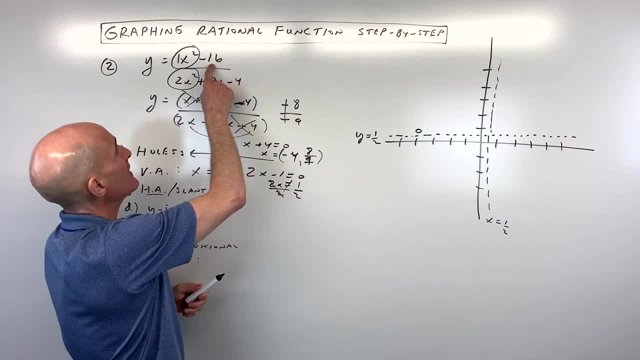 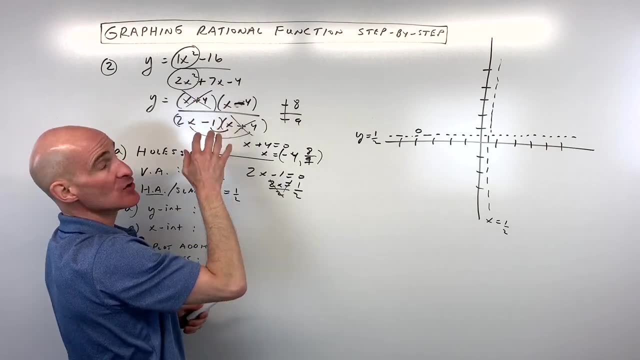 infinity, or x approaches positive infinity, the negative 16 and the negative 4 doesn't change. The 7x is not growing as fast as x squared. So what happens is you can do this on your calculator: Put in a large value for x, like, maybe like 100, or then maybe try 1000.. And what you'll notice? 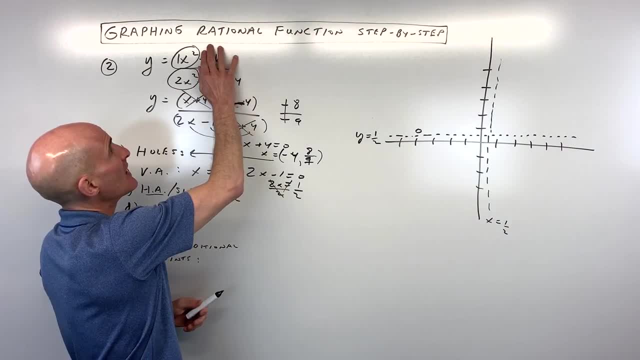 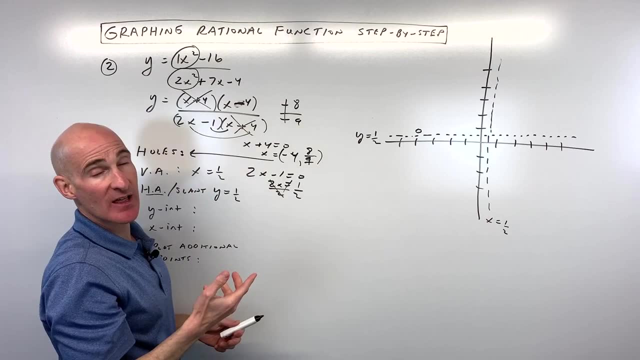 is because these terms are growing much faster than these terms. as x is bigger and bigger, it's really just going to look like 1x over 2x squared, 1x squared over 2x squared. The x-squareds are going to cancel and you're going to just be left with y equals 1 half. 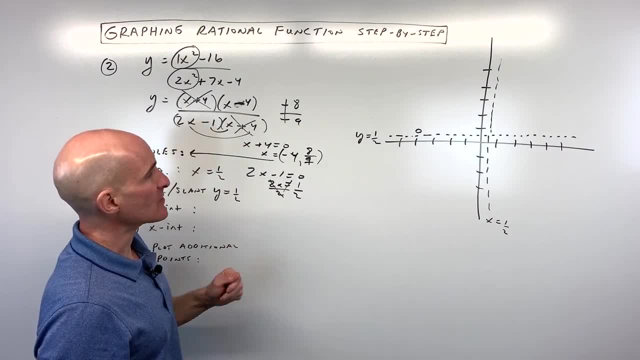 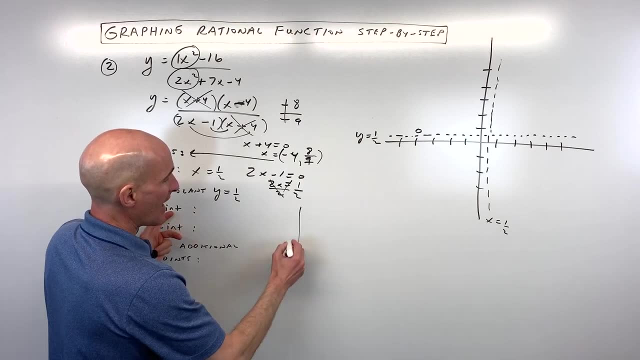 And you can just do that experiment and you'll see that that's approaching 1 half as x gets really large positive or really large negative number. Okay, so now for the y-intercepts and the x-intercepts. What you want to do is you want to make a table, You want to set x equal to 0 to find. 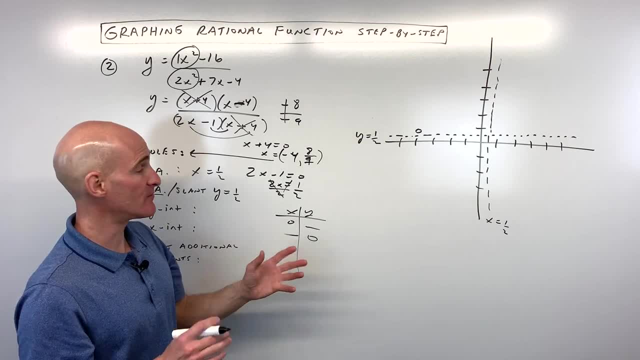 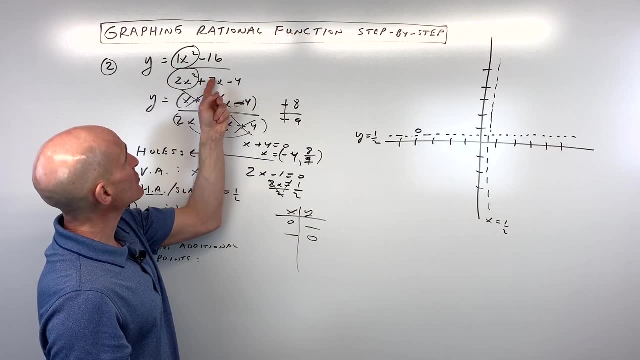 the y-intercept and y equal to 0 to find the x-intercept. So it's kind of like setting the opposite variable equal to 0. So here, if we put 0 in for x, it's going to cancel out this term, this term and this term. 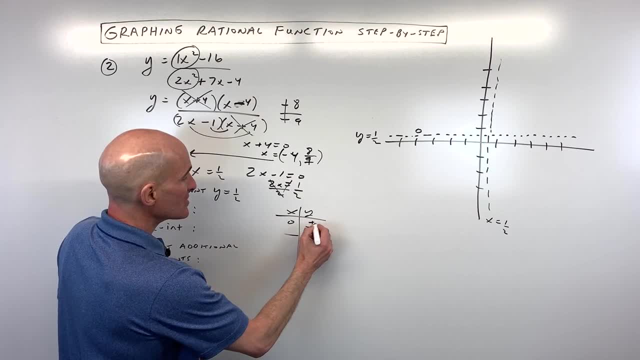 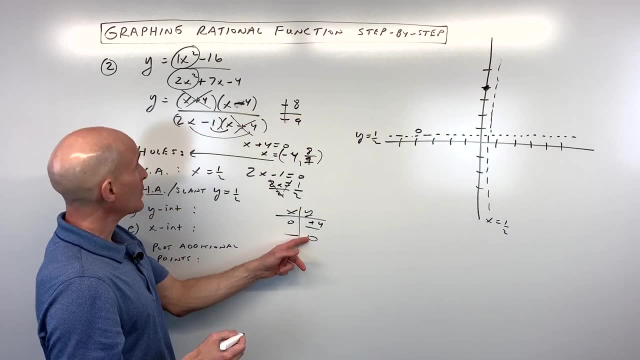 leaving us with negative 16 over negative 4, which is positive 4.. So at 0,, 4, right here that's our y-intercept, And by setting y equal to 0, we can solve for the x-intercept. But remember. 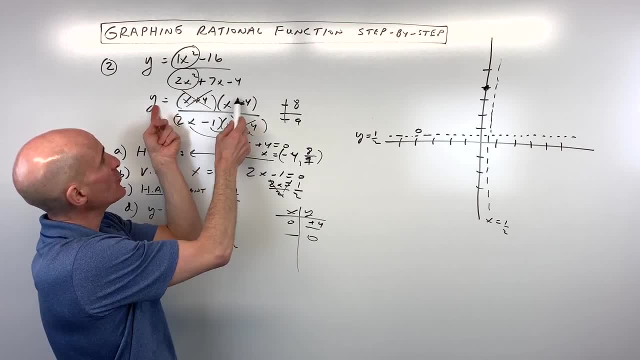 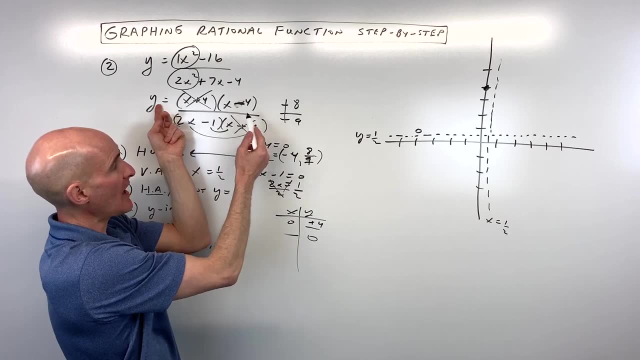 I showed you that shortcut where if you make y 0, that's only going to be possible if these factors in the numerator are equal to 0. So by setting x minus 4 equal to 0,, we get x equals 4.. 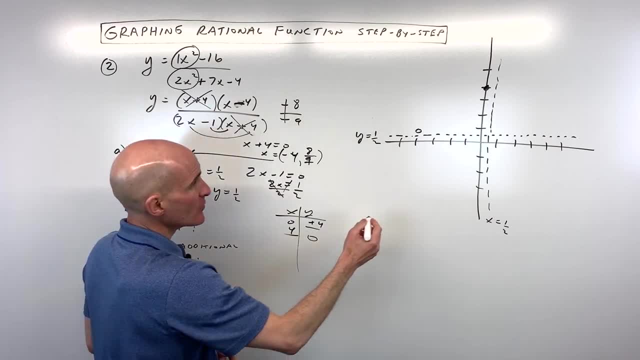 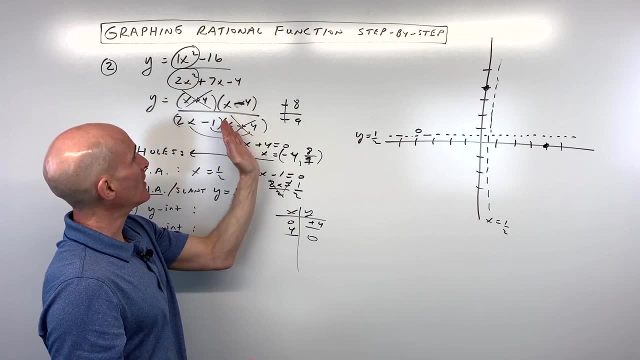 And this one we already canceled out over here. So this is just going to be over here at 1,, 2,, 3,, 4, and that's your x-intercept. Now again, I just wanted to show you when these factors cancel. 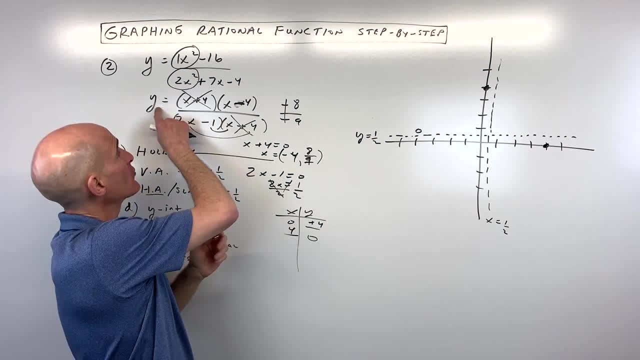 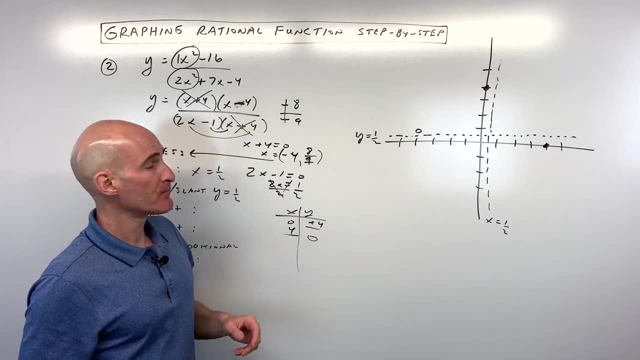 like this. the basic graph is going to be just like the graph of: y equals x minus 4 over 2x minus 1, with the exception of there just being this missing point, that removable point. Okay, now we just want to plot some additional points as needed to get a good graph here. 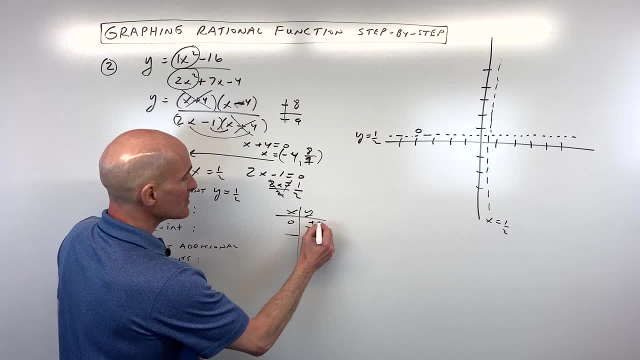 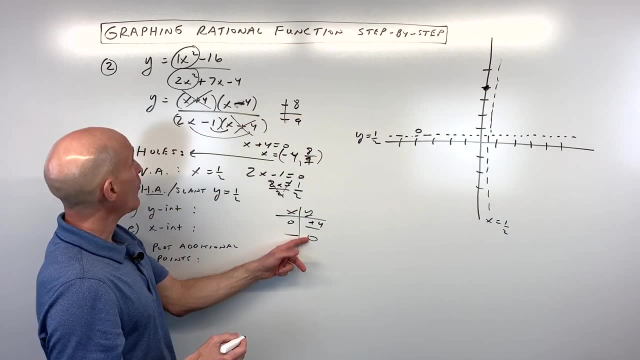 leaving us with negative 16 over negative 4, which is positive 4.. So at 0,, 4,, right here, that's our y-intercept, And by setting y equal to 0, we can solve for the x-intercept. 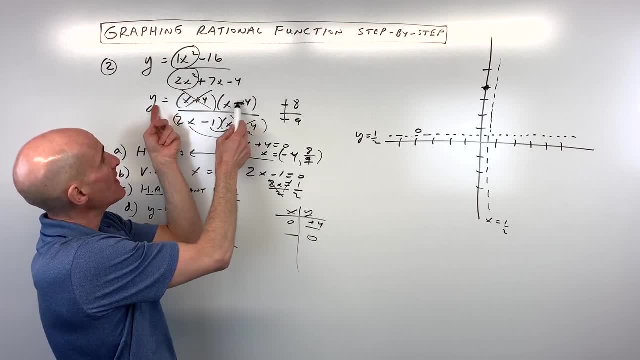 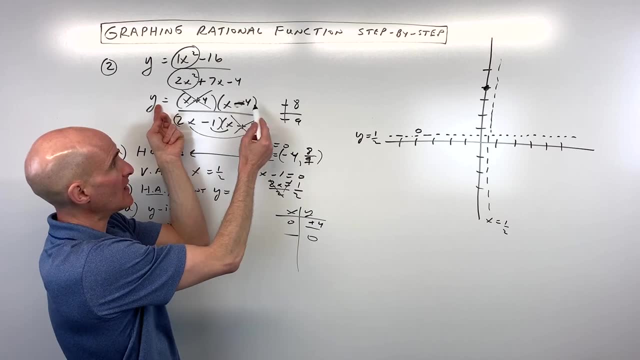 But remember I showed you that shortcut where if you make y 0, that's only going to be possible if these factors in the numerator are equal to 0. So by setting x minus 4 equal to 0, we get x equals 4.. 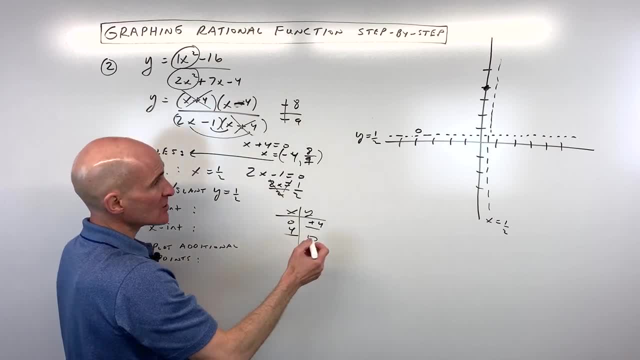 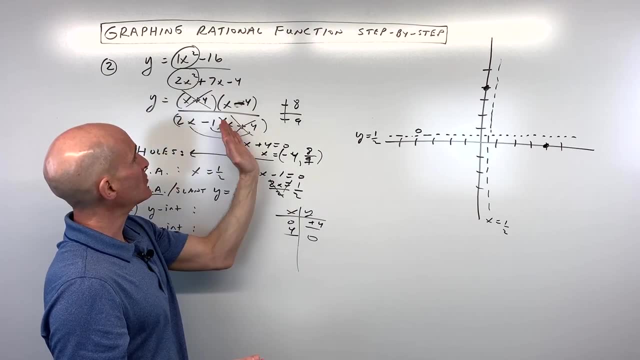 And this one we already canceled out over here. So this is just going to be over here at 1,, 2,, 3,, 4, and that's your x-intercept. Now again, I just wanted to show you when these factors cancel like this: 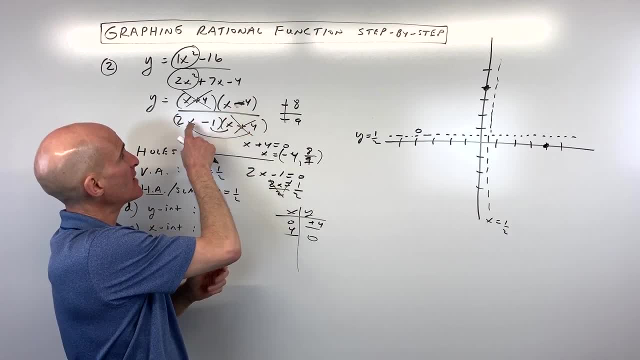 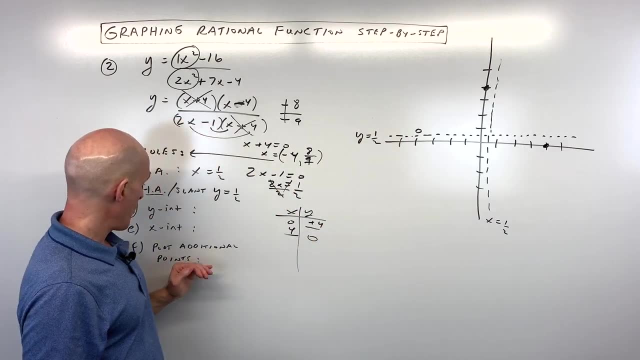 the basic graph is going to be just like the graph of: y equals x minus 4 over 2x minus 1, with the exception of there just being this missing point, that removable point. Okay, now we just want to plot some additional points, as needed to get a good graph here. 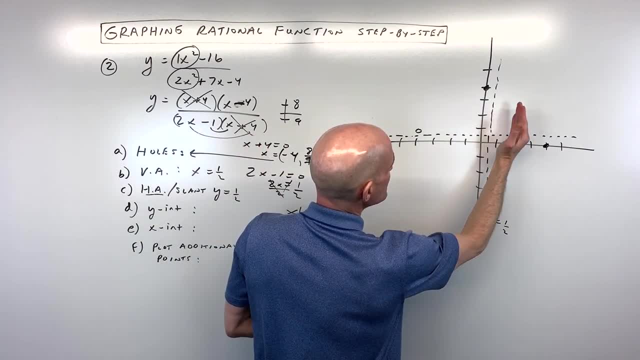 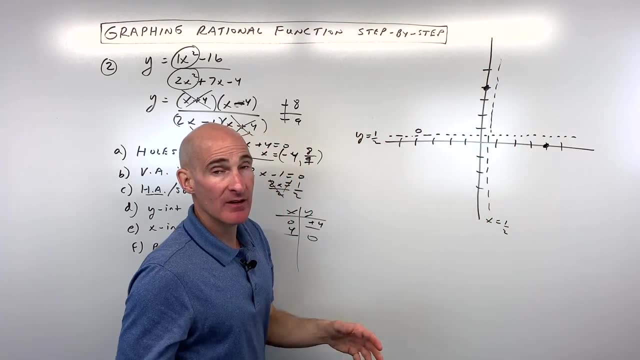 And again, remember our little strategy. We said if we can pick some points. We said if we can pick some points on either side of the vertical asymptote to figure out whether the graph is going up towards positive infinity or down towards negative infinity. 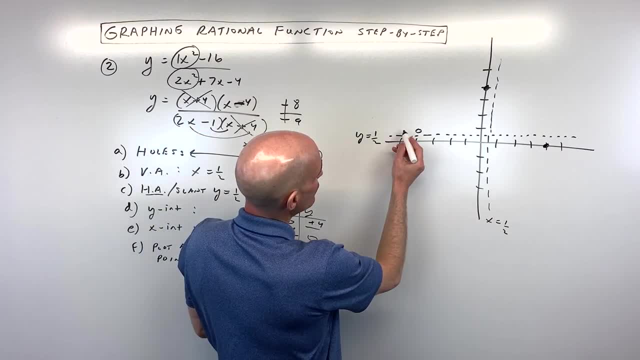 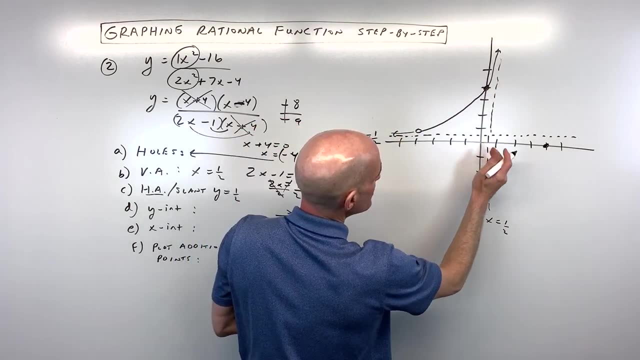 that will be a big help. But here, for this one, you can see that the graph is going like this and like this, right? So we've already got that branch of the graph Over here. let's just verify. Let's maybe pick: x equals 1.. 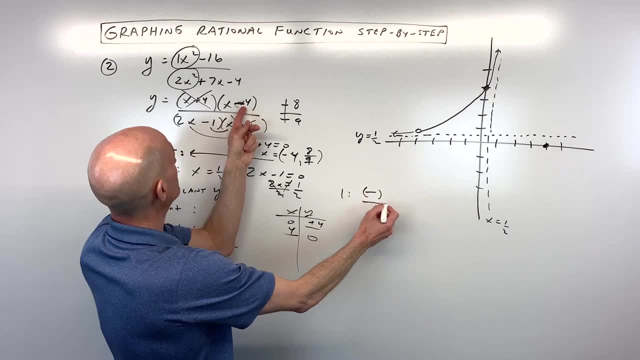 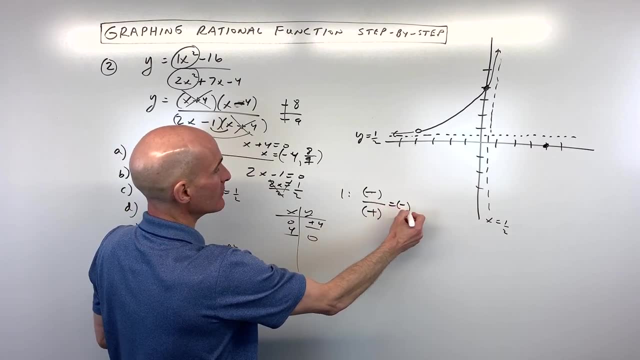 1 minus 4 is negative, 3, negative, And 2 times 1 is 2 minus 1 is positive 1, so that's positive And negative. divided by positive is a negative. So that tells us over here at 1, this is going to be approaching negative infinity. 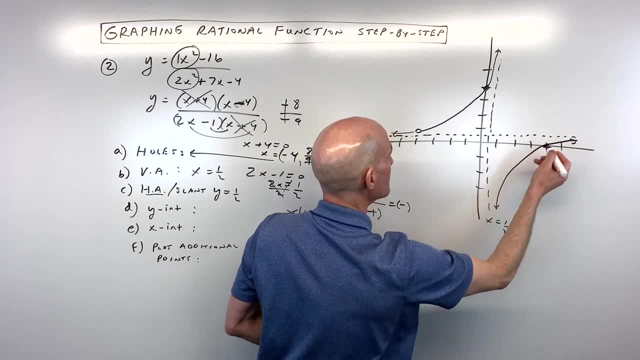 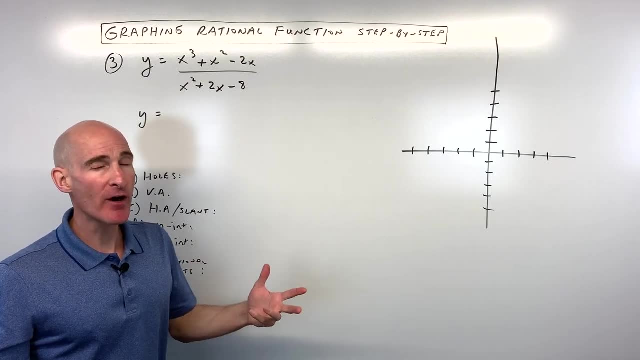 So you can see that the graph is going to look something like that And you got it Okay. number 3. See if you can do this one on your own. This is also a unique example, different from the other two that we've covered so far in this video. 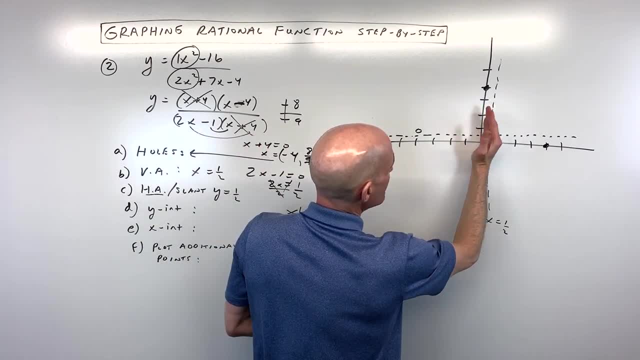 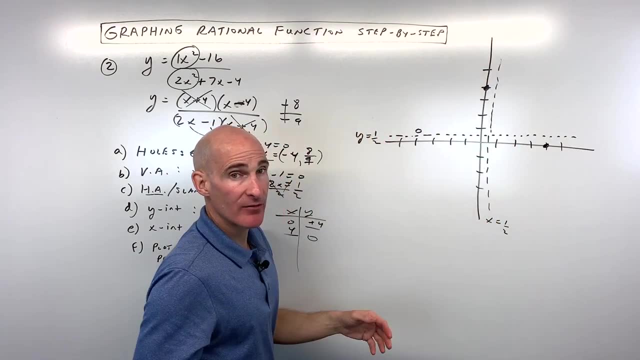 And again, remember our little strategy. We said if we can pick some points on either side of the vertical asymptote to figure out whether the graph is going up towards positive infinity or down towards negative infinity, that will be a big help. But here for this one, you can see that 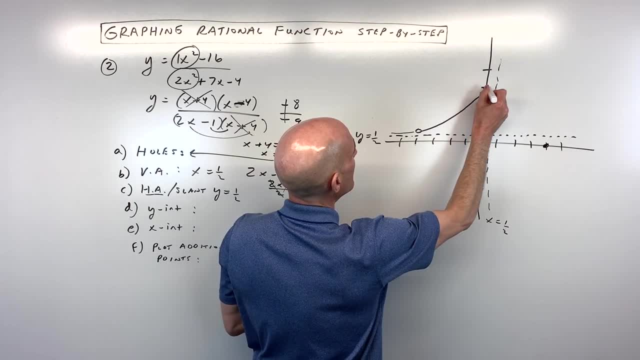 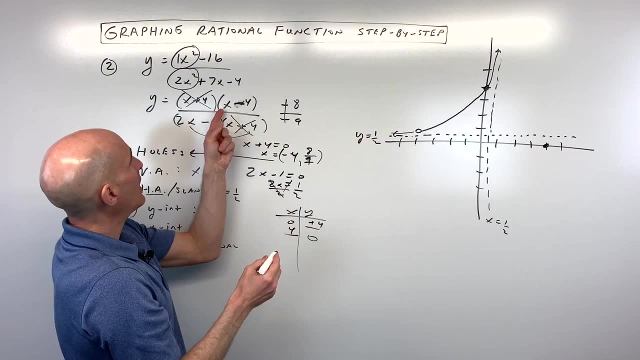 the graph is going like this and like this, right? So we've already got that branch of the graph Over here. let's just verify. Let's maybe pick: x equals 1.. 1 minus 4 is negative 3,. 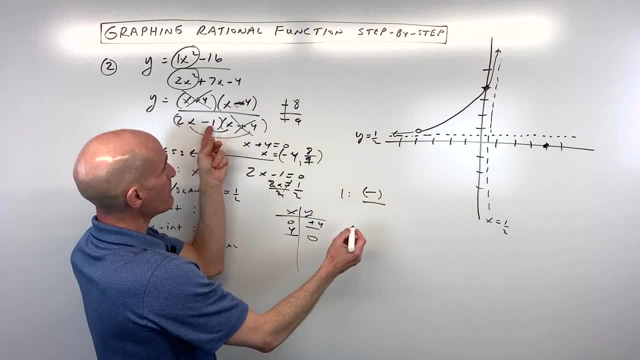 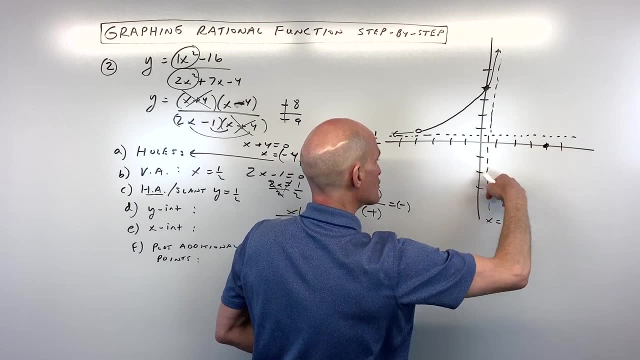 negative, And 2 times 1 is 2 minus 1 is positive 1, so that's positive And negative. divided by positive is a negative. So that tells us over here at 1, this is going to be approaching negative infinity. 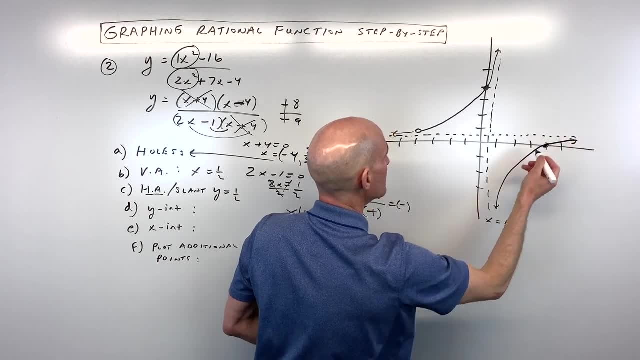 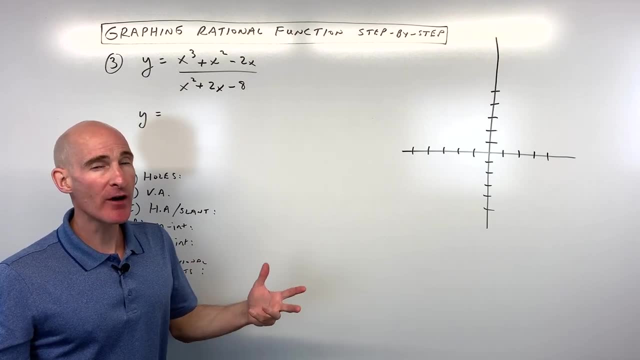 So you can see that the graph is going to look something like that And you got it Okay. number three: See if you can do this one on your own. This is also a unique example, different from the other two that we've covered so far in this video. We've got y equals x cubed plus x squared, minus 2x. 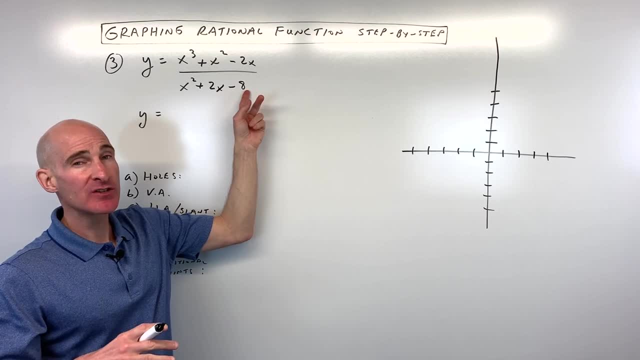 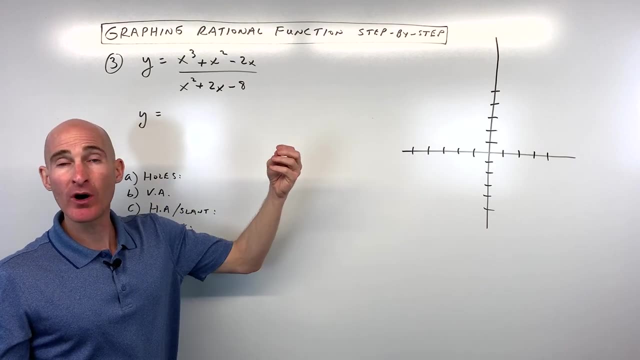 all over x squared plus 2x minus 8.. And before I jump into this problem, I just want to mention, if you like my teaching style, be sure to check out my video courses. I've got courses for Algebra 1,, Algebra 2, ACT math, SAT math. Go ahead and check out those courses. 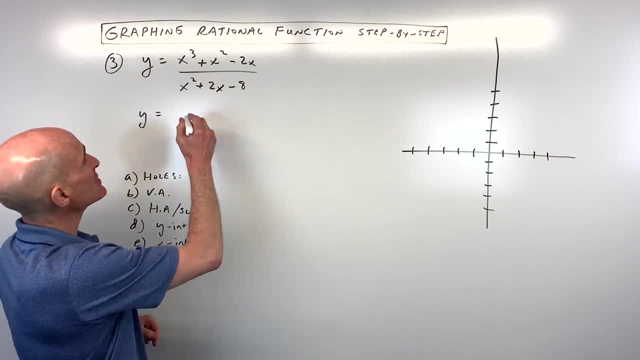 But let's dive into this example. now We've got the first thing is to factor right. So you can see, you can factor out an x out of all these. So that's going to be x squared plus x minus 2.. 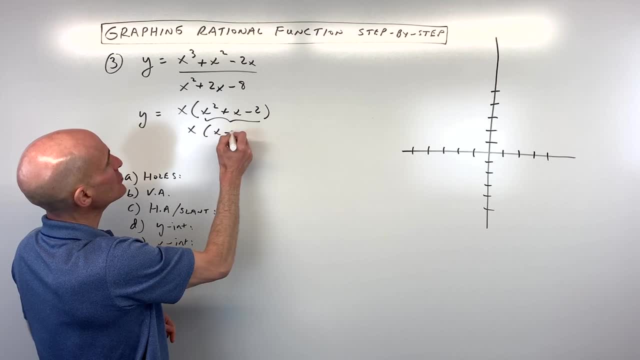 And then you can factor this part here a little bit further into x plus 2 and x minus 1.. So now the denominator is fairly easy to factor. This is just going to be x plus 4 and x minus 1.. And then you can factor this part here a little bit further into x plus 2 and x minus 1.. So now the denominator is fairly easy to factor. This is just going to be x plus 4 and x minus 1.. So now the denominator is fairly easy to factor. This is just going to be x plus 4 and x minus 2.. 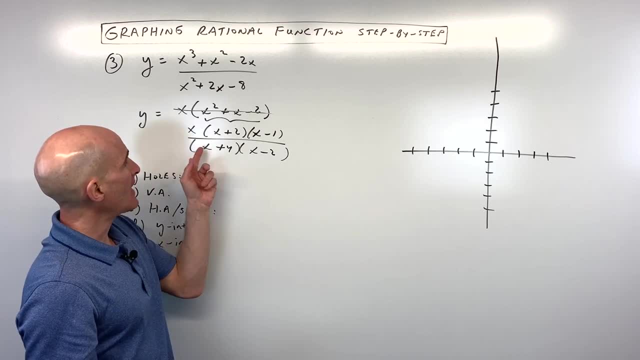 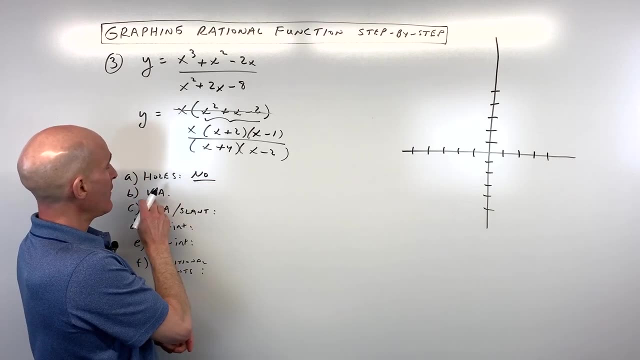 So the first step is to analyze: are there any holes in the graph? Are there any factors in the numerator that cancel with any factors in the denominator? In this case, there's not, So we're just going to say: no holes. okay For vertical asymptotes. now we want to look at the 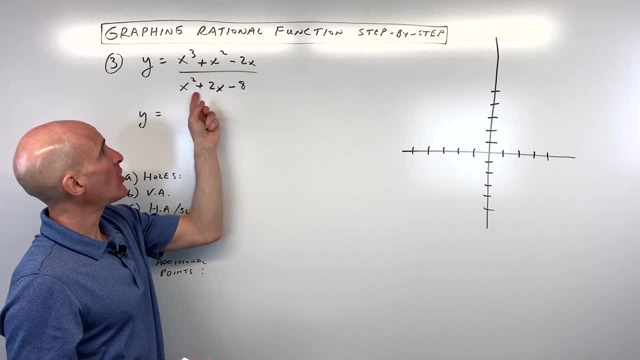 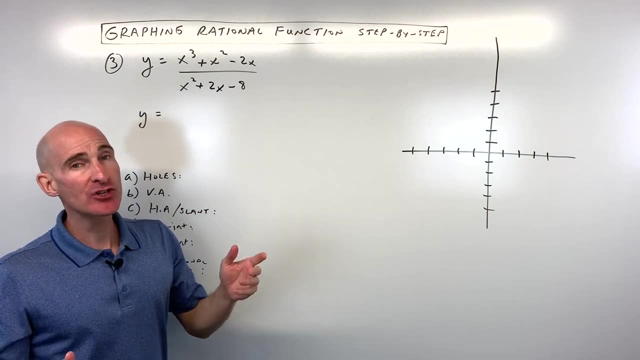 We've got y equals x cubed plus x squared minus 2x, all over x squared plus 2x minus 8.. And before I jump into this problem, I just want to mention, if you like, my teaching style, be sure to check out my 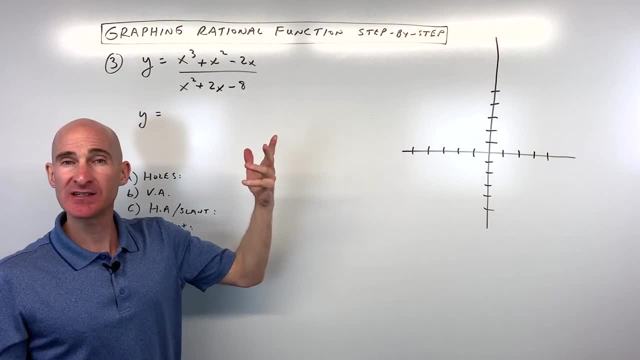 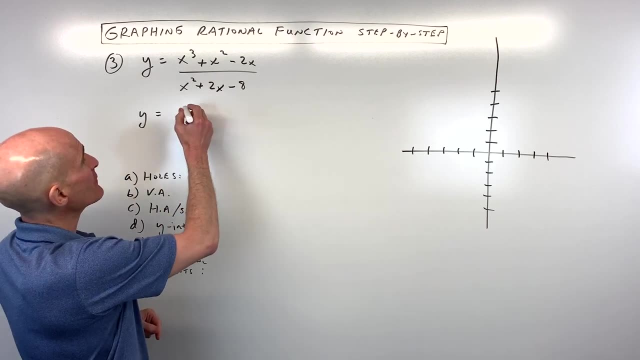 video courses. I've got courses for Algebra 1, Algebra 2, ACT math, SAT math. Go ahead and check out those courses, But let's dive into this example now We've got. The first thing is to factor right. 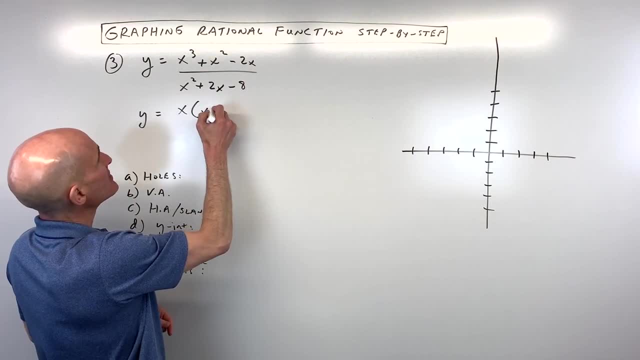 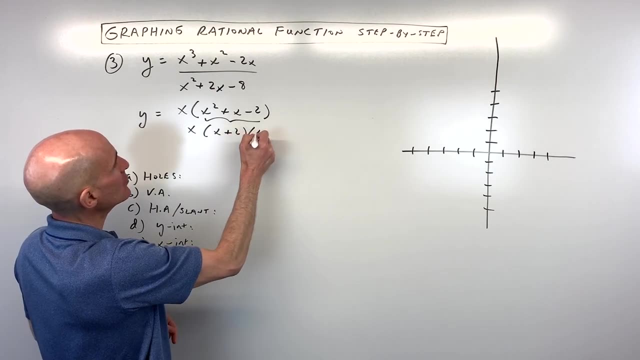 So you can see, you can factor out an x out of all these. So that's going to be x squared plus x minus 2.. And then you can factor this part here a little bit further into x plus 2 and x minus 1.. 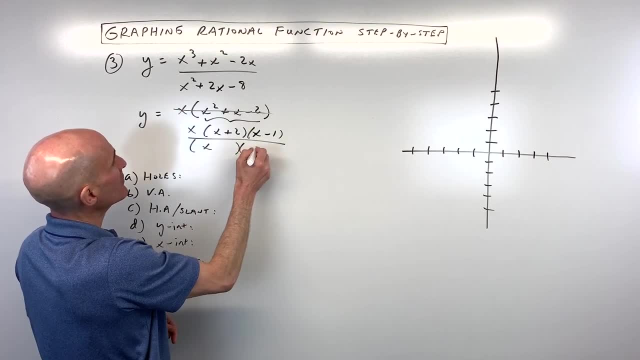 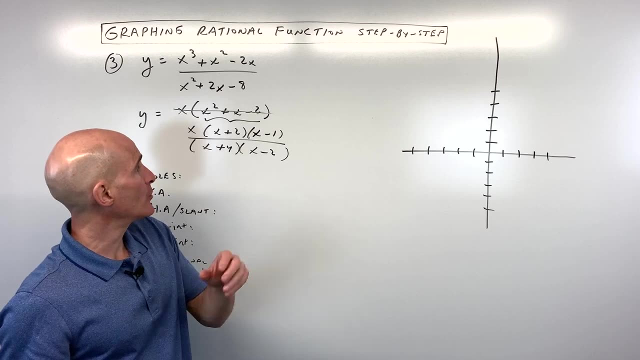 So now the denominator is fairly easy to factor. This is just going to be x squared plus x minus 2.. So now the denominator is fairly easy to factor. This is just going to be x squared plus x minus 2.. So the first step is to analyze: are there any holes in the graph? 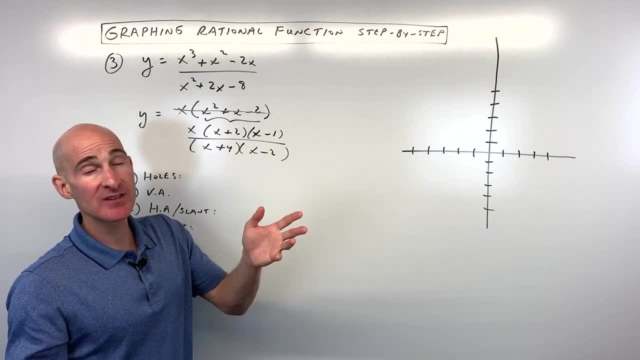 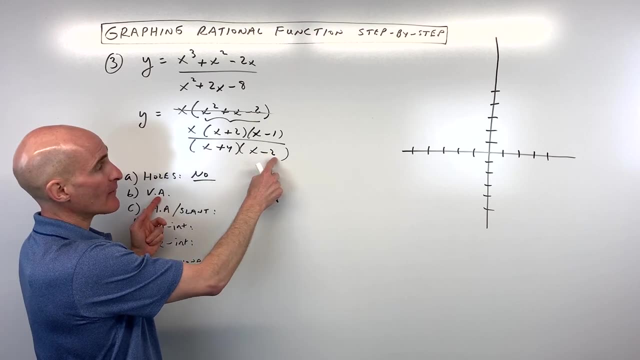 Are there any factors in the numerator that cancel with any factors in the denominator? In this case, there's not, So we're just going to say: no holes. Okay For vertical asymptotes. now we want to look at the denominators. 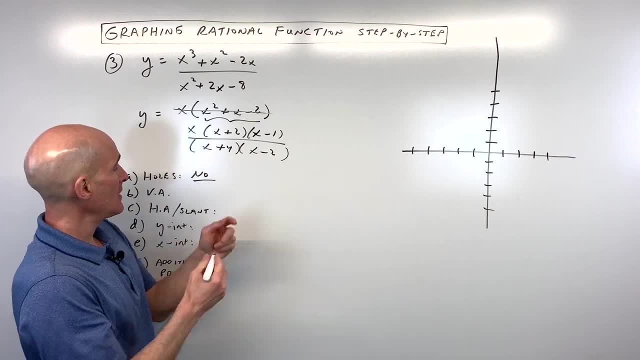 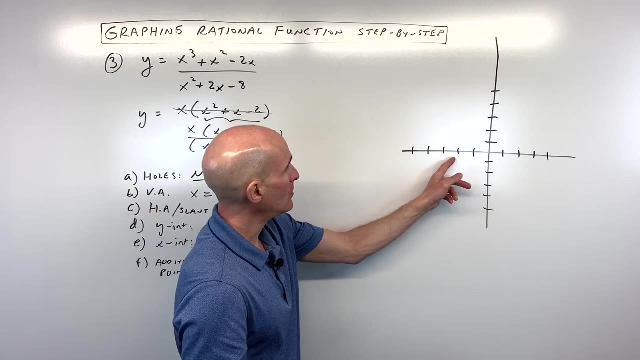 Remember we can't divide by 0. So by sending these factors to 0, we find our vertical asymptotes. So x equals negative 4 and x equals 2 are our vertical asymptotes. Let's draw those in. So this is: x equals negative 4 and x equals positive 2.. 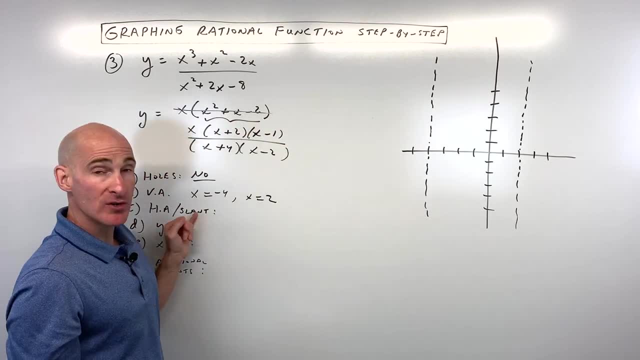 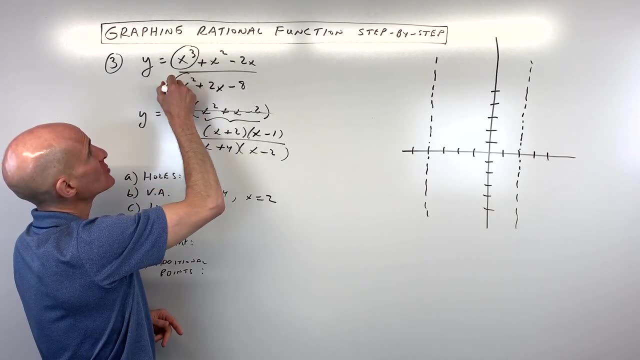 Looks like that. Now we want to analyze the horizontal asymptote or the slant asymptote, And how can we tell? Well, I'd like to go back to the original equation. And you want to zero in on those highest degree terms in the numerator and the highest degree term in the denominator. 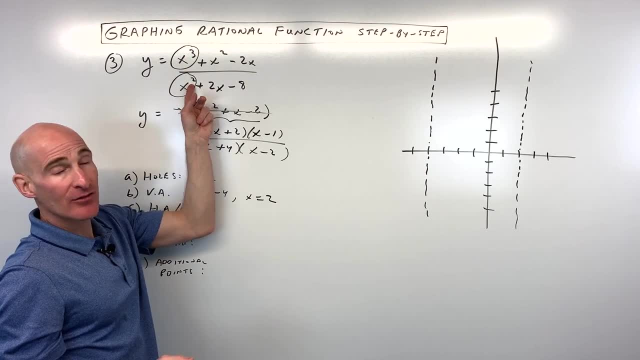 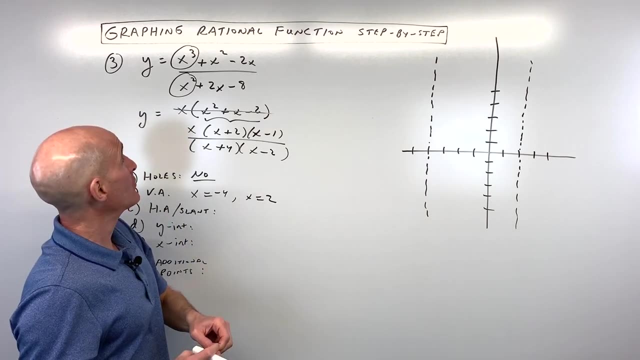 When the degree in the numerator is one degree higher than the degree in the denominator. that tells us that there's going to be a slant asymptote. Now you're probably saying, Mario, how do I find the equation of the slant asymptote? 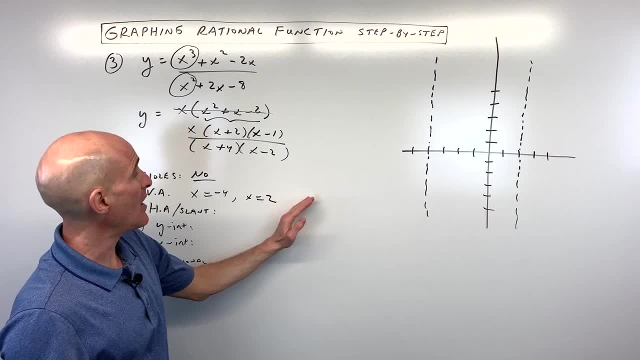 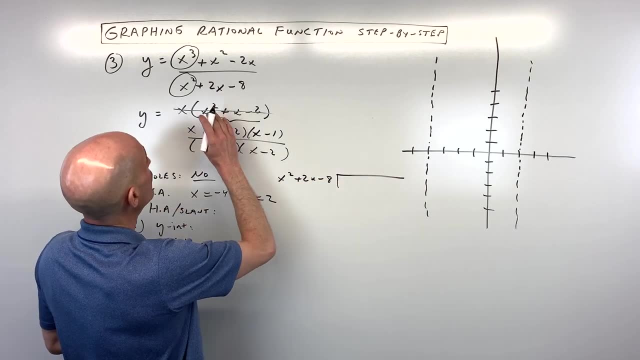 And you would do that by doing long division, polynomial long division. So let's go ahead and do that. So we're trying to see how many times does x squared plus 2x minus 8 go into x cubed plus x squared minus 2x? 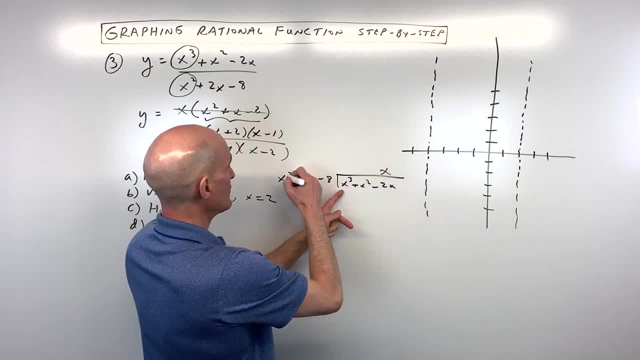 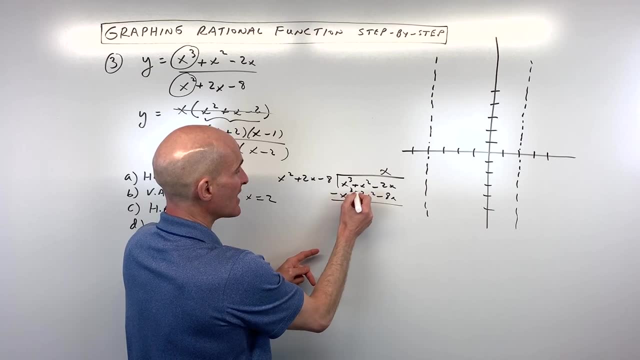 So x squared goes into x cubed x times. If we distribute, we get x cubed plus 2x squared minus 8x. We subtract, or you can change the signs to the opposite and add, Because subtraction is like adding the opposite. 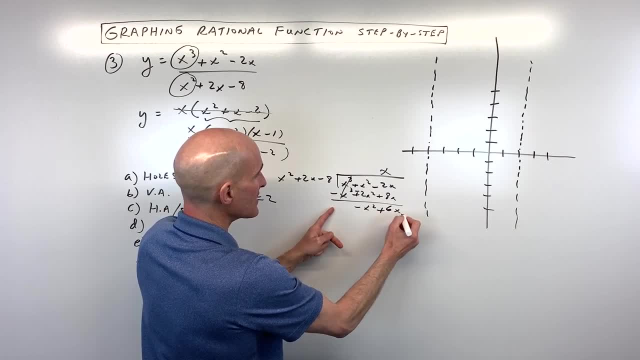 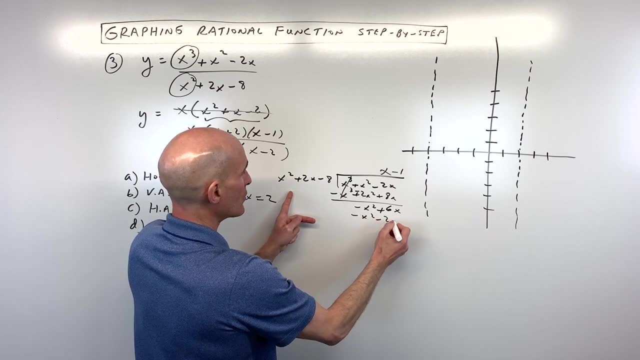 And this comes out to is that 6x? And then let's see how many times does x squared go into negative x squared? That's negative 1 times. If we distribute, we get negative x squared minus 2x plus 8.. 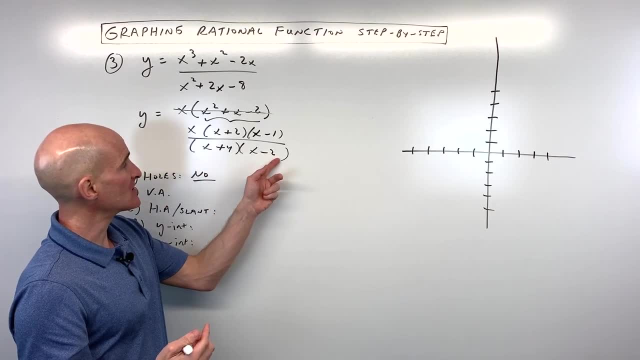 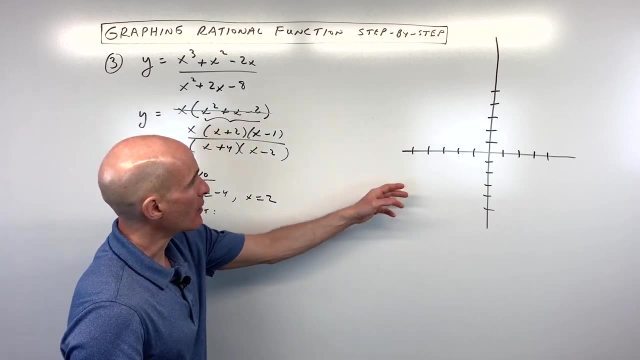 denominators. Remember we can't divide by zero. So by sending these factors to zero we find our vertical asymptotes. So x equals negative. 4 and x equals 2 are our vertical asymptotes. Let's draw those in, So this is: x equals negative. 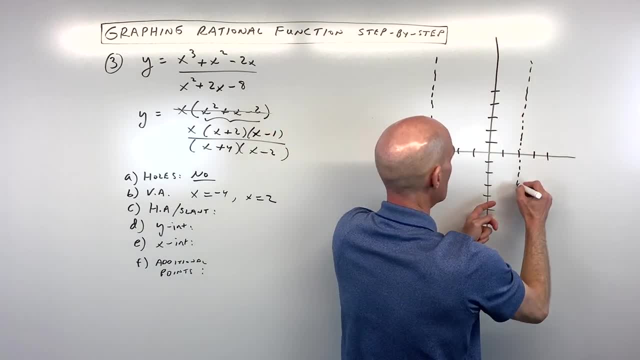 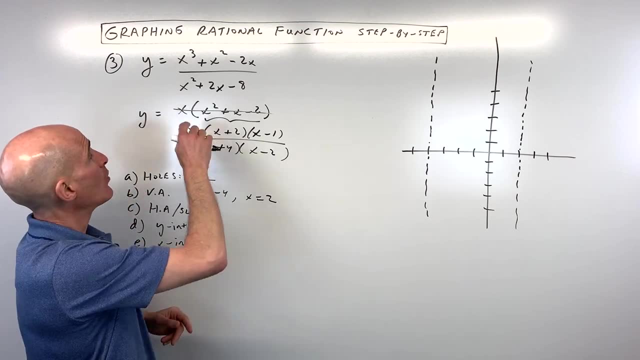 4 and x equals positive 2.. Looks like that. Now we want to analyze the horizontal asymptote or the slant asymptote, And how can we tell? Well, I'd like to go back to the original equation. and you want to zero in on those highest degree terms in the numerator and 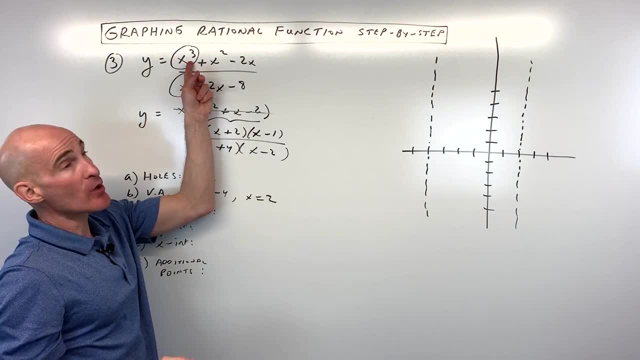 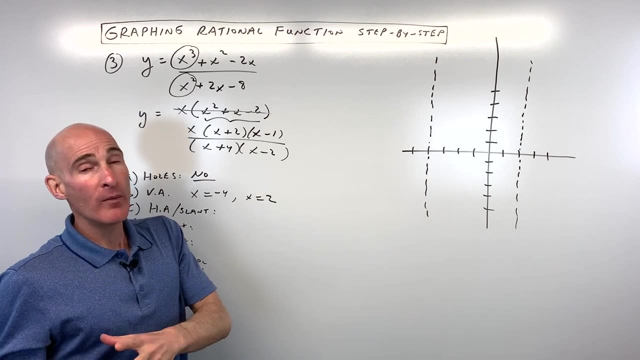 the highest degree term in the denominator. When the degree in the numerator is one degree higher than the degree in the denominator, that tells us there's going to be a slant asymptote. Now you're probably saying, Mario, how do I find the equation of the slant asymptote? And you would do. 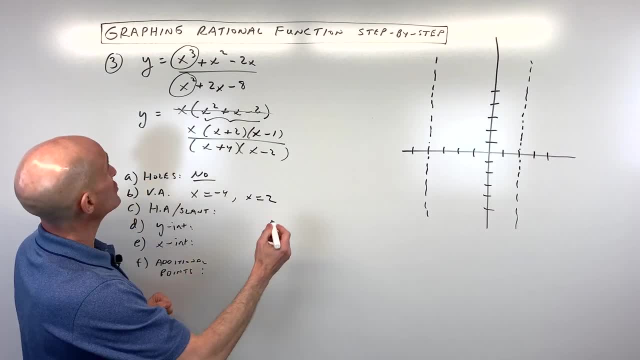 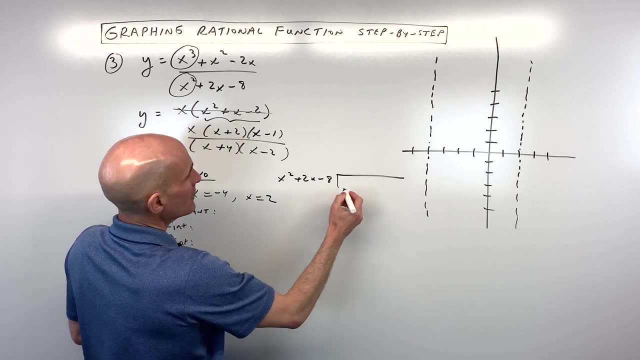 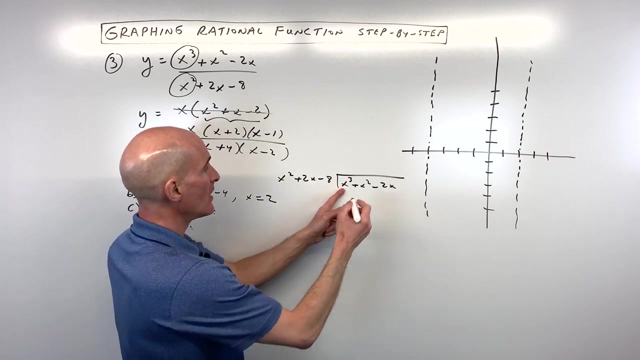 that by doing long division, polynomial long division. So let's go ahead and do that. So we're trying to see how many times does x squared plus 2x minus 8 go into x cubed plus x squared minus 2x. So x squared goes into x cubed x times. If we distribute we get x cubed plus 2x squared. 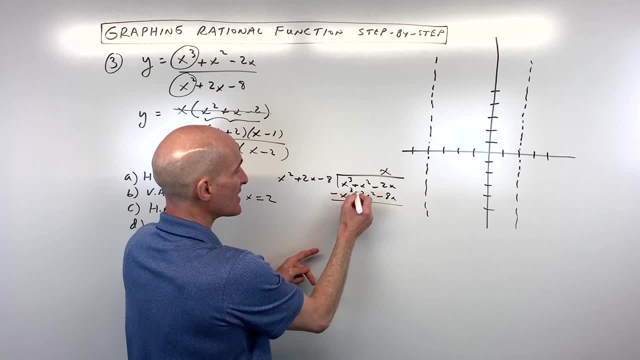 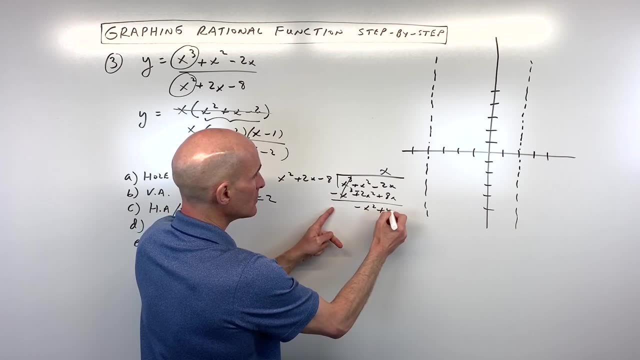 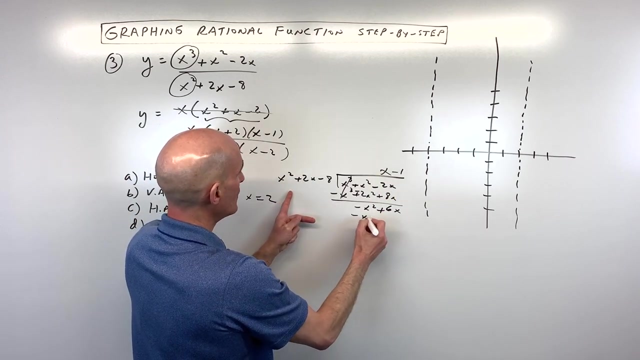 minus 8x, We subtract. or you can change the signs to the opposite and add, because subtraction is like adding the opposite And this comes out to is that 6x. And then let's see: how many times does x squared go into negative? x squared, That's negative 1 times. If we distribute, we get negative. 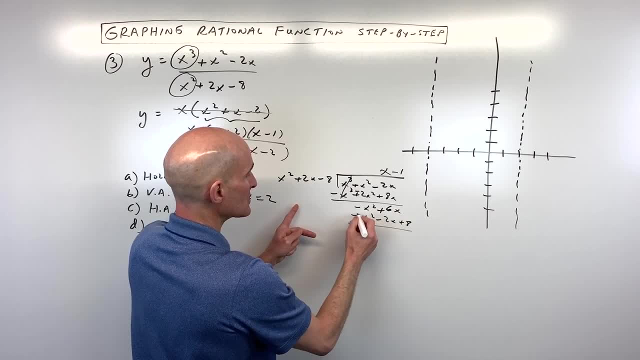 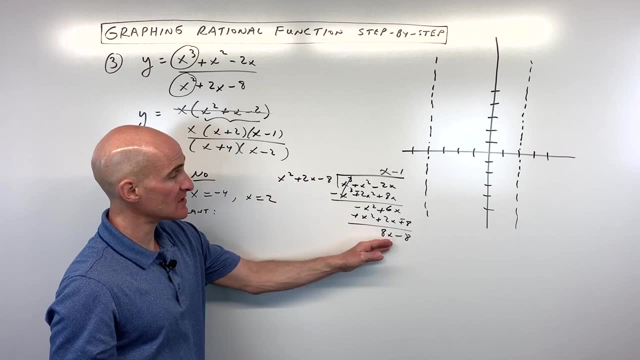 x squared minus 2x plus 8.. And if we subtract or change the signs to the opposite, we get 8x minus 8.. Now notice, this degree is lower than this degree. This is our remainder. You don't have to. 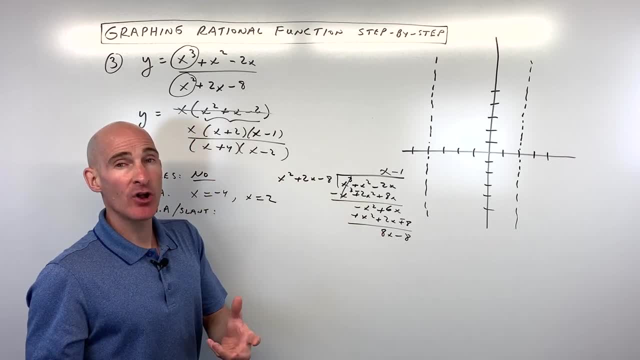 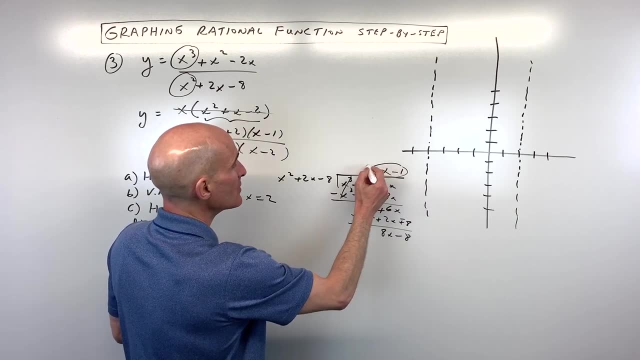 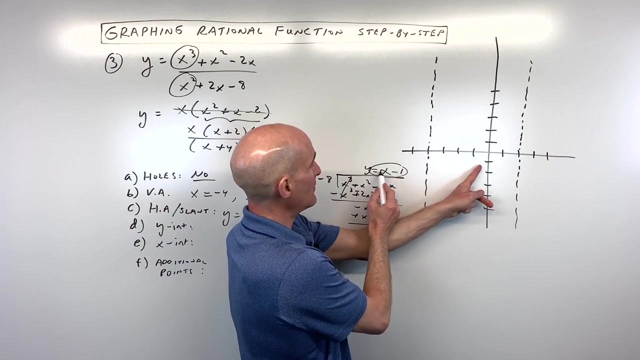 worry about the remainder. If you need help with the long division, check out my video on doing polynomial long division And I'll go over that in that video. But you can see this is really going to be: y equals x minus 1 is our slant asymptote. So the y intercept is going to be negative 1 and the slope is 1.. So 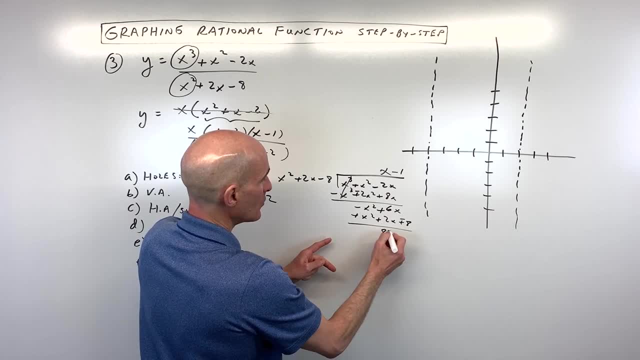 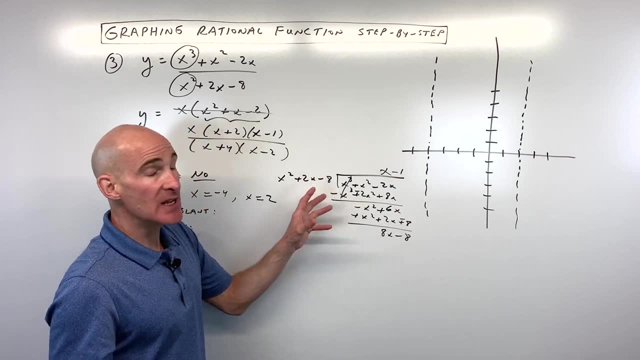 And if we subtract or change the signs to the opposite, we get 8x minus 8.. Now notice: this degree is lower than this degree. This is our remainder. You don't have to worry about the remainder. If you need help with the long division, check out my video on. 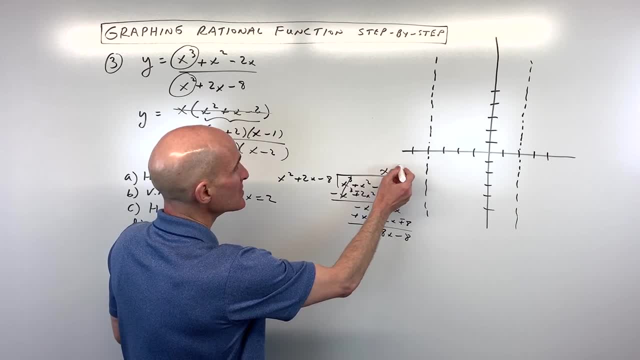 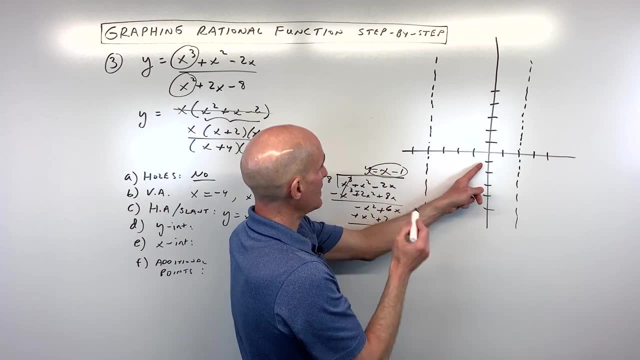 doing polynomial long division And I'll go over that in that video. But you can see this is really going to be: y equals x minus 1 is our slant asymptote. So the y-intercept is going to be negative 1.. 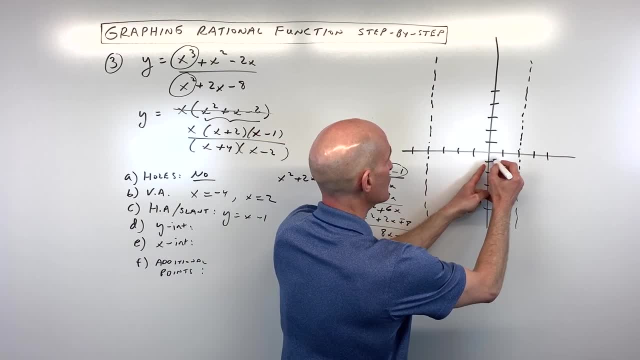 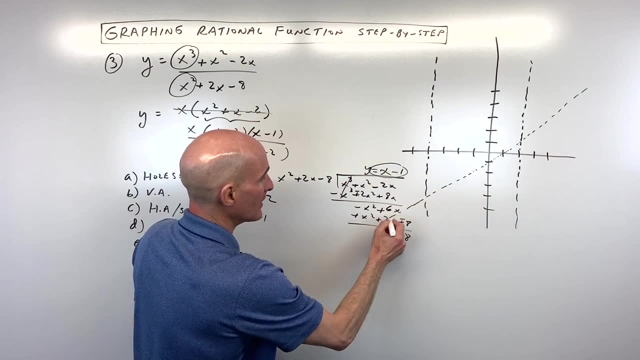 And the slope is 1.. So what? this is going to be starting here, it's going to be going up 1 over 1.. So it looks something like that: Okay, Okay, and I'm just going to erase this so it doesn't get in the way of our graph as we proceed. 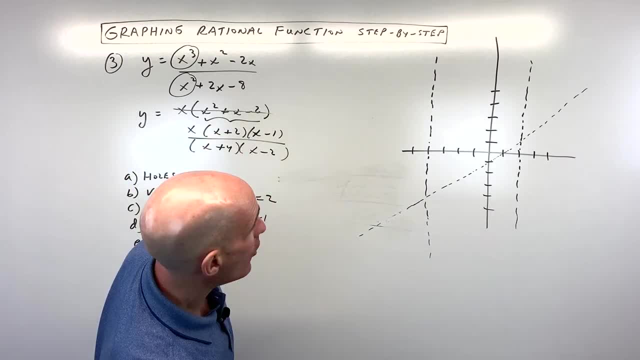 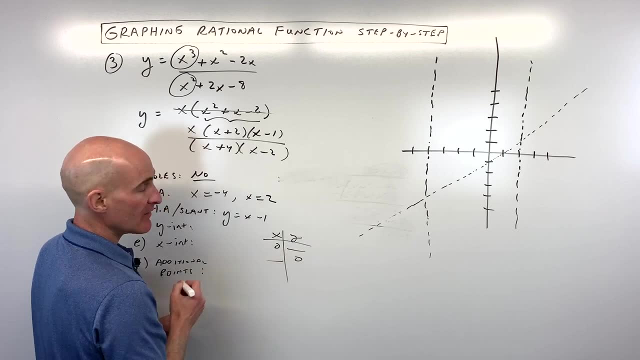 Okay, Okay. so now what we want to do is look at the x-intercept and the y-intercept And remember we do that by making a table and setting x to 0 and then setting y to 0. So by setting x to 0, it's going to cancel out all these terms except for this one. 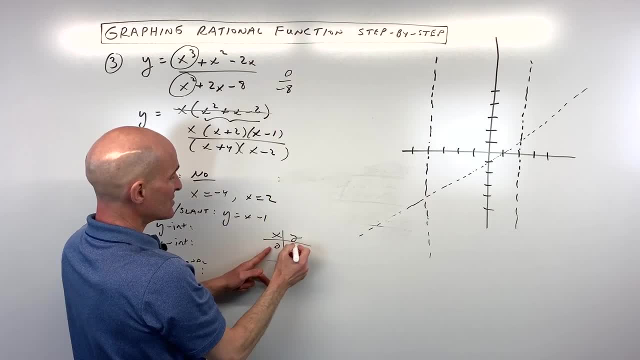 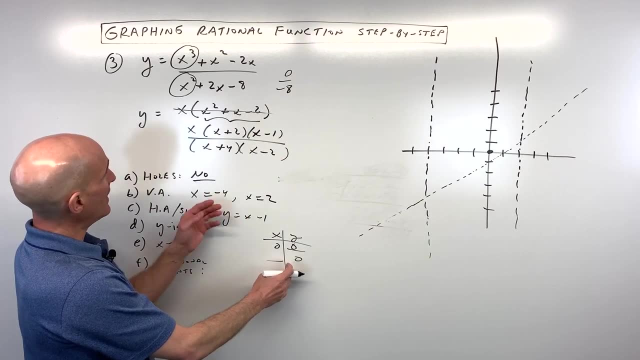 So it's going to be 0 over negative 8, which is just 0.. So it's going right here through the origin at 0, 0.. And if we set y to 0, okay, remember, the only way that y is going to be 0 is if the 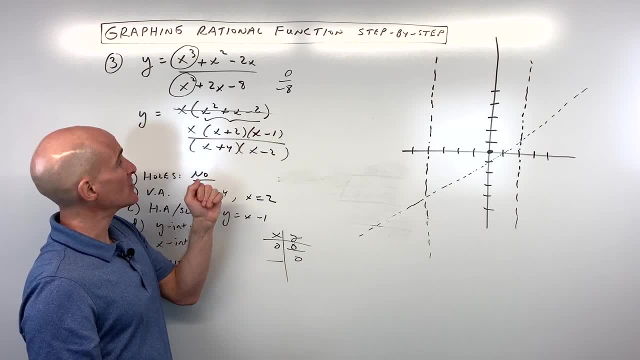 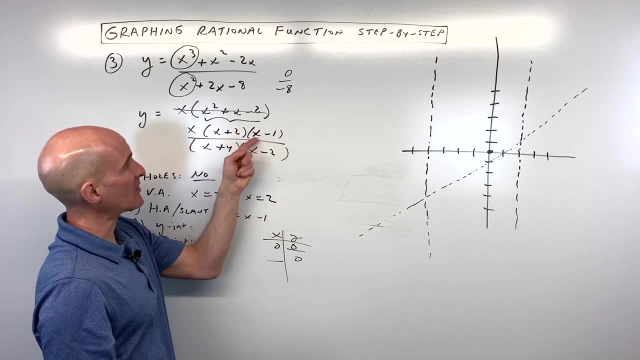 factors in the numerator are 0, because 0 divided by anything that's not 0 is 0.. We've already taken this one to account, 0, but it could also be negative 2 and positive 1.. I'm just setting these factors in the numerator to 0. 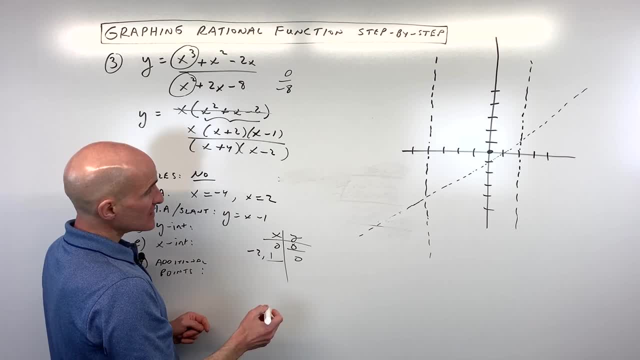 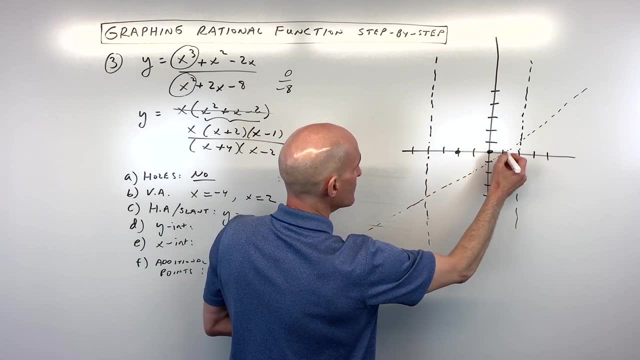 So I'm just going to write negative 2 or 1.. So let's see, it's going to cross right here at negative 2 and here at positive 1.. Okay, this is a pretty challenging graph. So now what we want to do is we want to plot some additional points. 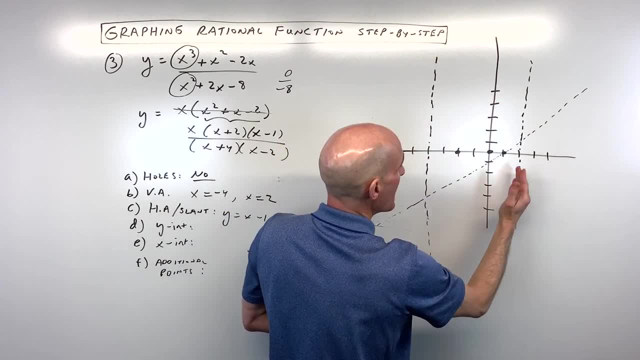 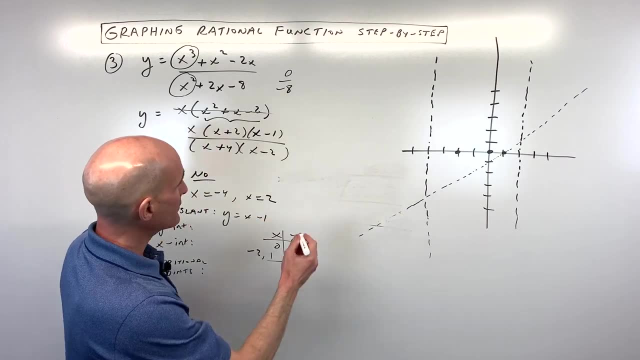 And what I usually do is pick points on either side. So I'm going to pick the side of the vertical asymptotes, because we want to see if the graph is going up towards positive infinity or down towards negative infinity. So let's start over here at negative 5.. 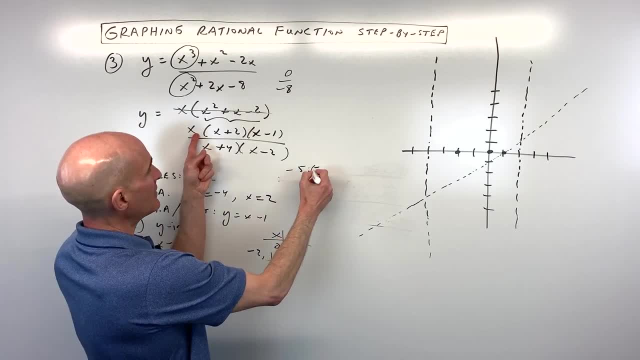 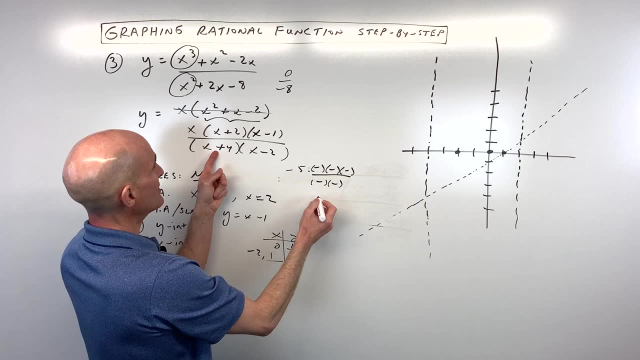 So let's see so negative 5, if I put negative 5 in here, I get a negative times a negative, times a negative all over. negative times a negative. So that comes out to 3 negatives is a negative, 2 negatives is a positive, a negative divided. 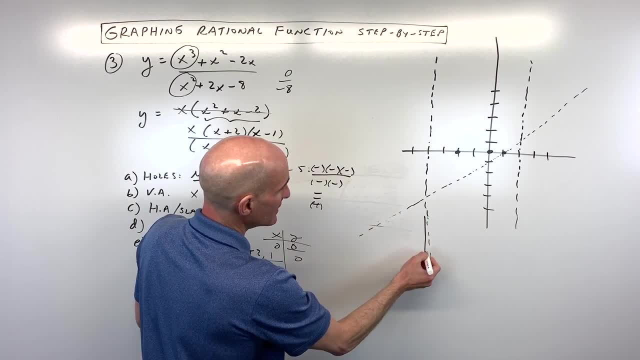 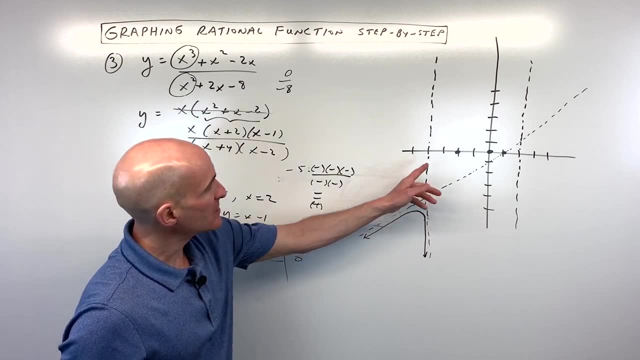 by a positive is a negative. So that tells us it's going down towards negative infinity. So you can see this graph is looking something like that. It's approaching the slant asymptote. Okay, now let's approach this vertical asymptote from this side. 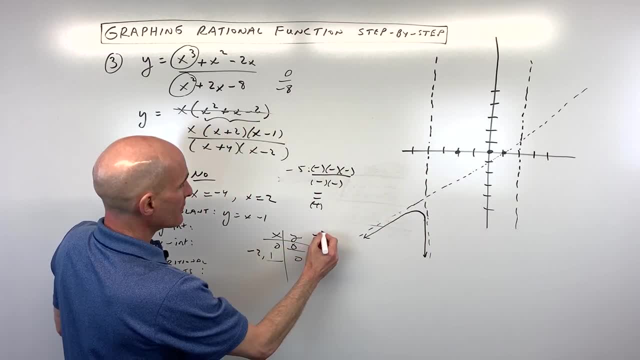 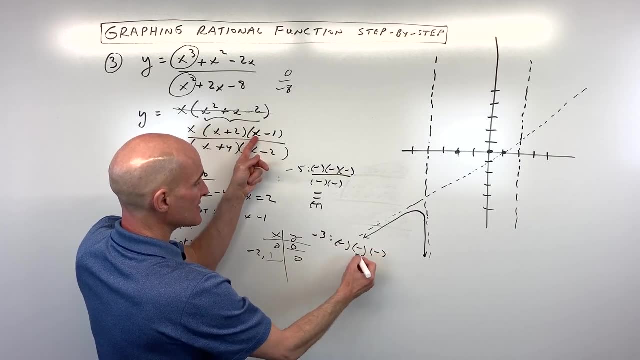 So let's maybe put in negative 3.. If we put in negative 3, we get a negative, Negative 3 plus 2 is negative, 1, that's negative. Negative 3 minus 1 is negative, 4, that's negative. 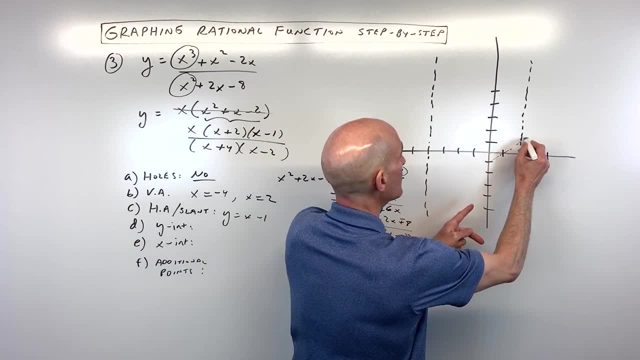 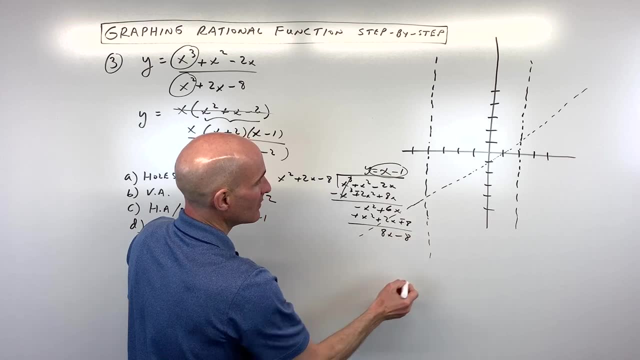 what this is going to be starting here. it's going to be going up 1 over 1.. So it looks something like that: Okay, Okay, and I'm just going to erase this so it doesn't get in the way of our, of our graph. 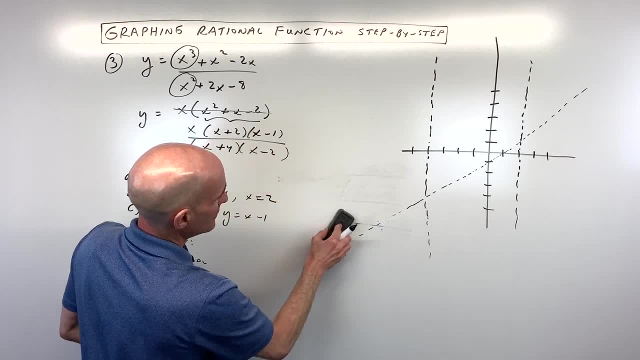 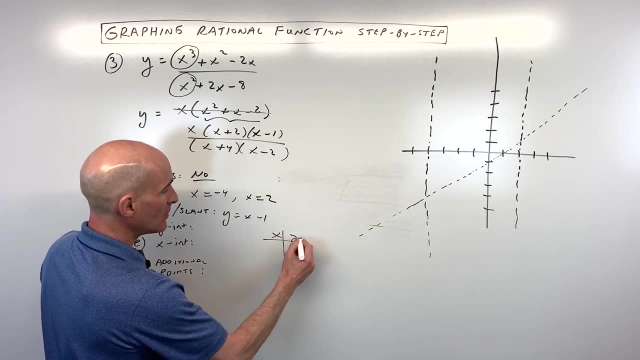 as we proceed. Okay, Okay. so now what we want to do is look at the x-intercept and the y-intercept. Remember, we do that by making a table and setting x to 0 and then setting y to 0. So by setting x to 0, it's. 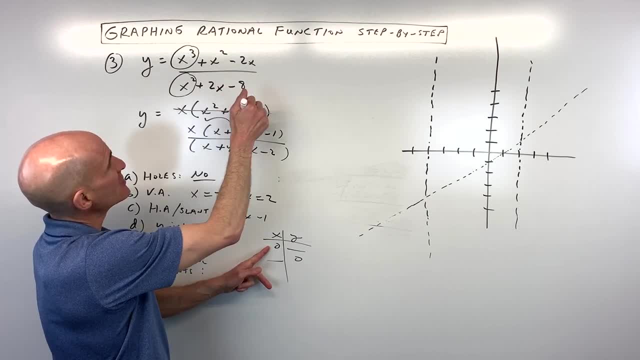 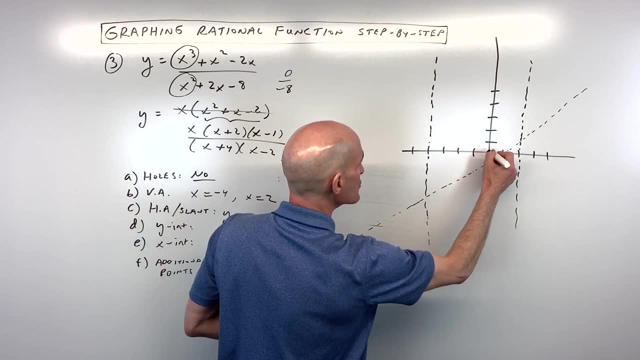 going to cancel out all these terms except for this one. So it's going to be 0 over negative 8, which is just 0. So it's going right here through the origin at 0, 0.. And if we set a y to 0,, 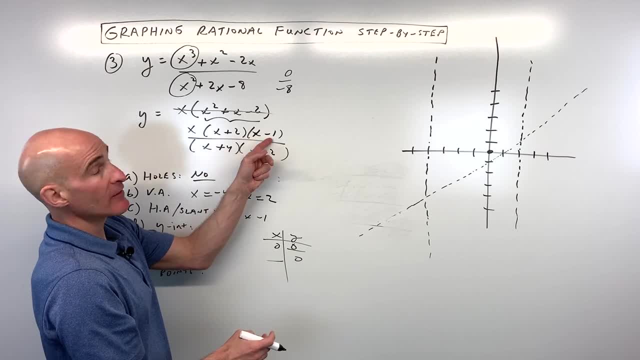 okay, remember, the only way that y is going to be 0 is if the factors in the numerator are 0. Because 0 divided by anything that's not 0 is 0. We've already taken this one to account: 0,. 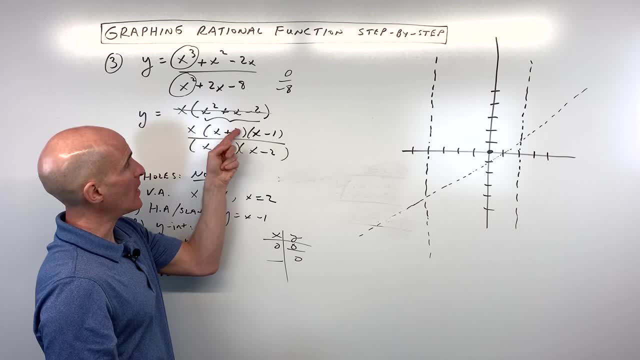 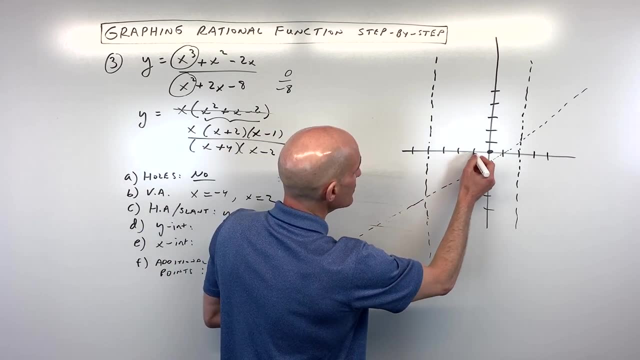 but it could also be negative 2 and positive 1.. I'm just setting these factors in the numerator to 0., So I'm just going to write negative 2 or 1.. So let's see, It's going to cross right here. 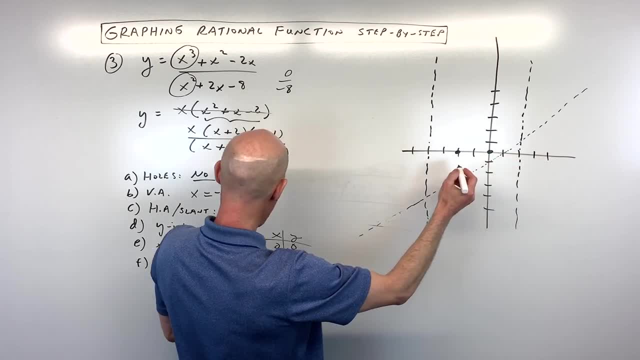 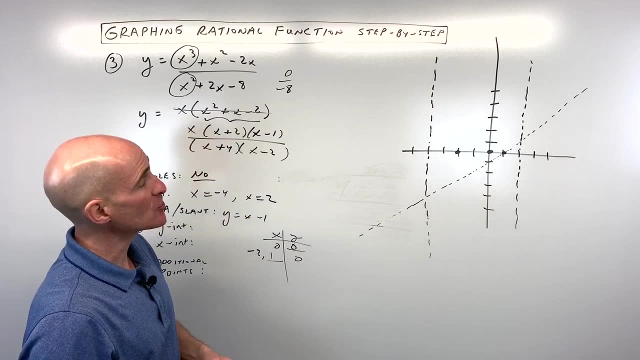 at negative 2 and here at positive 1.. Okay, this is a pretty challenging graph. So now what we want to do is we want to plot some additional points, and what I usually do is pick points on either side of the vertical asymptote. 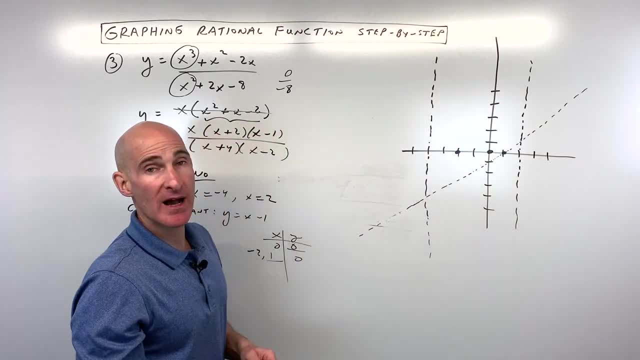 Okay. So you might ask: what are these two points? So I assume the proprietary reporting point is two, Because we want to see if the graph is going up towards positive infinity or down towards negative infinity. So let's start over here at negative 5.. 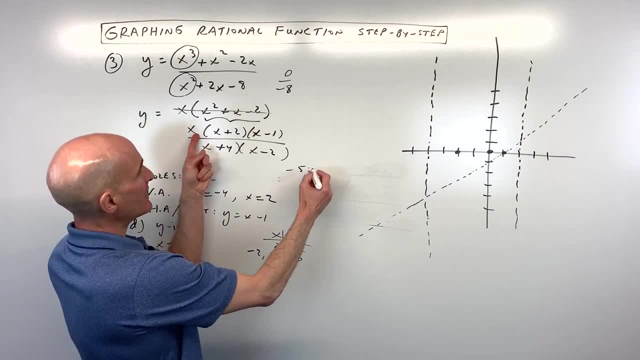 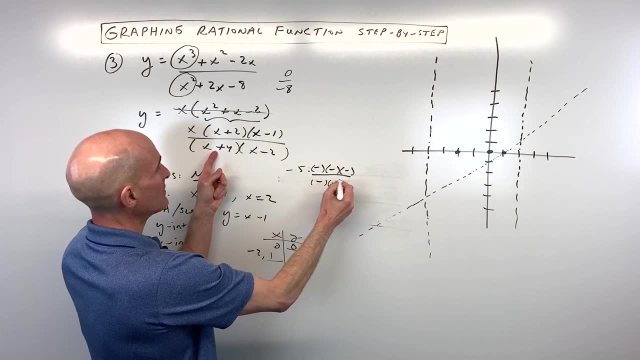 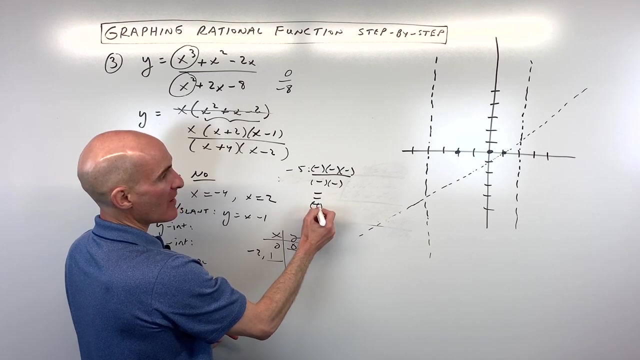 So let's see so negative 5, if I put negative 5 in here, I get a negative times a negative times a negative all over negative times a negative. So that comes out to 3 negatives is a negative, 2 negatives is a positive. a negative divided by a positive is a negative. 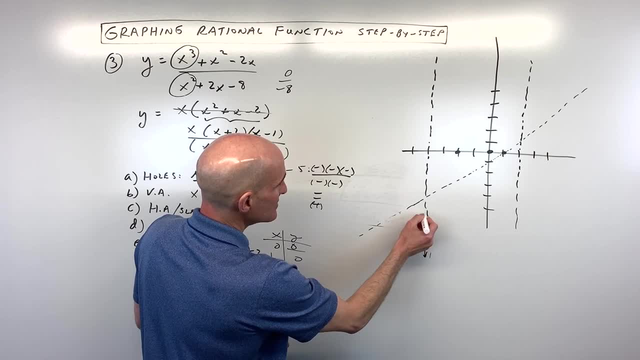 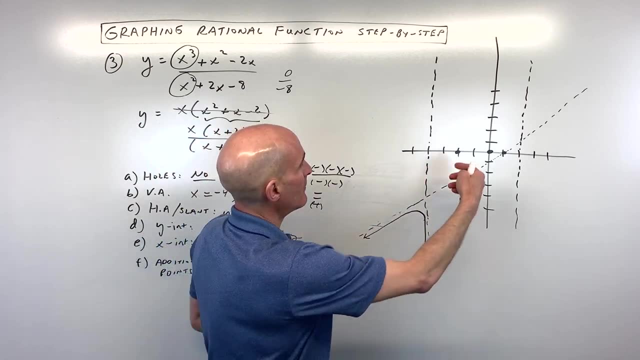 So that tells us it's going down towards negative infinity. So you can see, this graph is looking something like that: It's approaching the slant asymptote. Okay, now let's approach this vertical asymptote from this side. So let's maybe put in negative 3.. If we put in negative 3,, 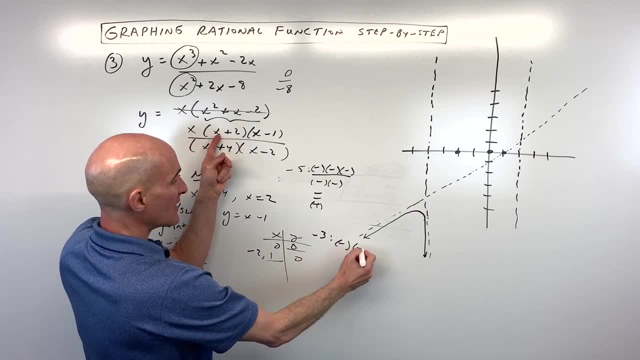 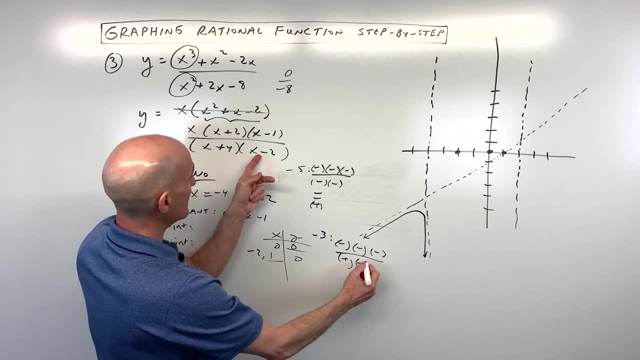 we get a negative. Negative: 3 plus 2 is negative: 1, that's negative. Negative: 3 minus 1 is negative: 4, that's negative. Negative: 3 plus 4 is positive: 1, that's positive. Negative: 3 minus 2 is negative. 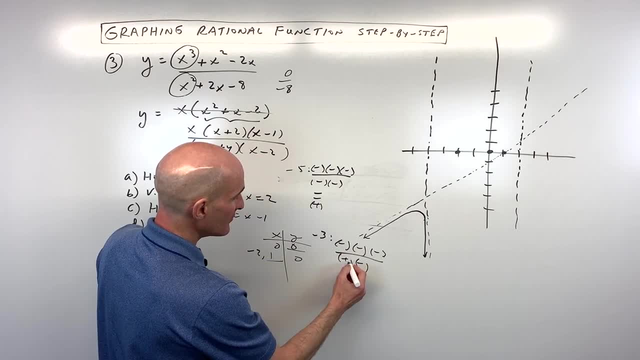 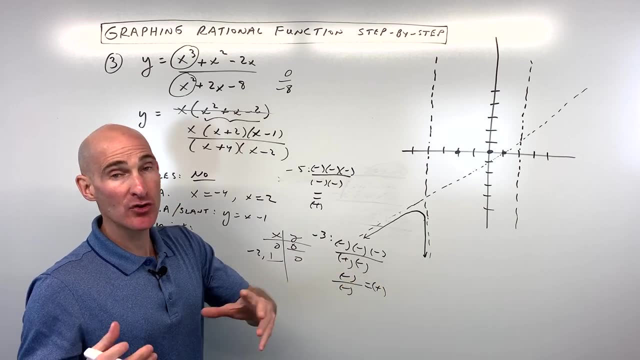 5, that's negative. So here we get 3 negatives multiplies to a negative. A positive times a negative is a negative, A negative over a negative is a positive. See how we're just analyzing the signs. It's not so important the number. I mean you could get the number and then plot that point precisely. 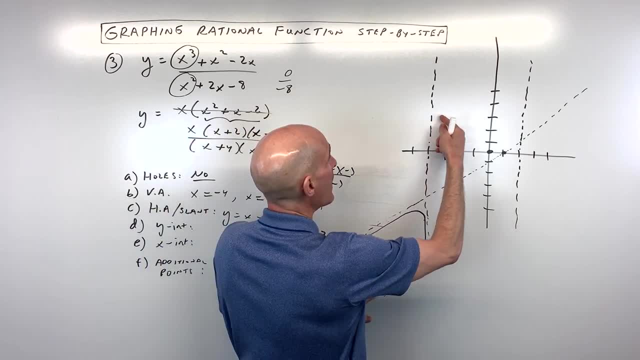 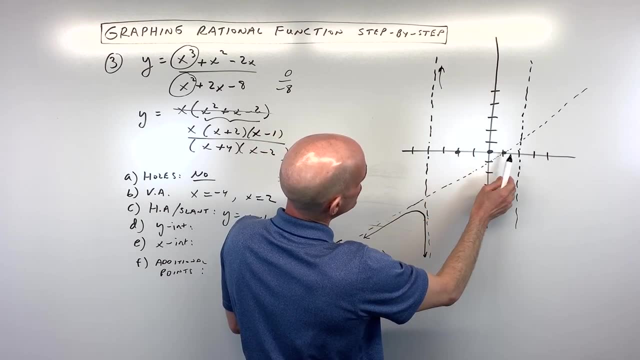 But the main thing is, I want to figure out: this is positive, It's going up towards positive infinity, So I'm just going to draw an arrow like that. And so now what happens here? Well, let's go now to this vertical asymptote. 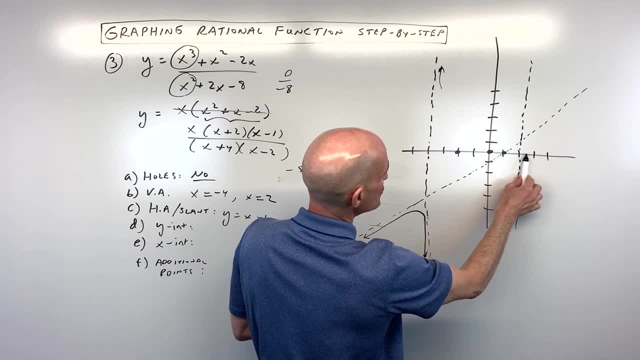 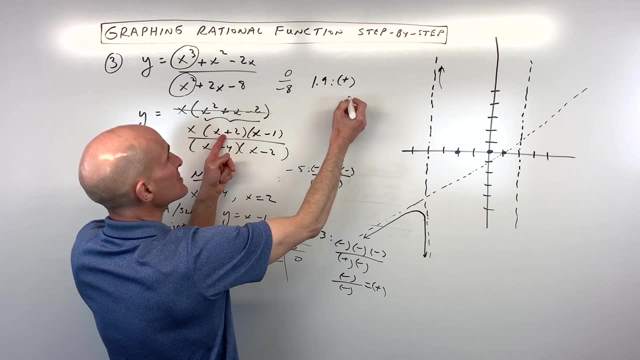 Let's pick 1.9 and 2.1.. So just on either side. So if I pick 1.9 here, that's going to be positive. right, This is going to be positive, This is going to be positive. 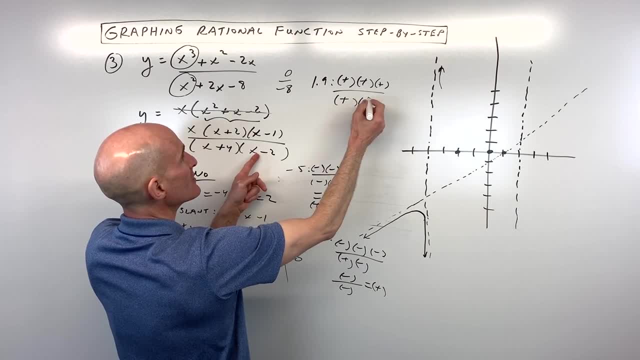 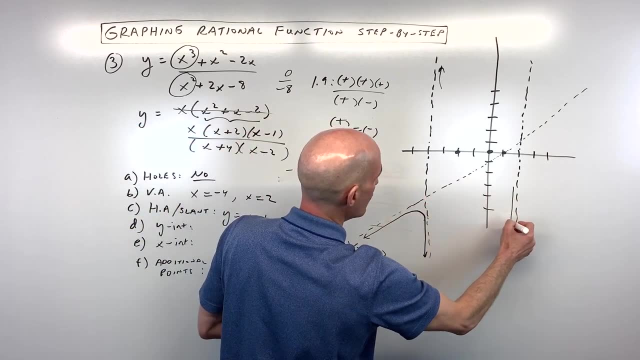 This is going to be positive, This is going to be negative. So we have a positive divided by a negative, which is a negative, which tells us that this is going down like this. Let's go from this side here, Let's pick, maybe what did I say? 2.1.. 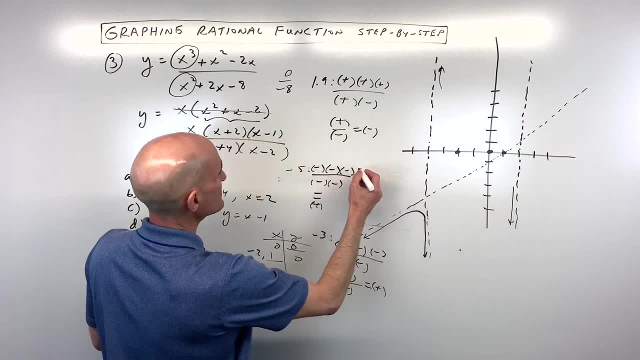 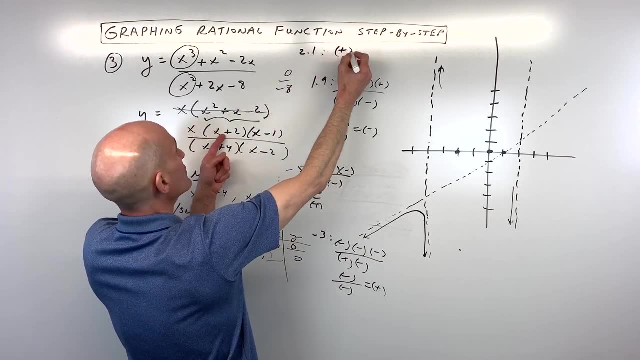 So let's see So for 2.1, see we need some space here. How about up here 2.1?? So 2.1, we get a positive. 2.1 plus 2 is positive. 2.1 minus 1 is positive. 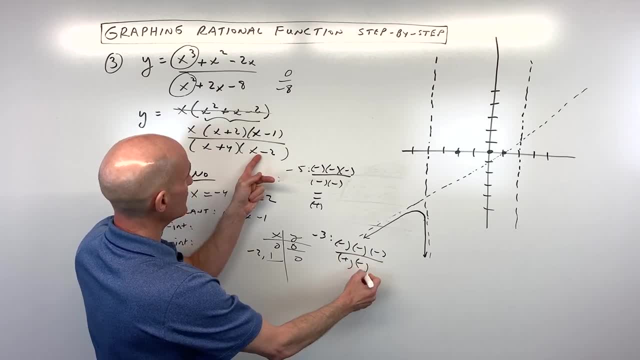 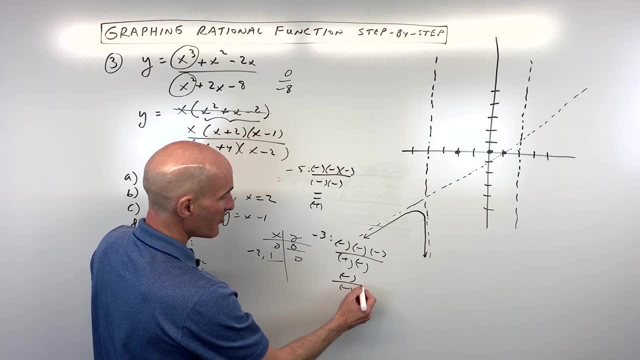 Negative: 3 plus 4 is positive. 1, that's positive. Negative: 3 minus 2 is negative. 5, that's negative. So here we get 3 negatives multiplied by 2 is negative. Positive times: a negative is a negative. a negative divided by a negative is a positive. 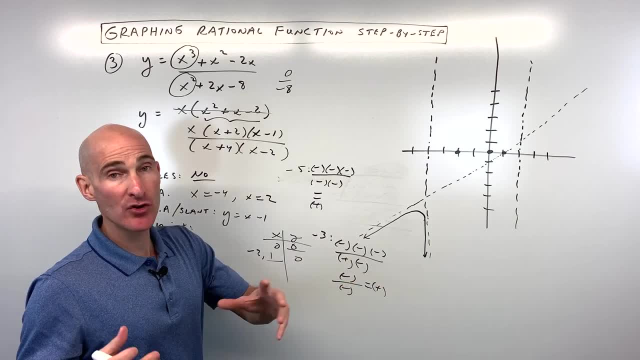 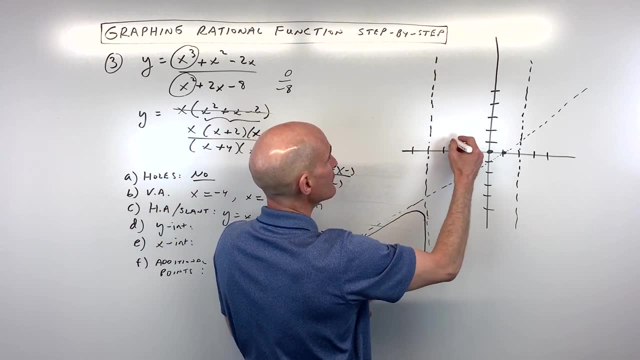 See how we're just analyzing the signs. It's not so important the number. I mean you could get the number and then plot that point precisely. but the main thing is I want to figure out: this is positive. it's going up towards positive infinity. 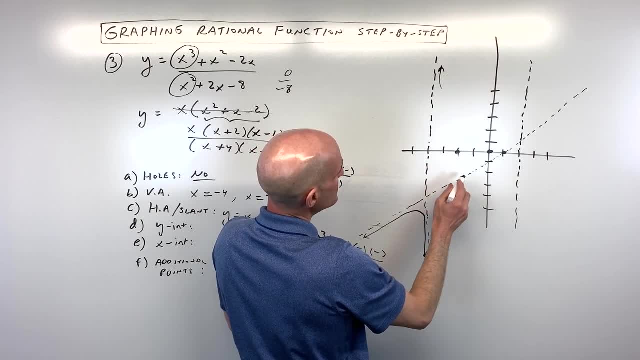 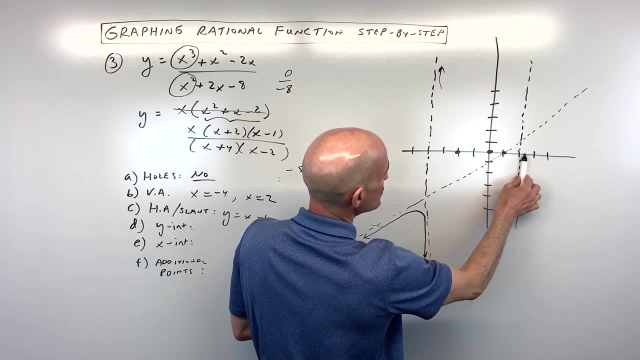 So I'm just going to draw an arrow like that. And so now what happens here? well, let's go now to this vertical asymptote. Let's pick 1.9 and 2.1, so just on either side. So if I pick 1.9 here, that's going to be positive. 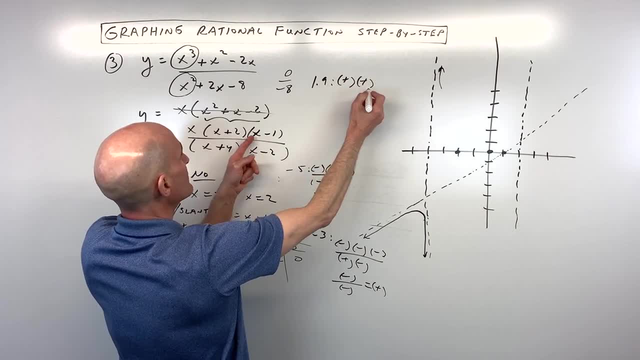 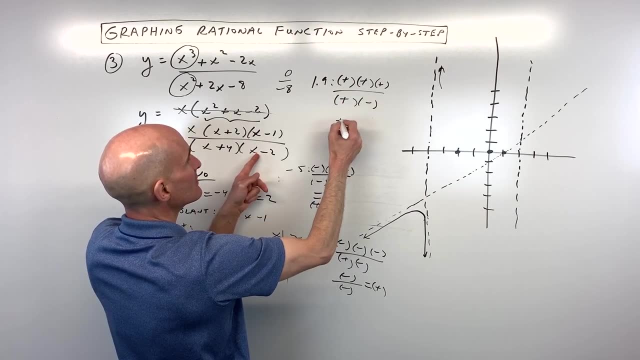 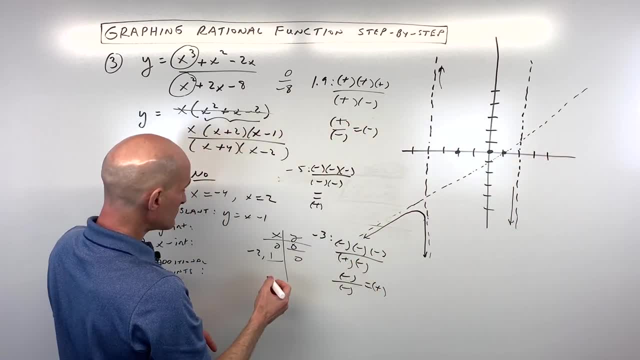 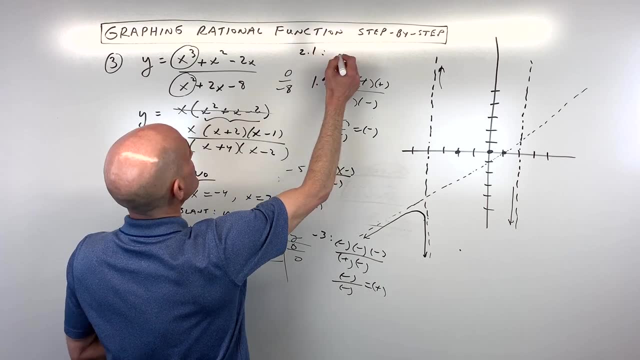 Let's go from this side here, Let's pick maybe what did I say? 2.1.. So let's see, So for 2.1, see, we need some space here. how about up here, 2.1.. 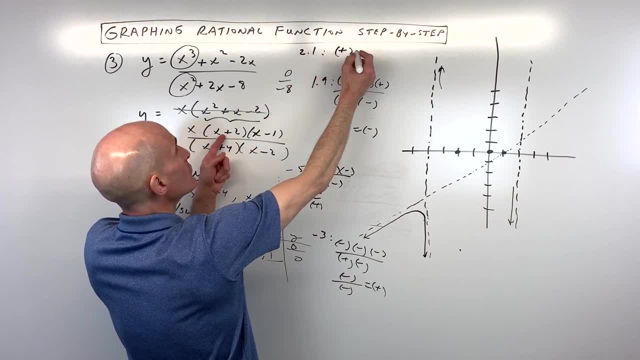 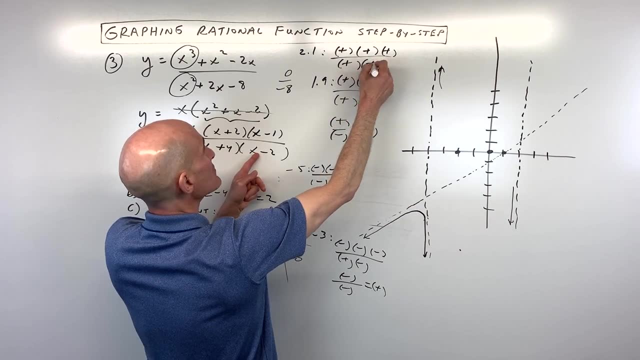 So 2.1, we get a positive. 2.1 plus 2 is positive, 2.1 minus 1 is positive. This is positive and this is positive. So you can see this is going to be positive over positive, which is positive, so that 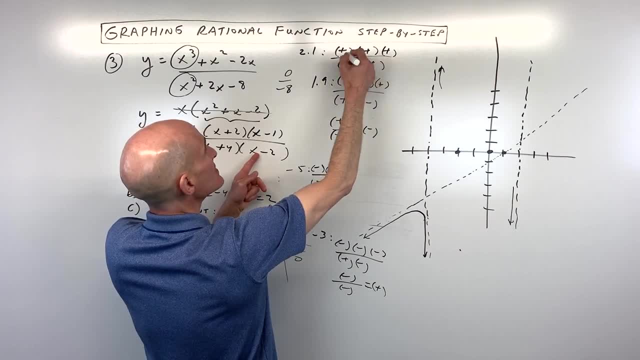 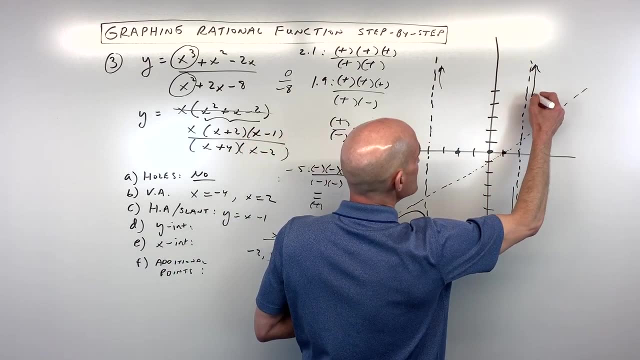 This is positive And this is positive. So you can see, this is going to be positive over positive, which is positive. So that means this is going up towards positive infinity right there. So this branch, you can see it's basically going something like this, approaching that slant asymptote. 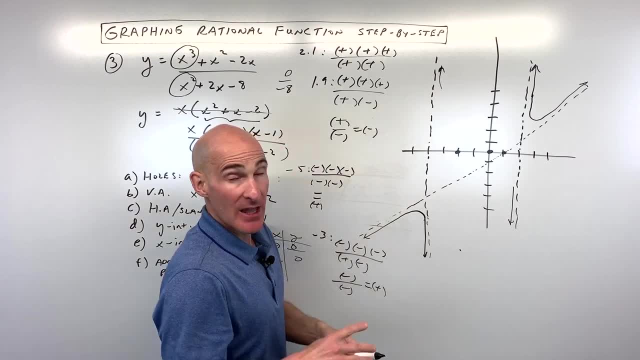 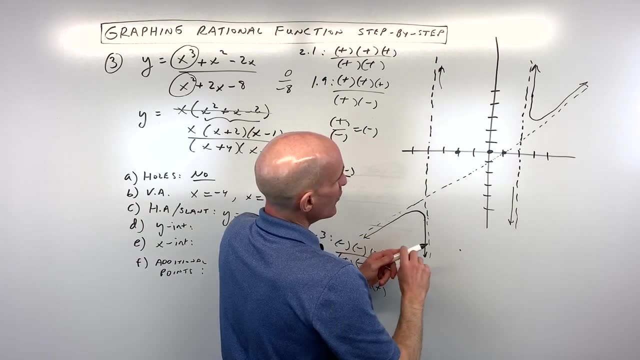 But what happens in here? Well, you can see that and you can plot some additional points here too, Like I might put in maybe like a half and maybe like negative one, But what you're going to see is this graph is actually going to go like this: 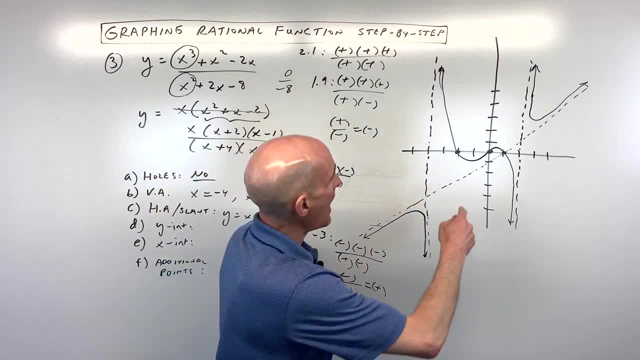 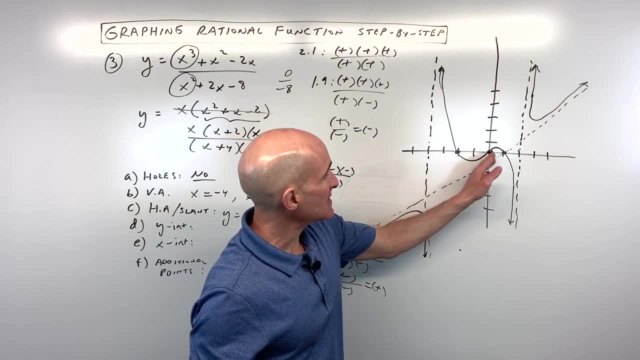 And you got it. Now some people will ask me say: well, how did you know to bend right there, Like, why don't you go way up here and then way down here and like that? Well, you can, like I said, plot some additional points when you get to calculus. 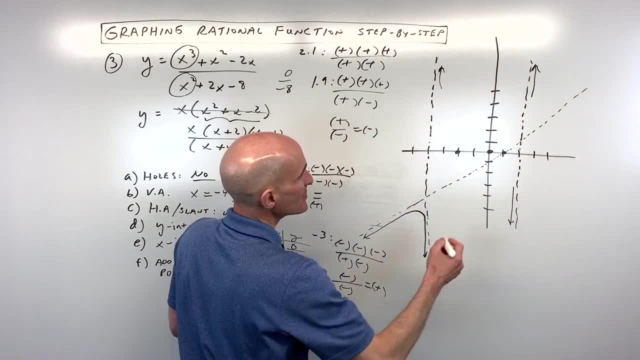 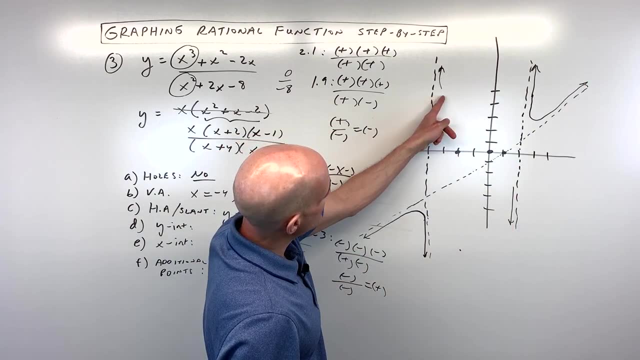 means this is going up towards positive infinity, right there. So this branch, you can see, it's basically going something like this, approaching that slant asymptote. But what happens in here? Well, you can see that and you can plot some additional points here too, like I might put. 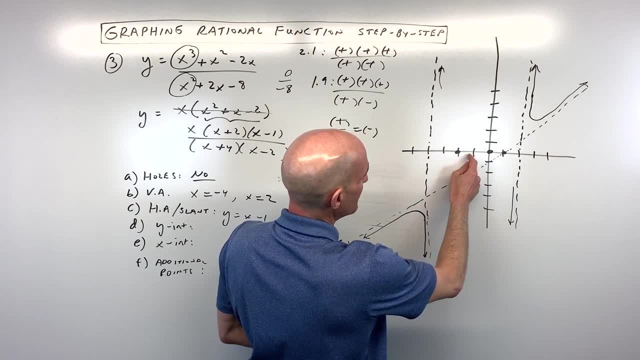 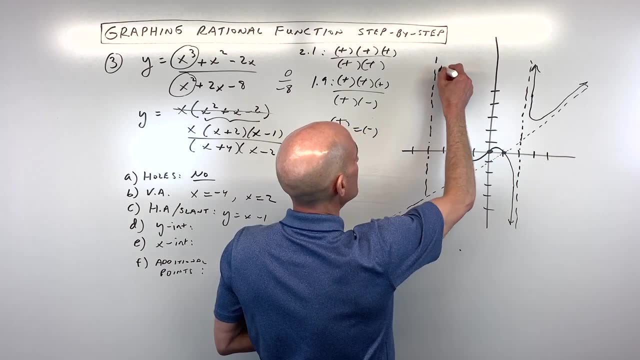 in, maybe like a half and maybe like negative 1.. But what you're going to see is this graph is actually going to go like this and you got it. Now some people will ask me say, well, how did you know to bend right there? 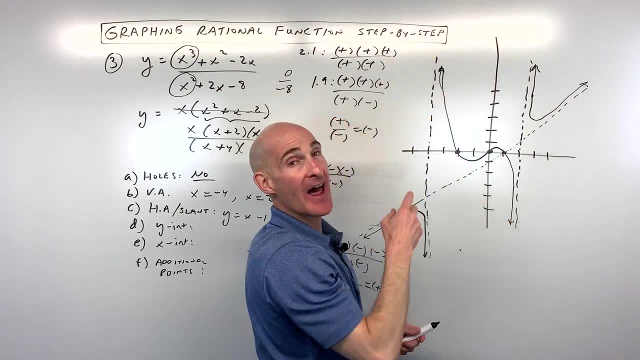 Like: why didn't you go way up here and then way down here and like that? Well, you can, like I said, plot some additional points. When you get to calculus, you're going to be able to find this exact point where the